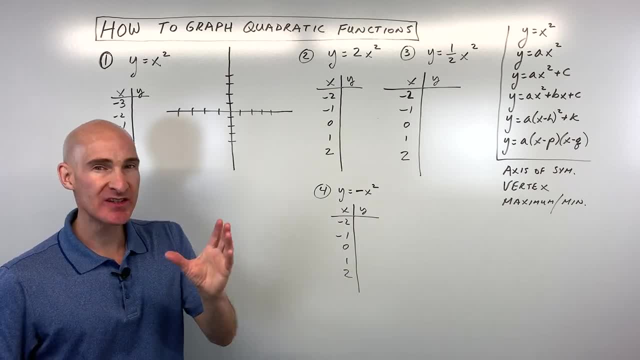 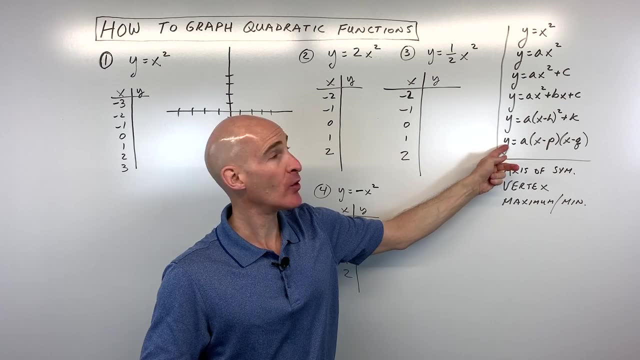 In this lesson you're going to learn how to graph quadratic equations. These are the parabola-shaped graphs, And what we're going to do is we're going to work through all these different forms of the quadratic equation here to graph these parabolas in these different 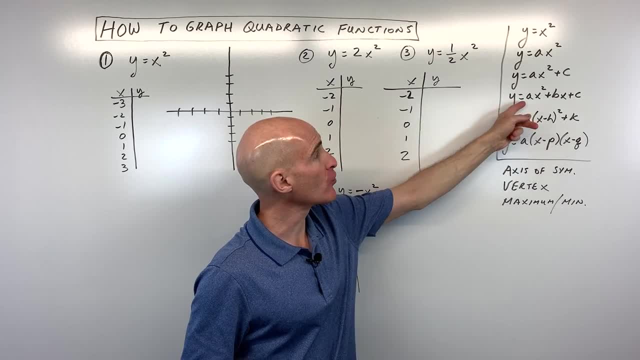 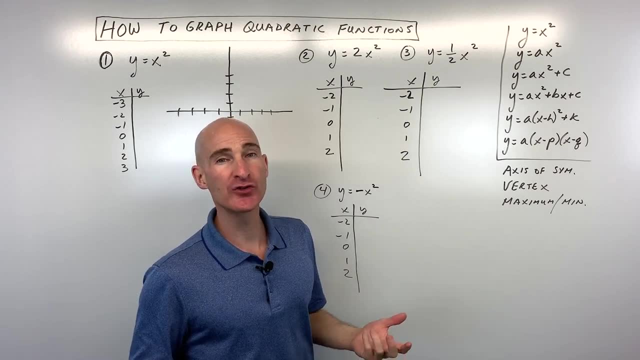 forms. So we've got the vertex form, the intercept form, the standard form and then some of the parent function graphs. We're also going to talk about transformations and we're going to talk about how to approach these graphs so you can easily get a good graph. So let's. 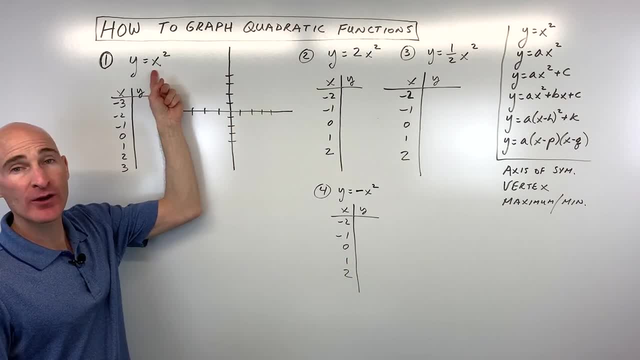 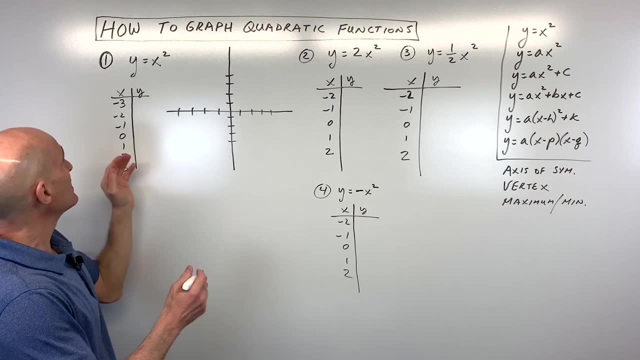 dive in. The first problem is just to basically look at the y equals x squared form of the equation, And this is what we call our parent function. What you can do is you can just pick some points. I usually pick a couple negative, zero and a couple positive, And 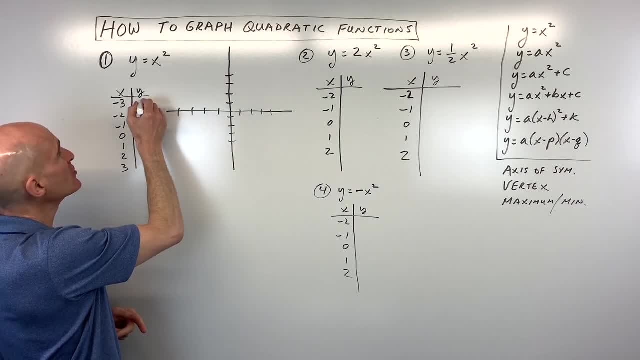 we're just going to put those in for x. So we've got negative three squared, which is nine. negative two squared, which is four. negative one squared, which is one. zero squared is zero. one squared is one times one, which is one. two squared is two times two, which. 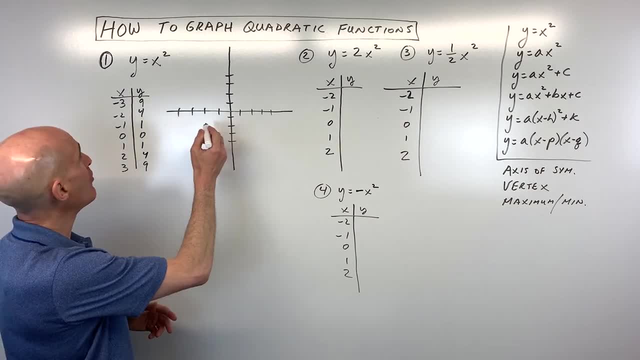 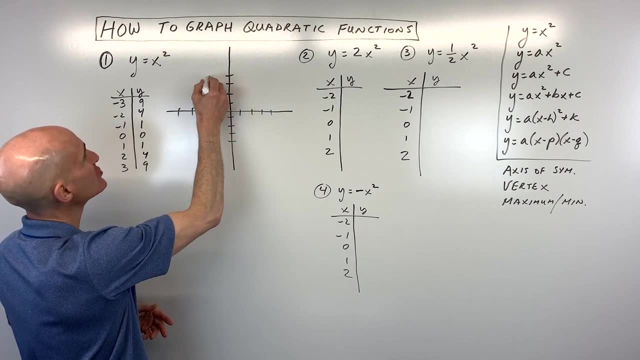 is four and three squared is nine. Now let's go ahead and plot these points. We've got negative three, nine, which is way up here, So I'm going to skip that one. Negative two: four, which is right here. Negative one: 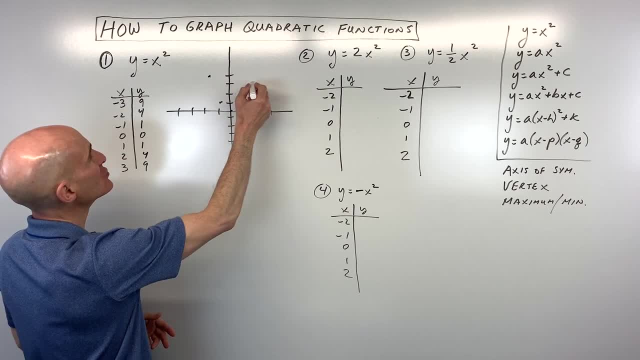 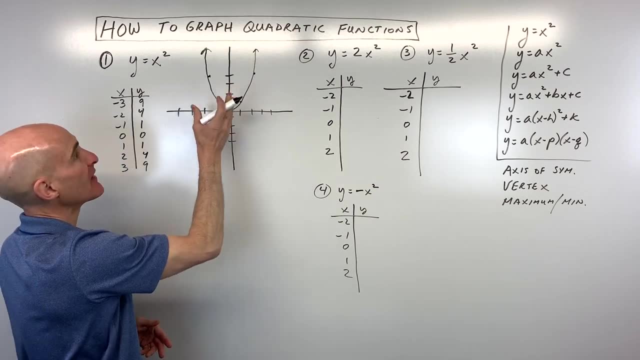 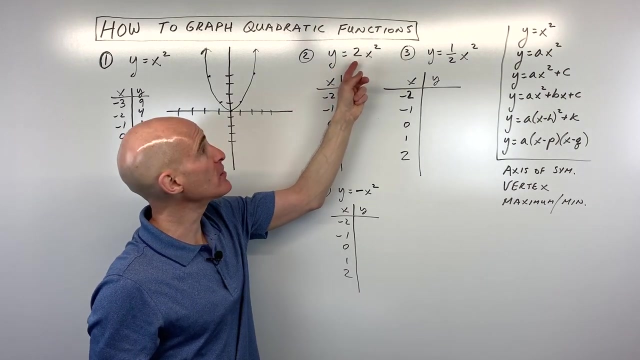 one which is here Zero, zero, one, one, two, four, three, nine. When you graph this, you get this nice u-shaped graph And that's what we call a parabola. Now what happens when you have like for number two? we have y equals two x squared. What do you think? 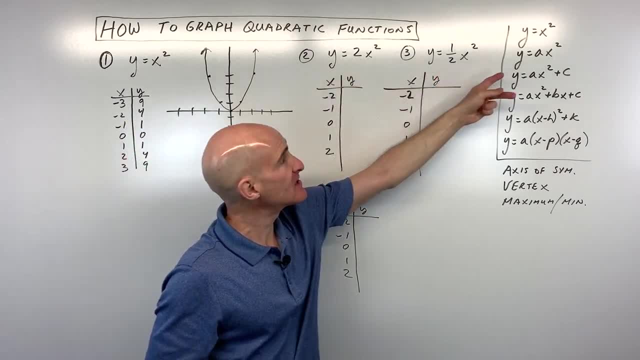 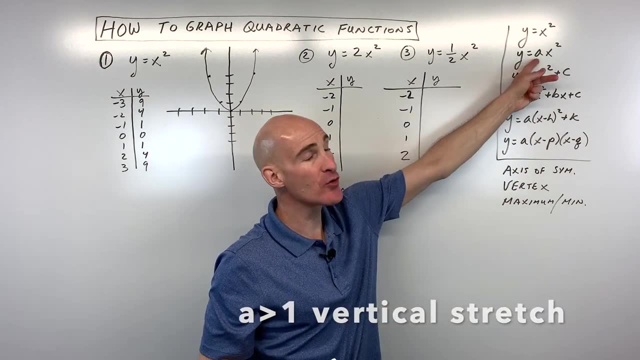 that two does Well. see this, this is the form we're working with now. The a value. if it's greater than one, it stretches the graph, And if it's between zero and one, it shrinks the graph. Okay, 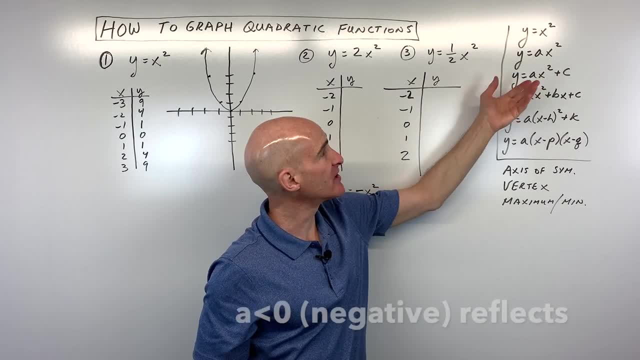 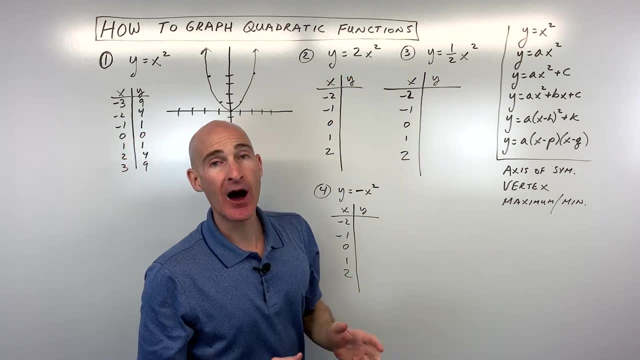 it's a vertical shrink like a compression, And if it's negative, what it does is it reflects it over the x-axis. it's going to make it open down, Okay, and we're going to look at all those different types now. So let's go ahead and look at: y equals two x squared. 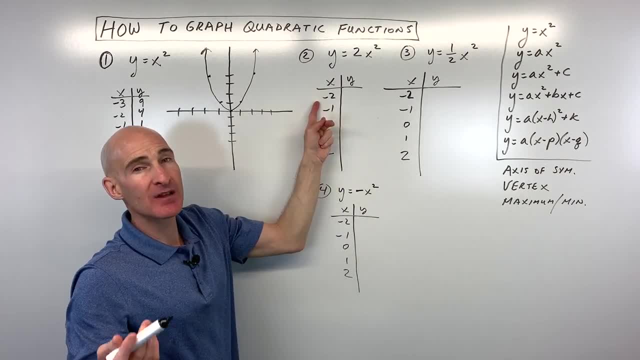 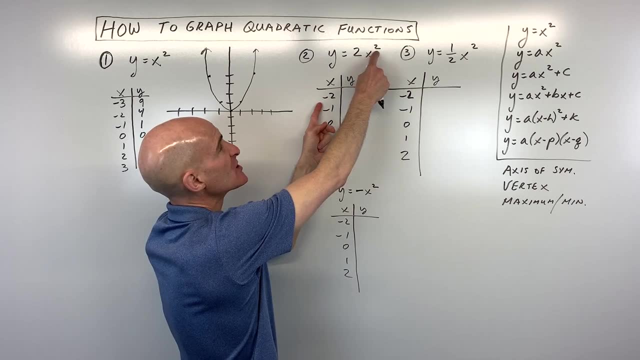 Again, you can make a table. Sometimes what students make a mistake is they're going to think about working from left to right. You want to think of doing the order of operations, the PEMDAS. So if we put negative two in here and we square it, negative two squared is 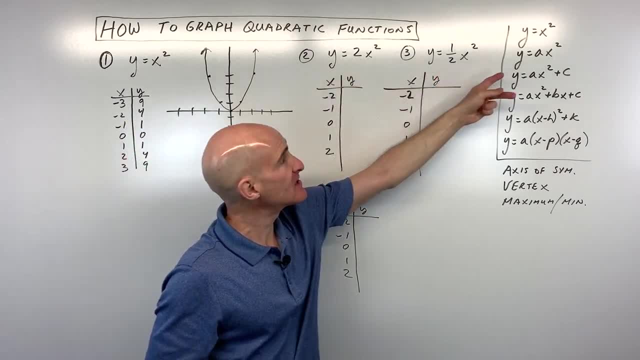 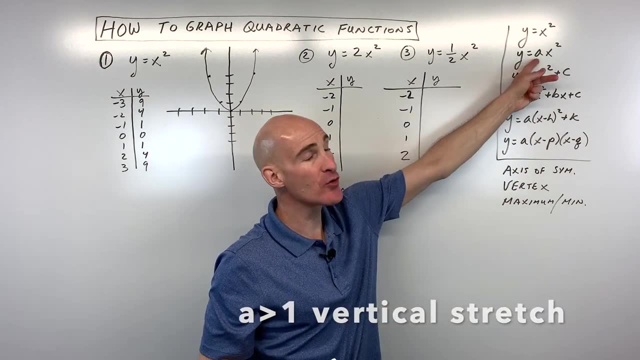 that two does Well. see this, this is the form we're working with now. The a value. if it's greater than one, it stretches the graph, And if it's between zero and one, it shrinks the graph. Okay, 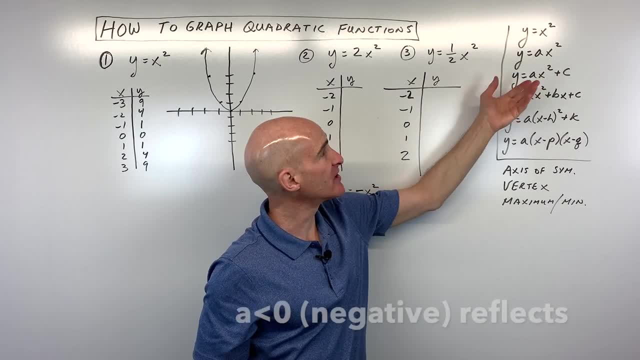 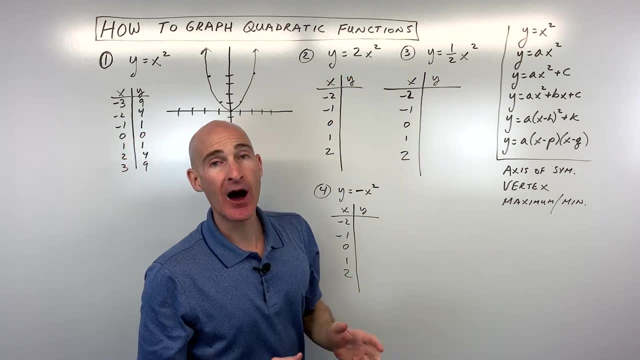 it's a vertical shrink like a compression, And if it's negative, what it does is it reflects it over the x-axis. it's going to make it open down, Okay, and we're going to look at all those different types now. So let's go ahead and look at: y equals two x squared. 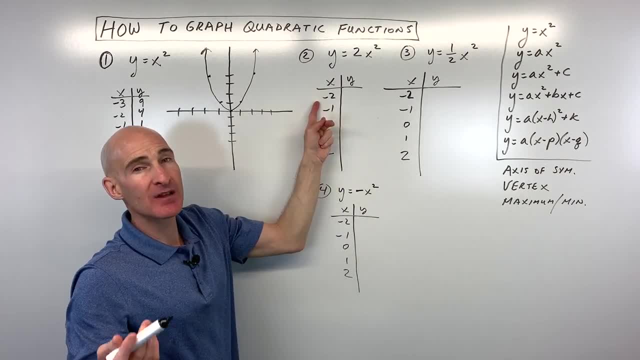 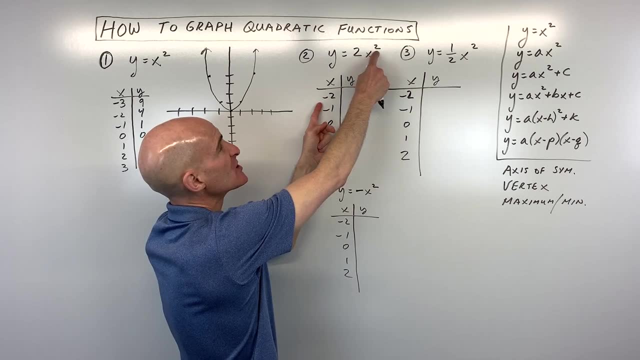 Again, you can make a table. Sometimes what students make a mistake is they're going to think about working from left to right. You want to think of doing the order of operations, the PEMDAS. So if we put negative two in here and we square it, negative two squared is 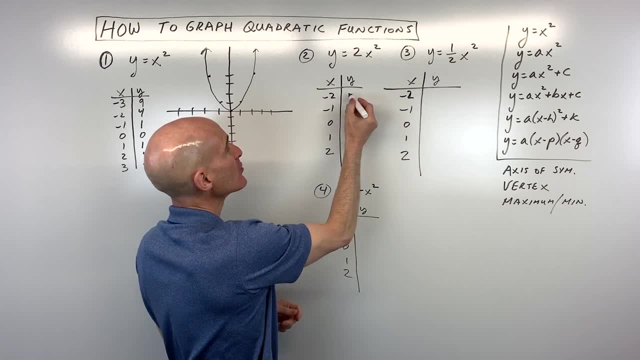 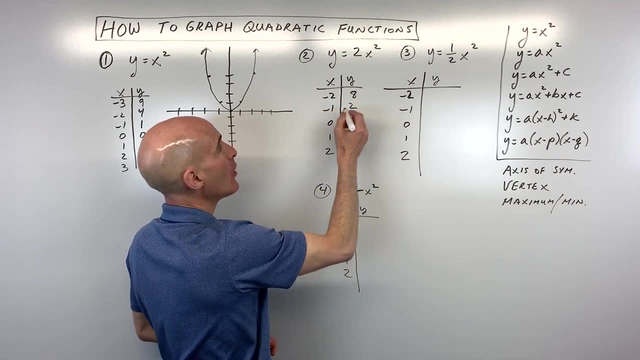 negative two times negative. two, which is four times this two here, which gives us eight Negative. one squared is one times two is two. Zero squared is zero times two is zero. One squared is one times two is two, And two squared is four times two is. 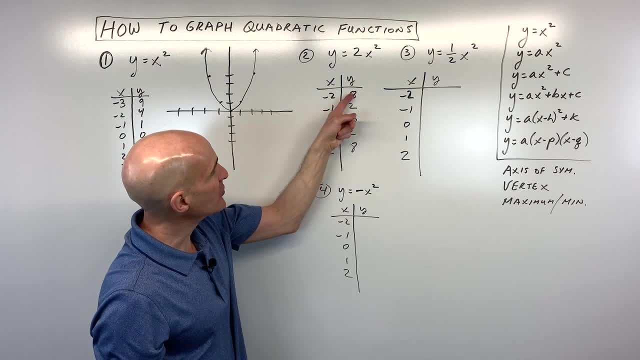 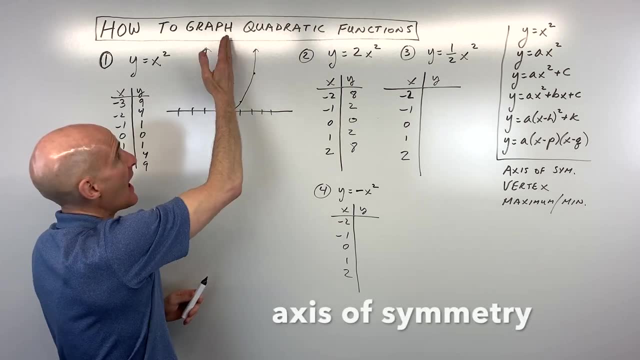 eight. Now, one thing that you'll probably notice is that see how these values here are the same. These values here are the same, And that's because the graph, the equation graph, is symmetric about this axis of symmetry. Now, when we talk about axis of symmetry, 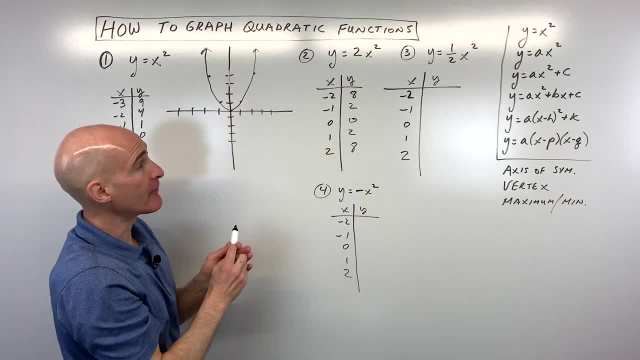 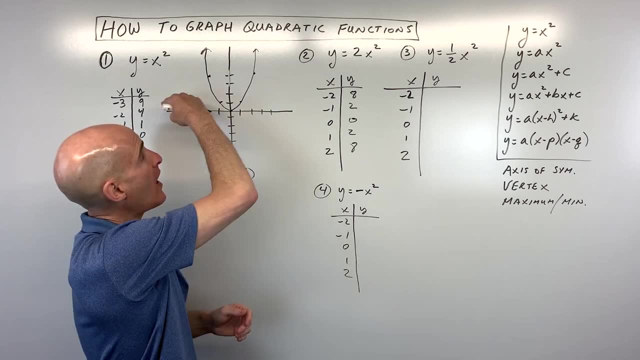 it's this vertical line, okay, that divides the parabola in half In this parent function. that line is the line x equals zero. Remember: x equals lines are vertical lines, whereas y equals lines are the horizontal lines. The other thing I want to talk about and this: 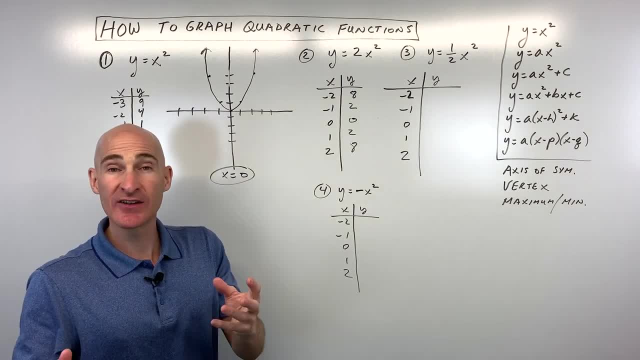 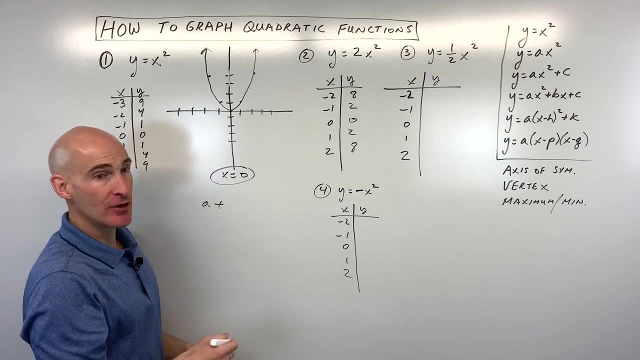 is something that sometimes, when I'm working with students, tutoring students- you know their teachers give them all different little techniques and you might find this helpful. When this a value is positive, you can think about it. when you're positive, what do you? 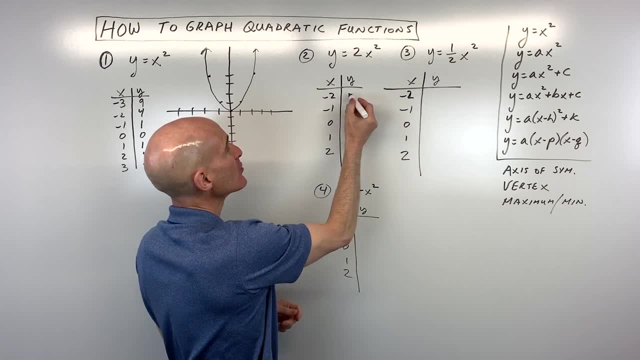 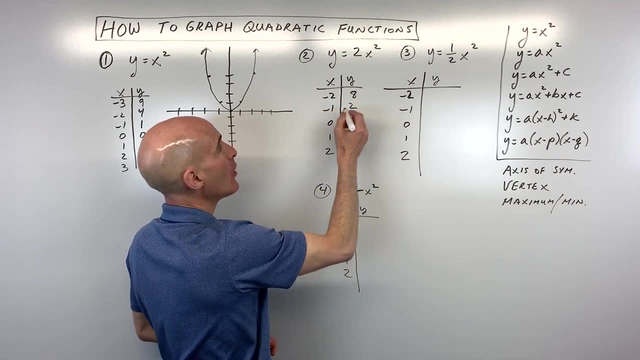 negative two times negative. two, which is four times this two here, which gives us eight Negative. one squared is one times two is two. Zero squared is zero times two is zero. One squared is one times two is two, And two squared is four times two is. 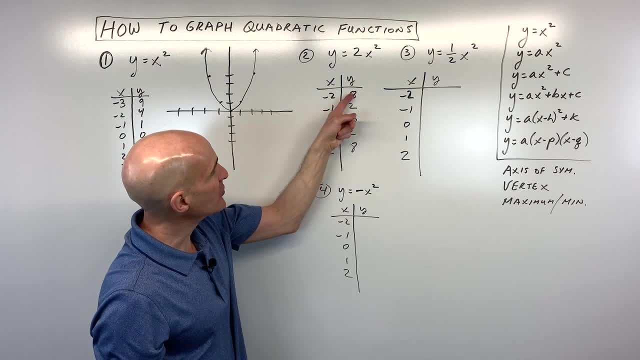 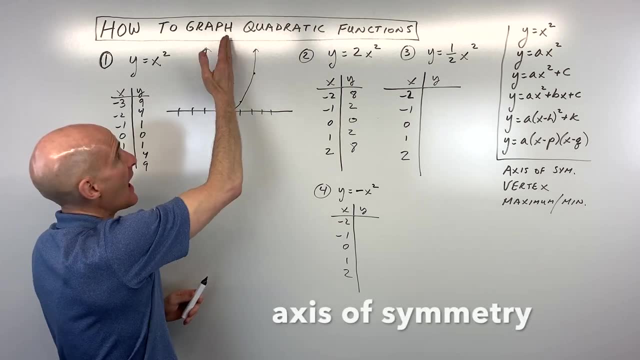 eight. Now, one thing that you'll probably notice is that see how these values here are the same. These values here are the same, And that's because the graph, the equation graph, is symmetric about this axis of symmetry. Now, when we talk about axis of symmetry, 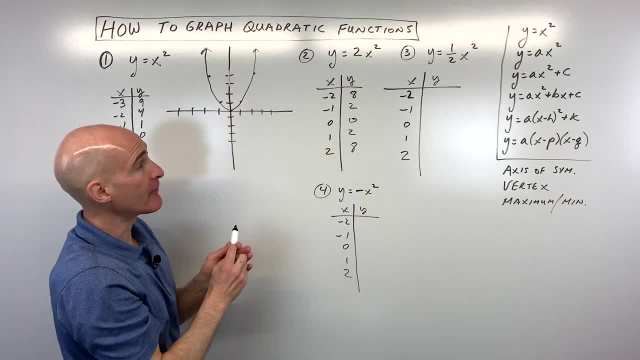 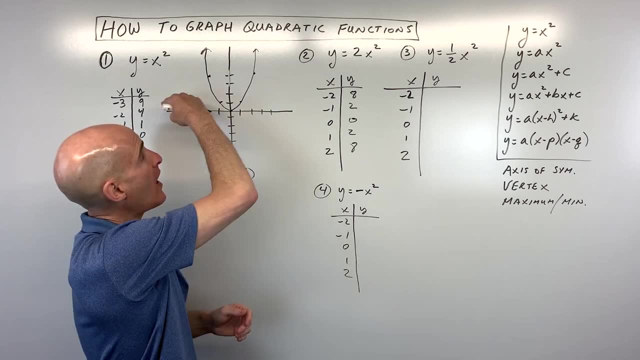 it's this vertical line, okay, that divides the parabola in half In this parent function. that line is the line x equals zero. Remember: x equals lines are vertical lines, whereas y equals lines are the horizontal lines. The other thing I want to talk about and this: 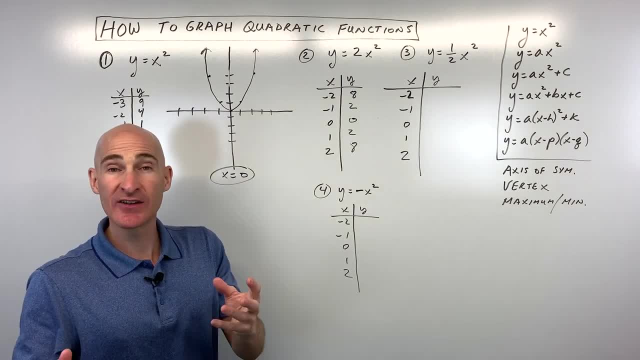 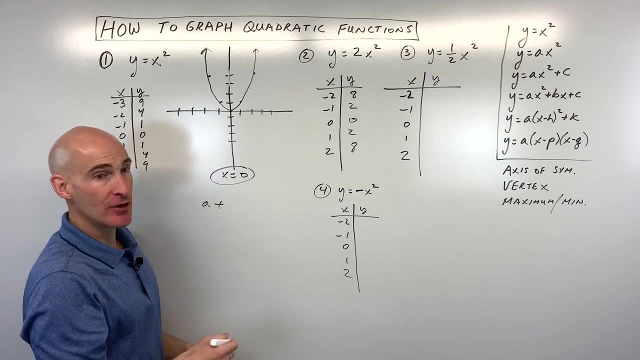 is something that sometimes, when I'm working with students, tutoring students- you know their teachers give them all different little techniques and you might find this helpful. When this a value is positive, you can think about it. when you're positive, what do you? 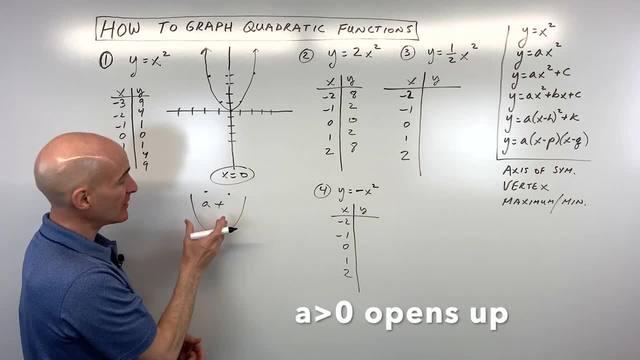 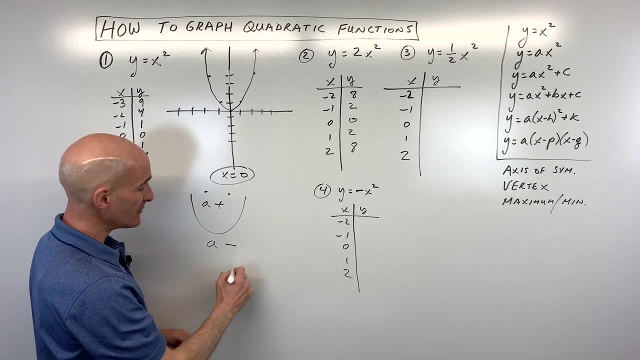 do You smile? right, So you can think of a as positive. that opens up. see that smile, There we go. Whereas if you think about being negative, right say, if the a value is negative, opening down. See how this is kind of like a frown. okay, opening down So you could. 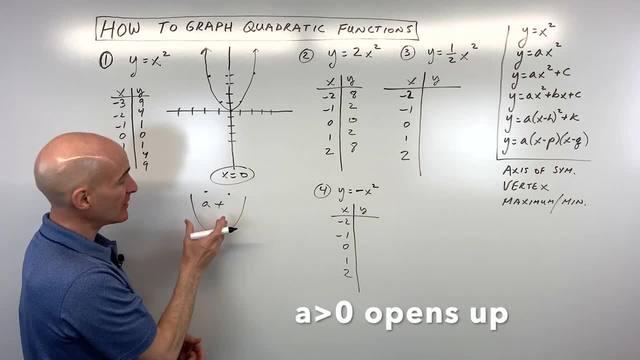 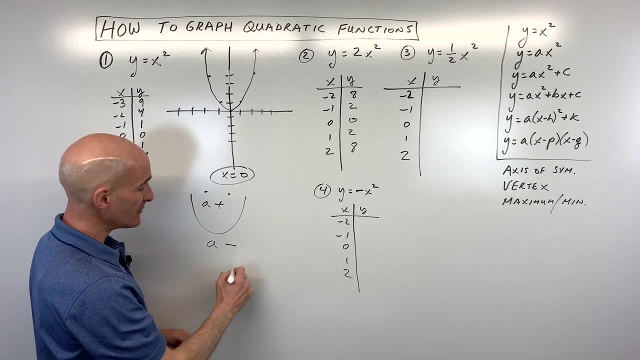 do You smile? right, So you can think of a as positive. that opens up. see that smile, There we go. Whereas if you think about being negative, right say, if the a value is negative, opening down. See how this is kind of like a frown. okay, opening down So you could. 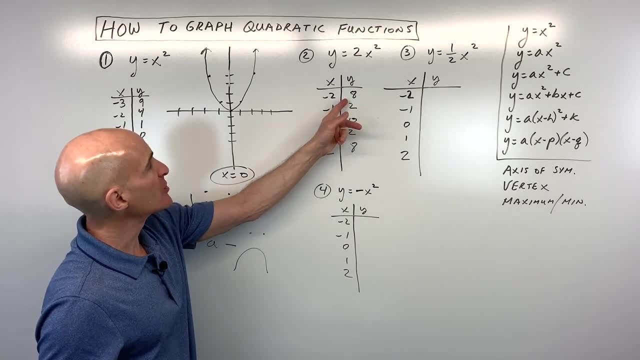 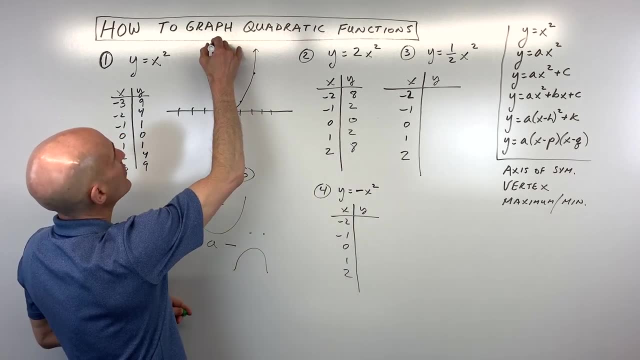 use that as a way of kind of remembering, if that helps you. But let's go ahead and plot these points. I'm going to switch colors here. Let's go to green and we've got- let's see- negative two, eight, which is way up here. We've got negative one, two, which is right. 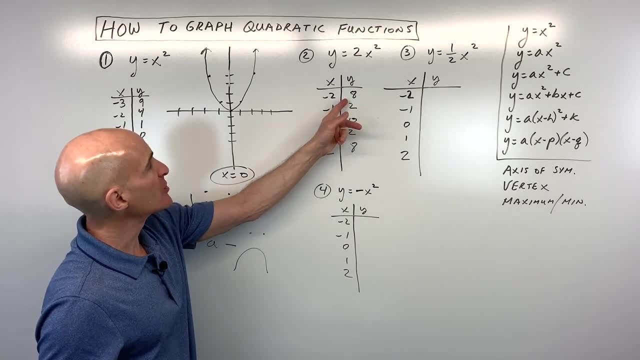 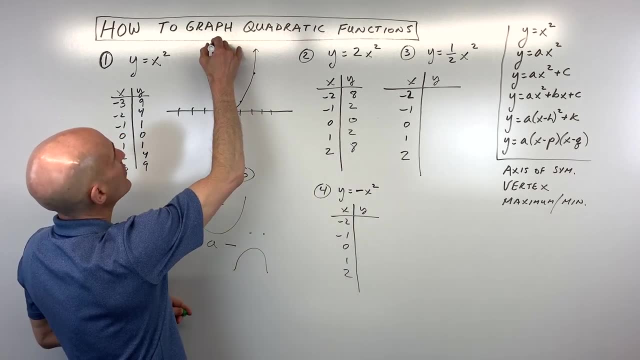 use that as a way of kind of remembering, if that helps you. But let's go ahead and plot these points. I'm going to switch colors here. Let's go to green and we've got- let's see- negative two, eight, which is way up here. We've got negative one, two, which is right. 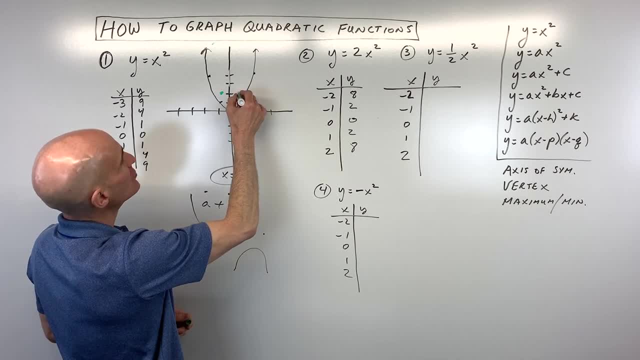 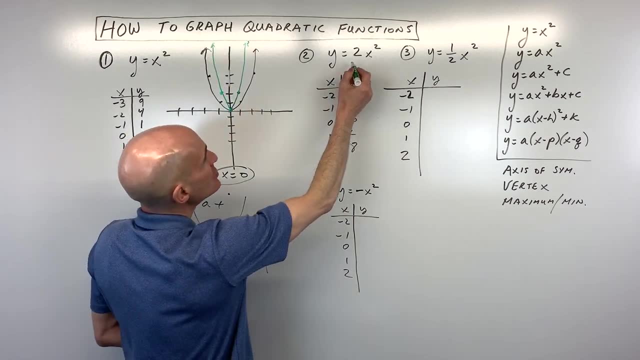 here: Zero, zero which is here, One, two which is here and two eight, which is way up here. So, when you look at this graph, what do you notice? Well, the two. okay, that a. 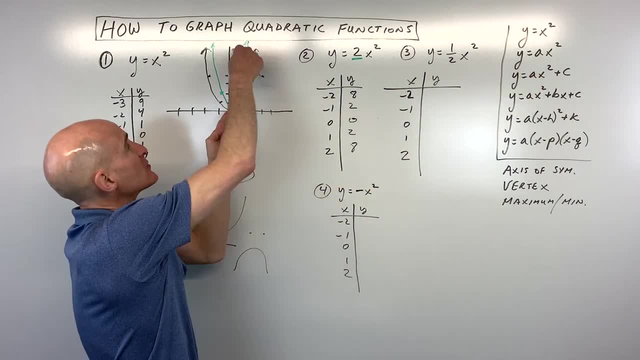 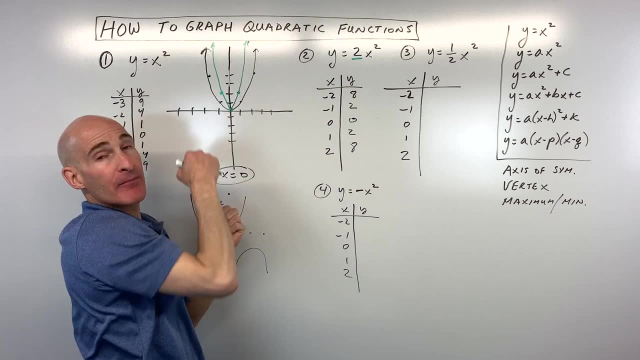 value is greater than one. so it's a vertical stretch, which means that the graph is going up faster. Some people refer to this as being narrower, but I just like to think of it as a vertical stretch. like you're pulling it up vertically and that's why it's you know. 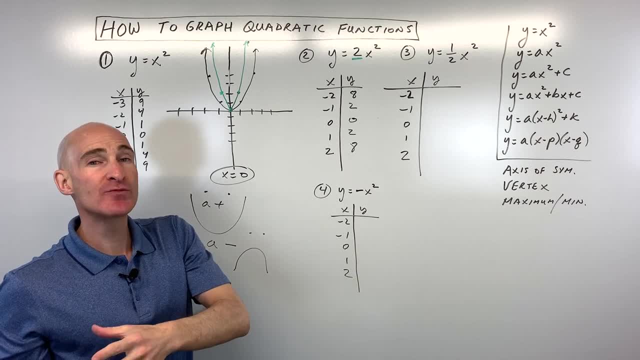 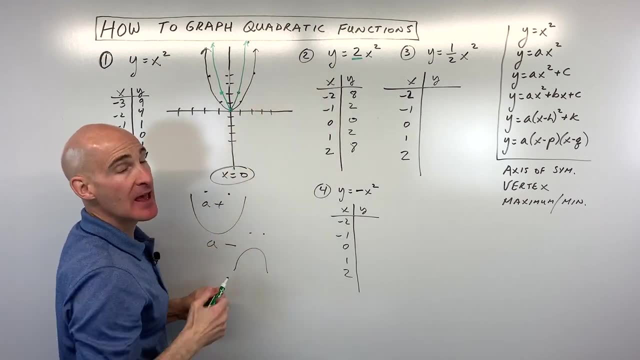 like narrower, like that. The other thing that comes up when you're doing these problems is domain and range. So when you think about domain, you think about what can the x values be? So I usually look from left to right. And when you think about the range, you think: 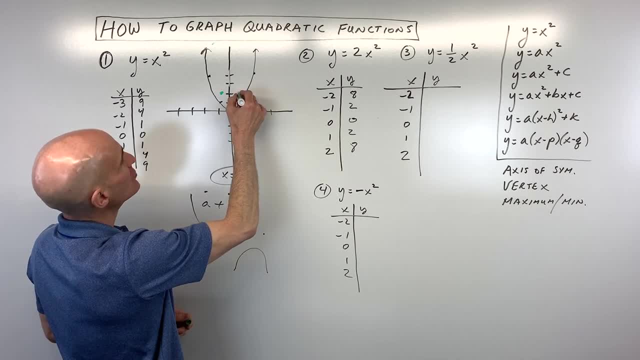 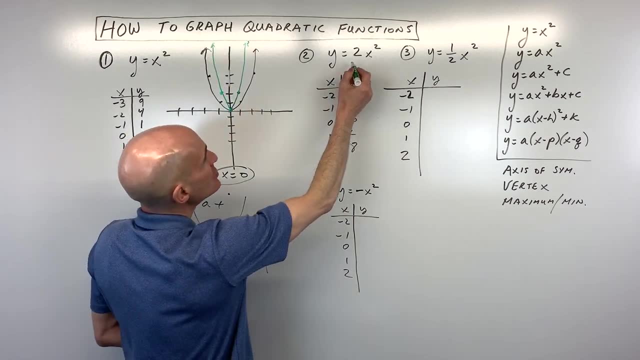 here: Zero, zero which is here, One, two which is here and two eight, which is way up here. So, when you look at this graph, what do you notice? Well, the two. okay, that a. 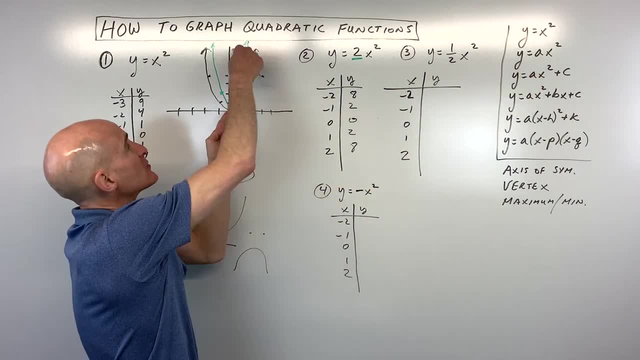 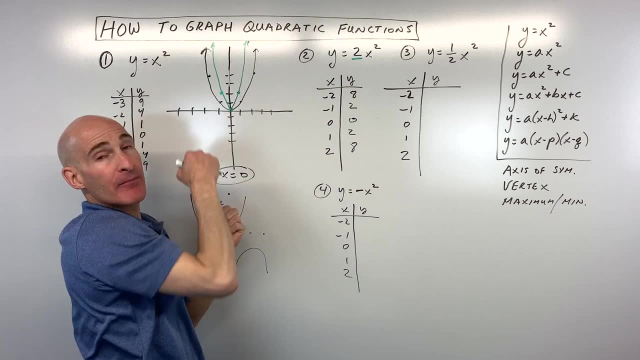 value is greater than one. so it's a vertical stretch, which means that the graph is going up faster. Some people refer to this as being narrower, but I just like to think of it as a vertical stretch. like you're pulling it up vertically and that's why it's you know. 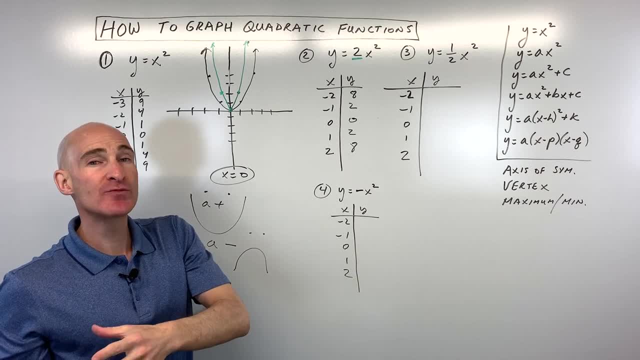 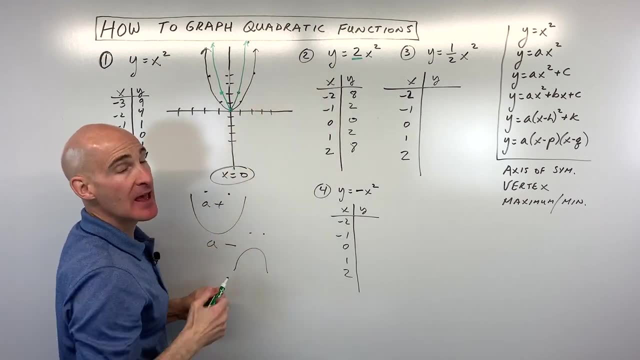 like narrower, like that. The other thing that comes up when you're doing these problems is domain and range. So when you think about domain, you think about what can the x values be? So I usually look from left to right. And when you think about the range, you think: 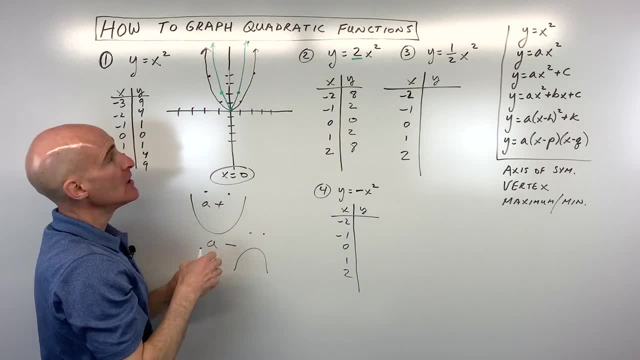 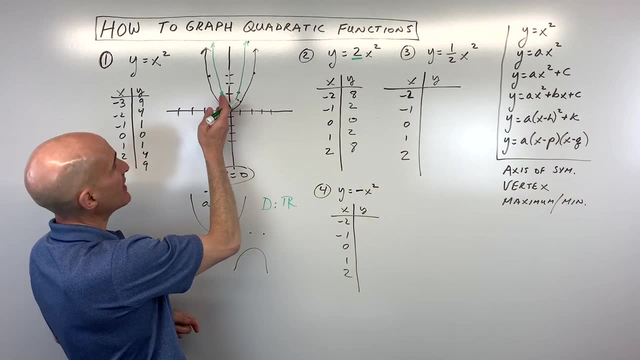 about? what can the y values be? So I kind of think from low to high, With these parabolas that we're going to be working with in this video, the domain is always going to be all real numbers. So that means that x can go all the way to negative infinity, all the. 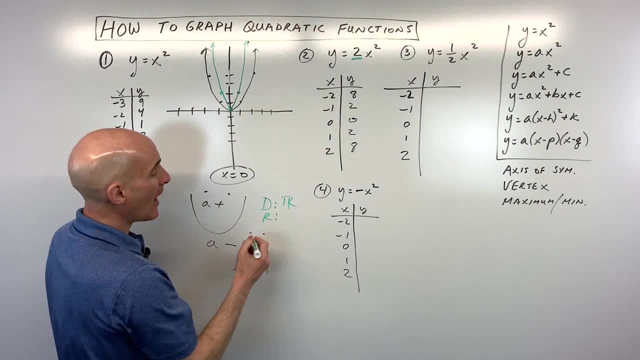 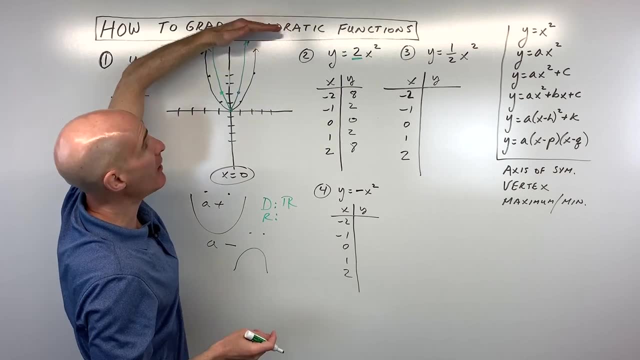 way to positive infinity. When we look at the range- okay the y values- you can see that negative over here it is equal to zero. it just touches right at the x axis and it's above the x axis. So we say that the range is y is greater than or equal to zero If 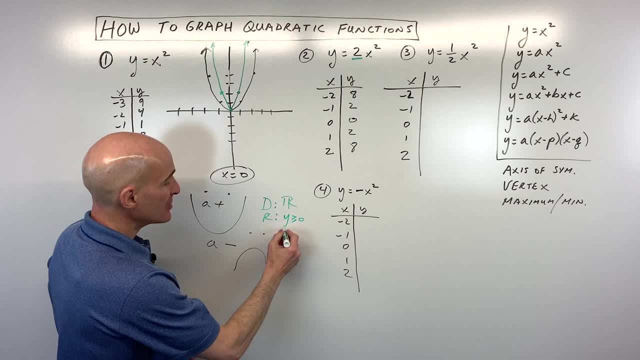 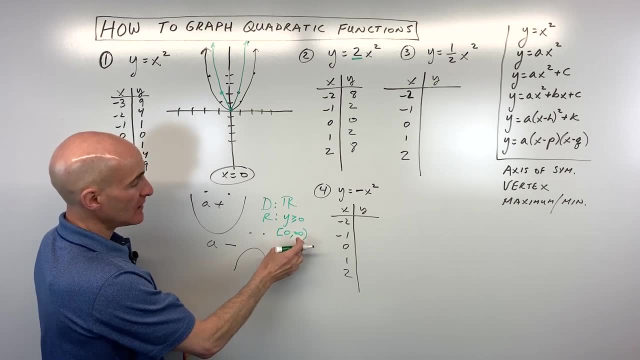 you're using the interval notation as you go on. in math it's going to be looking something like this: where it's equal to zero all the way up to positive infinity can never reach infinity. that's an open interval here on the right. So we're going to work with inequalities. 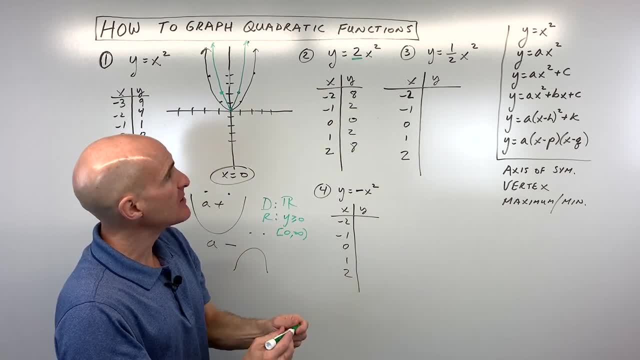 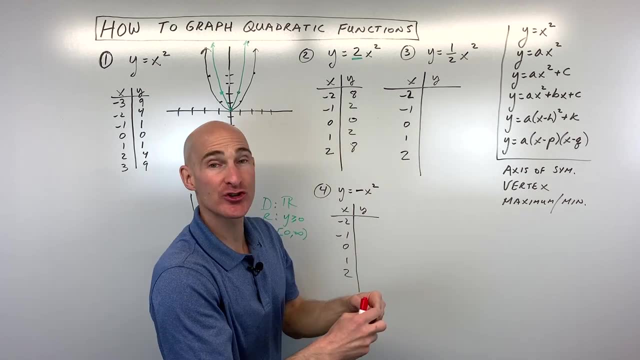 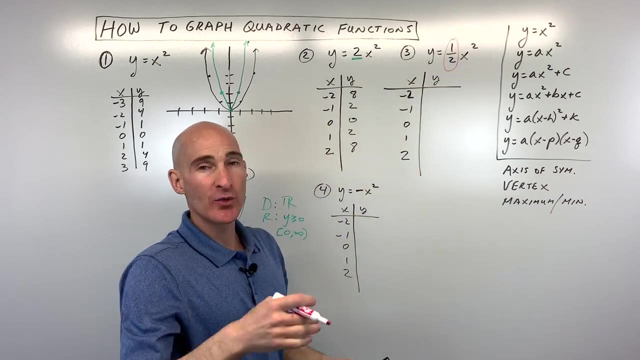 though, for this video. So let's go to number three. Now, what do you think happens here? with y equals one half x squared? Well, if you said that the one half is going to be a vertical shrink, you're absolutely right. And that's again it's because this a value here is between zero and one. So when 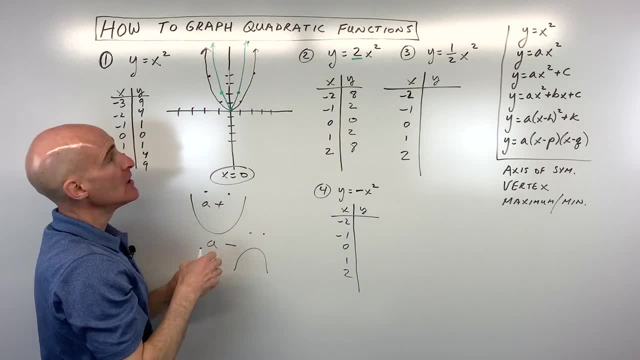 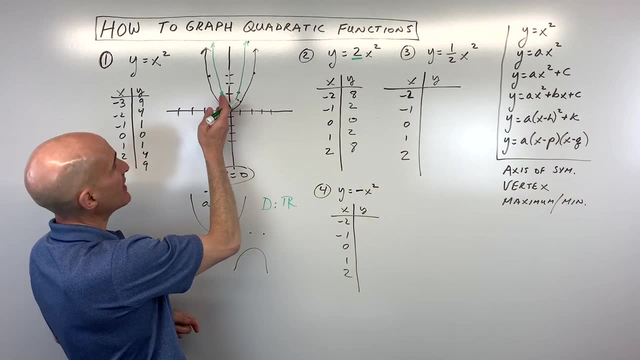 about? what can the y values be? So I kind of think from low to high, With these parabolas that we're going to be working with in this video, the domain is always going to be all real numbers. So that means that x can go all the way to negative infinity, all the. 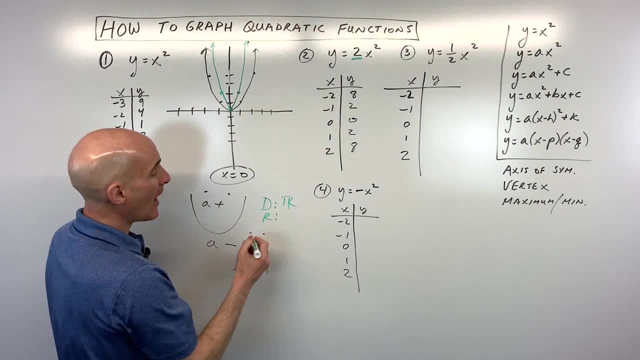 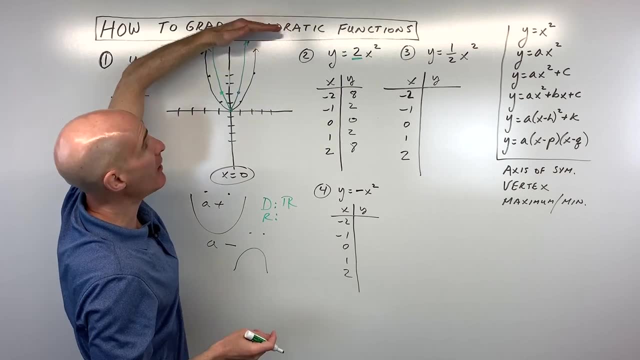 way to positive infinity. When we look at the range- okay the y values- you can see that negative over here it is equal to zero. it just touches right at the x axis and it's above the x axis. So we say that the range is y is greater than or equal to zero If 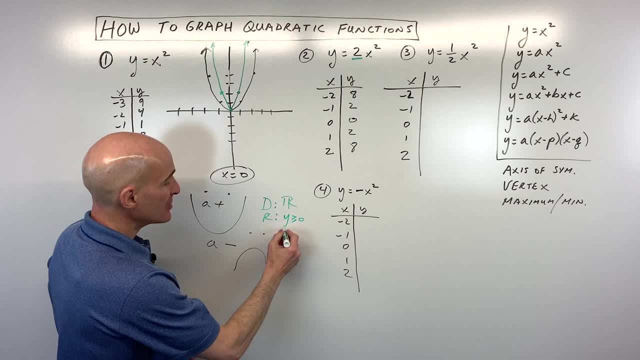 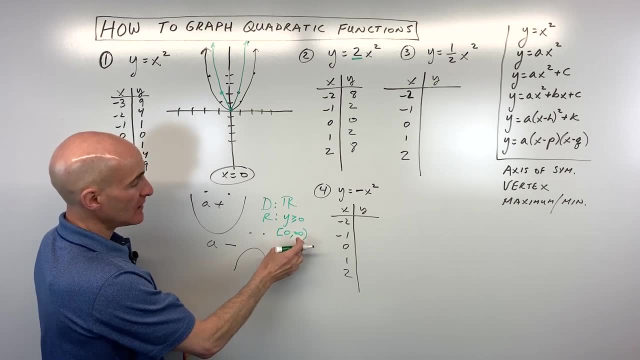 you're using the interval notation as you go on. in math it's going to be looking something like this: where it's equal to zero all the way up to positive infinity can never reach infinity. that's an open interval here on the right. So we're going to work with inequalities. 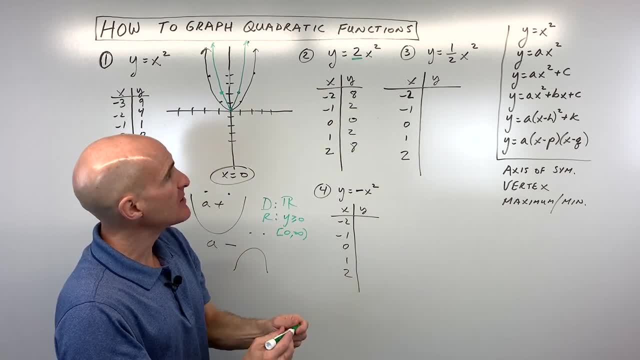 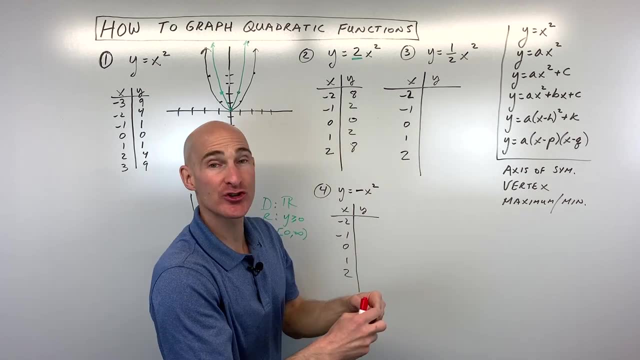 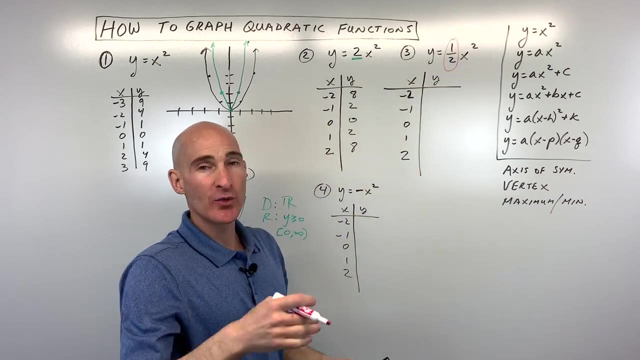 though, for this video. So let's go to number three. Now, what do you think happens here? with y equals one half x squared? Well, if you said that the one half is going to be a vertical shrink, you're absolutely right. And that's again it's because this a value here is between zero and one. So when 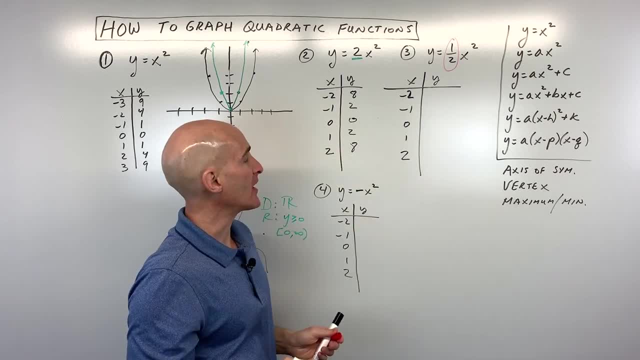 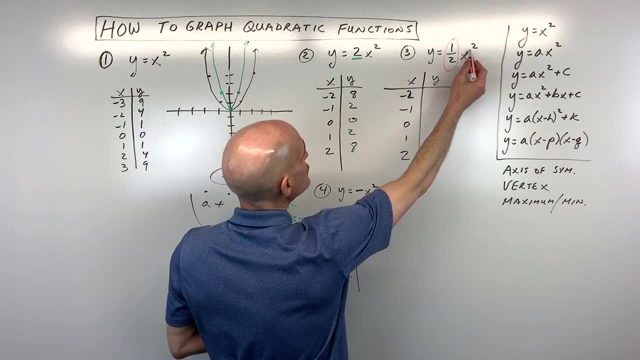 it's less than one like that, but it's still positive. you know it's going to be a vertical shrink. we're going to talk about negative next, So let's go ahead and plot some points here. So we've got negative two. let's see: negative two squared is four times a half. 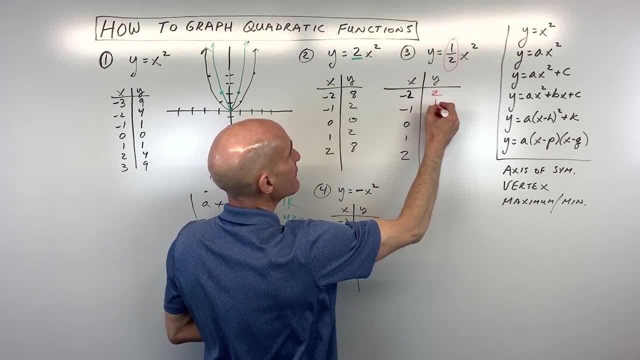 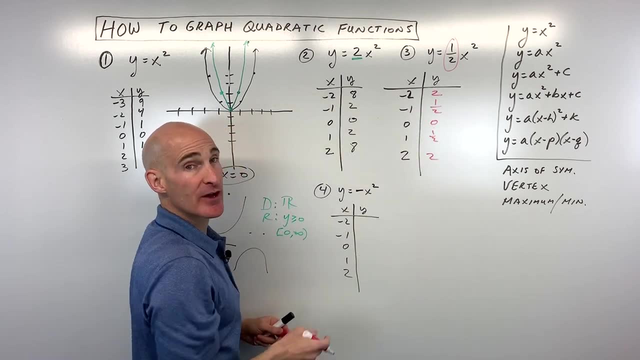 is two negative. one squared is one times a half is a half Zero. squared is zero times a half is zero. And then these are going to be the same. Okay, see how it's symmetric. it's the same on both sides. So let's plot that on the same graph. 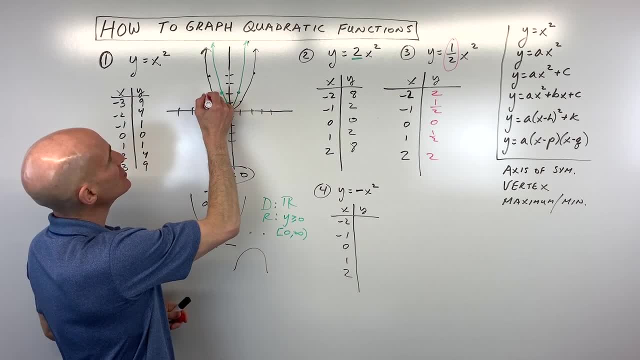 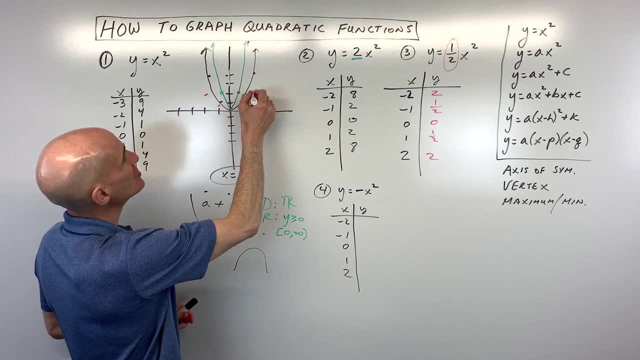 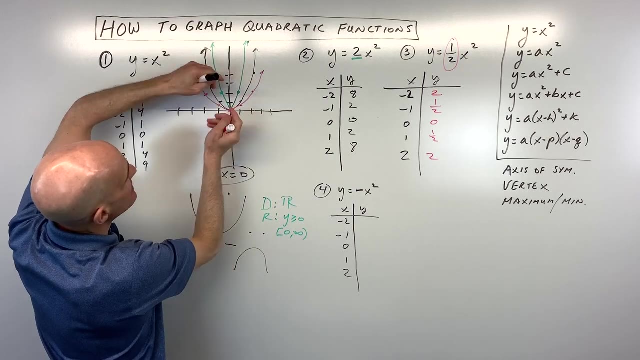 so we can see what this looks like: Negative two, two. negative one a half, zero. zero one a half and two two. So here see the red graph. this is a vertical shrink. So what happened was? it actually made the graph wider. See, the black one was the original one, the. 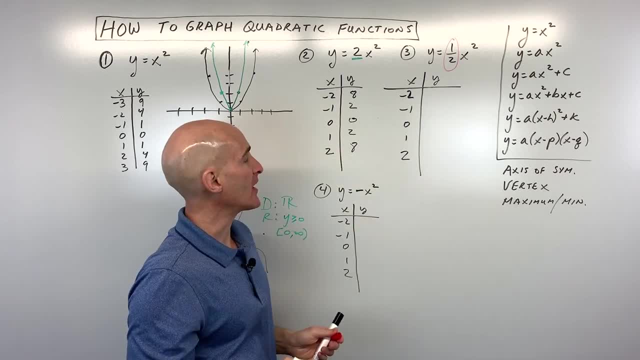 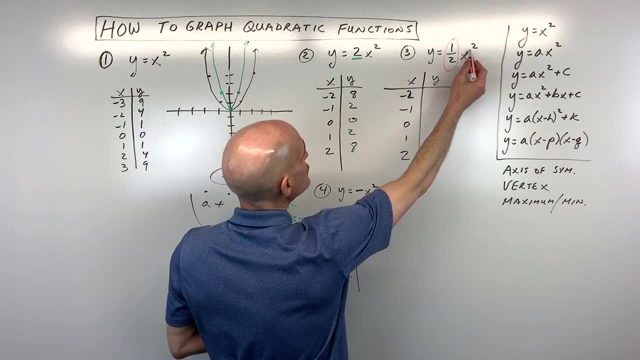 it's less than one like that, but it's still positive. you know it's going to be a vertical shrink. we're going to talk about negative next, So let's go ahead and plot some points here. So we've got negative two. let's see: negative two squared is four times a half. 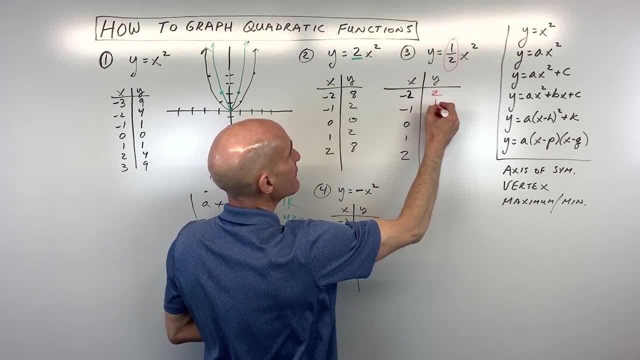 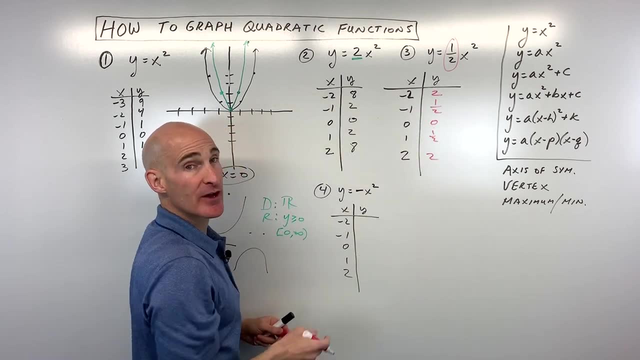 is two negative. one squared is one times a half is a half Zero. squared is zero times a half is zero. And then these are going to be the same. Okay, see how it's symmetric. it's the same on both sides. So let's plot that on the same graph. 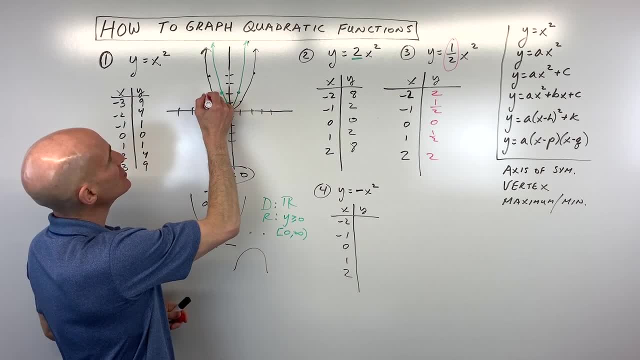 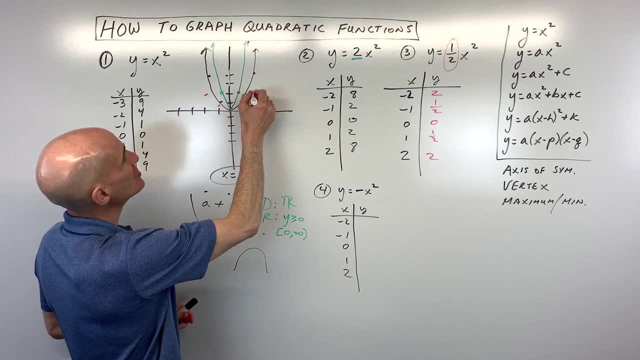 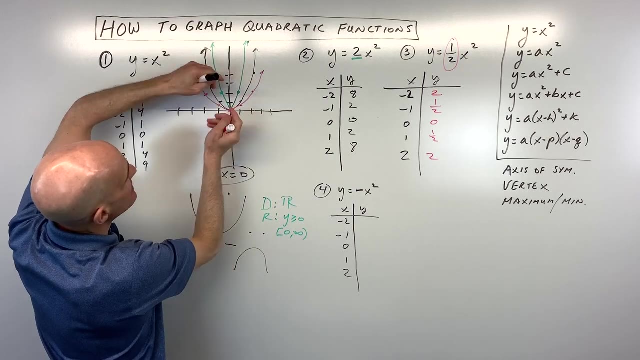 so we can see what this looks like: Negative two, two. negative one a half, zero. zero one a half and two two. So here see the red graph. this is a vertical shrink. So what happened was? it actually made the graph wider. See, the black one was the original one, the. 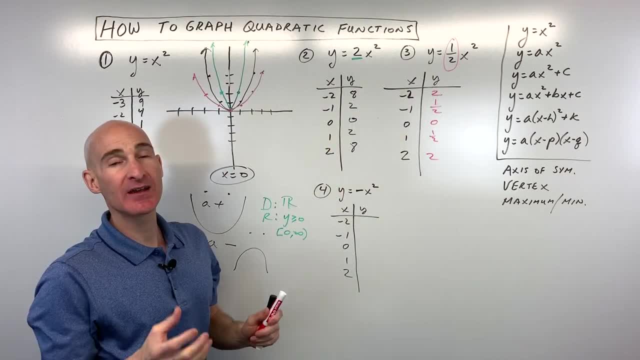 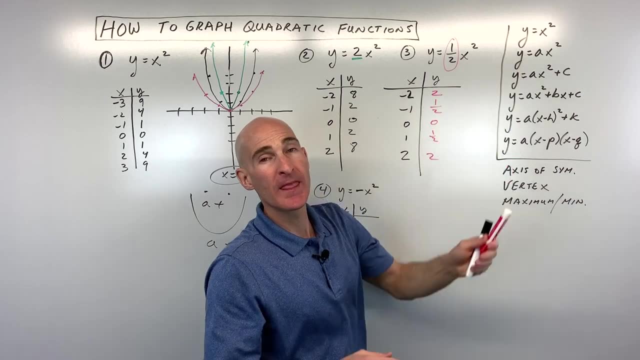 red one is the new one and it's just a vertical shrink. you're compressing it, making it wider. The domain and the range are exactly the same. So these are just. when you're talking about the a value, you're talking about the vertical stretch or shrink. or in number four, where 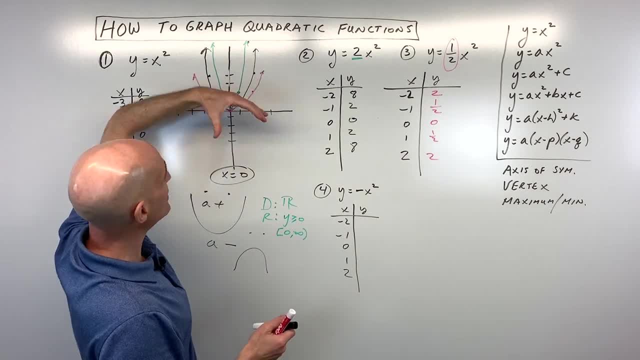 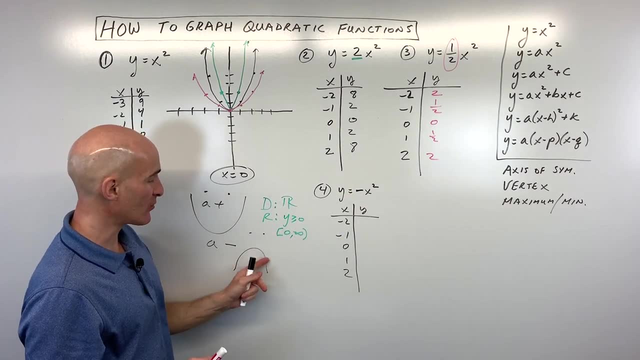 we see that it's negative the a value, then it's going to be a reflection over the x axis and it's going to open downward, Just like we said, when this a value is negative, it's kind of like when a person's negative they're frowning- okay, it's going to be opening downward. 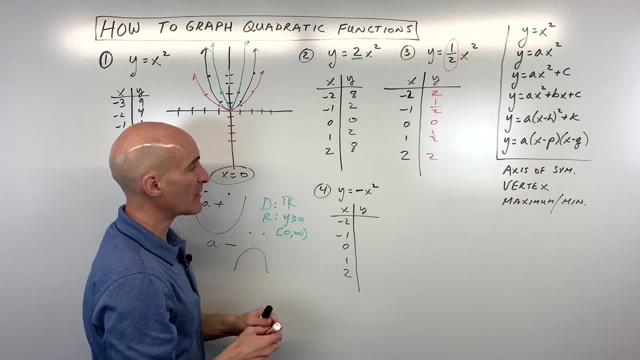 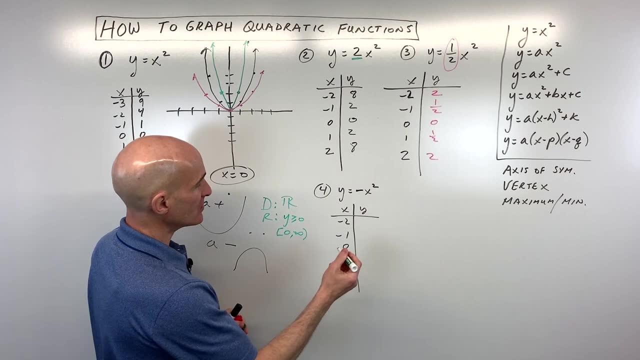 So let's plot a few values here. We're going to get into some more difficult ones here in just a minute, but I just want to lay the foundation here for you so you kind of know how these all work. just working with the parent function. So we've got negative two. 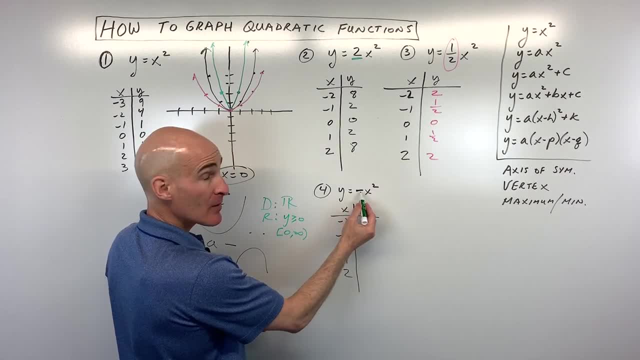 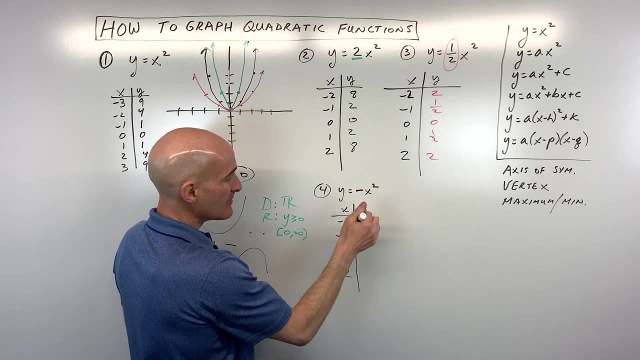 squared, which is four. Now, remember, some people think negative times a negative. well, isn't that a positive, Mario? Well, remember, you want to do the exponents first. So negative two squared is four times a negative is going to give us a negative four Negative one squared. 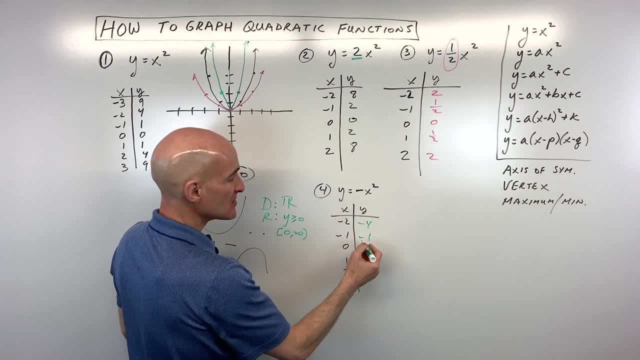 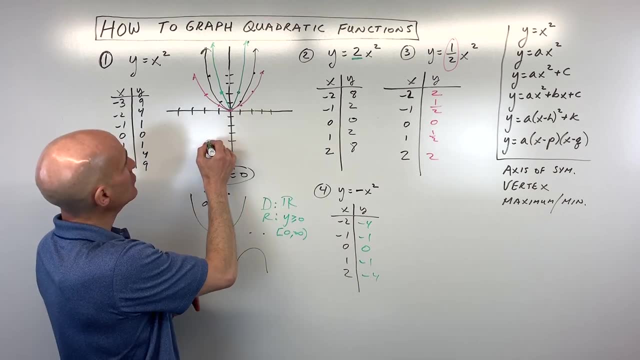 is one times a negative gives us negative one. Zero. squared is zero times a negative is still zero. And then we're getting the same negative one, negative four. So if we plot those negative two, negative four, negative one, negative one, zero, zero one, negative one and two. 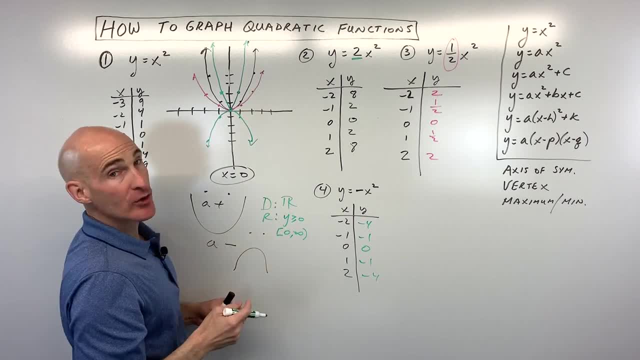 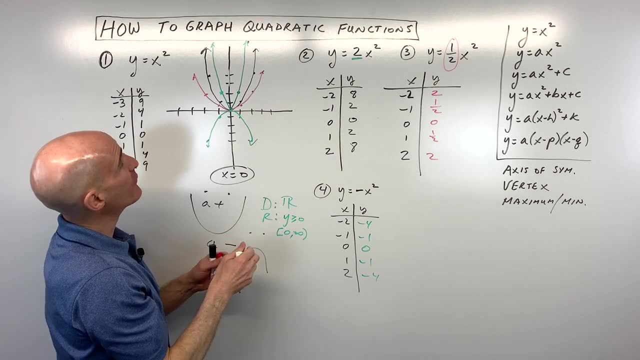 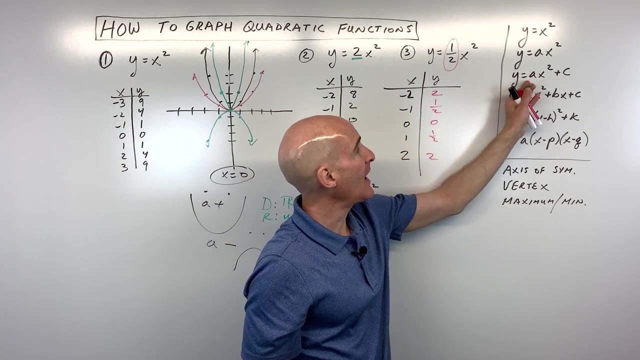 negative four. what you'll notice is that it has the same shape as the original graph. the y equals x squared the parent function: same shape, it's just been reflected over the x axis. All right, so let's dive into some of the ones that involve ax squared plus. 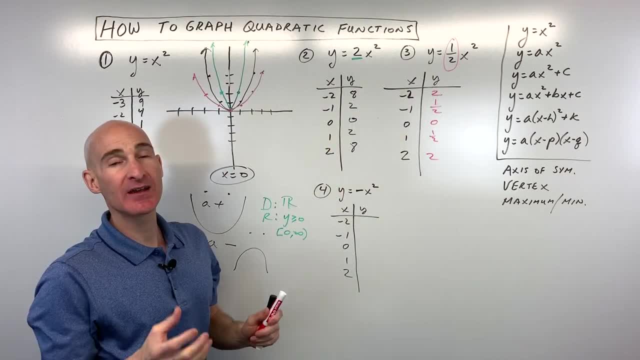 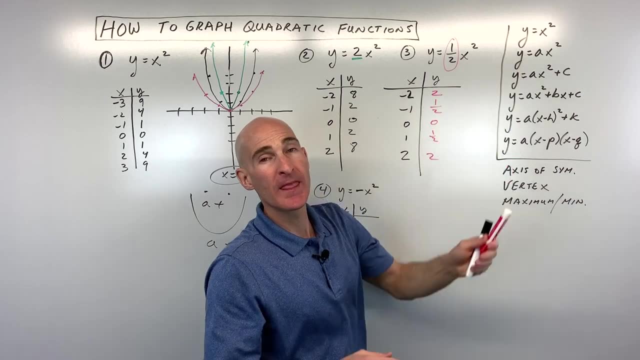 red one is the new one and it's just a vertical shrink. you're compressing it, making it wider. The domain and the range are exactly the same. So these are just. when you're talking about the a value, you're talking about the vertical stretch or shrink. or in number four, where 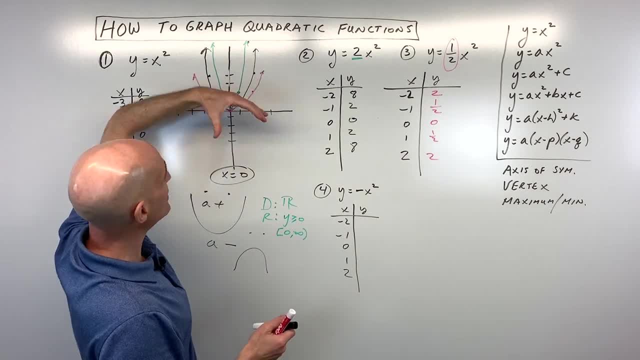 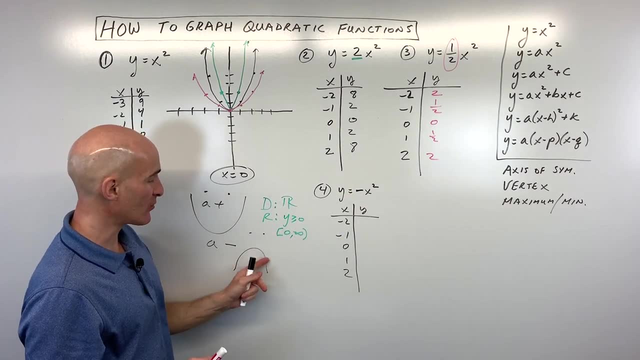 we see that it's negative the a value, then it's going to be a reflection over the x axis and it's going to open downward, Just like we said, when this a value is negative, it's kind of like when a person's negative they're frowning- okay, it's going to be opening downward. 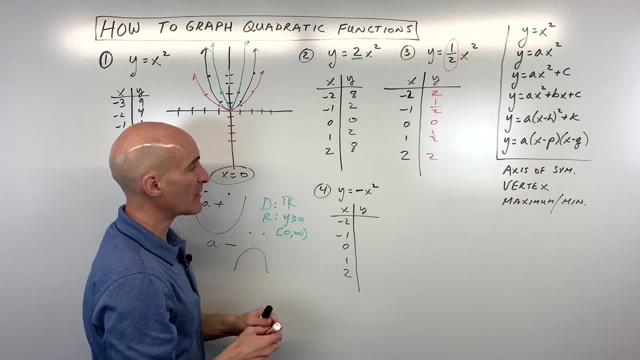 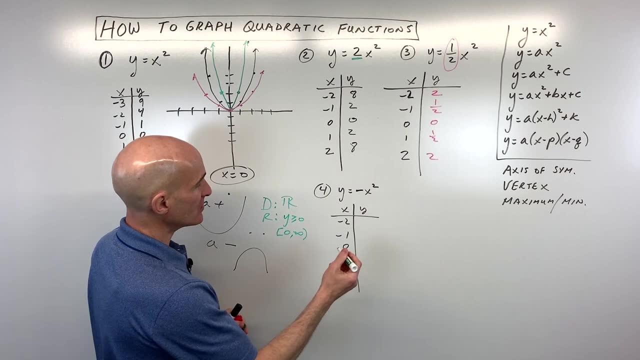 So let's plot a few values here. We're going to get into some more difficult ones here in just a minute, but I just want to lay the foundation here for you so you kind of know how these all work. just working with the parent function. So we've got negative two. 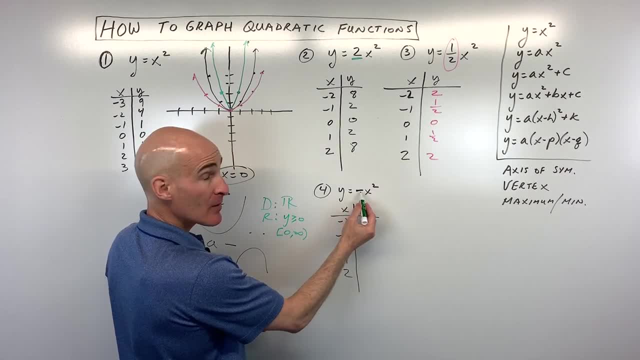 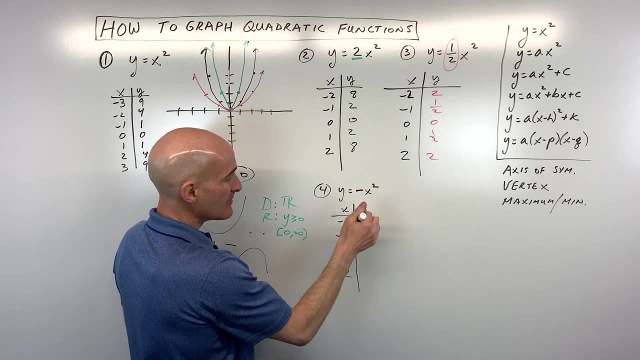 squared, which is four. Now, remember, some people think negative times a negative. well, isn't that a positive, Mario? Well, remember, you want to do the exponents first. So negative two squared is four times a negative is going to give us a negative four Negative one squared. 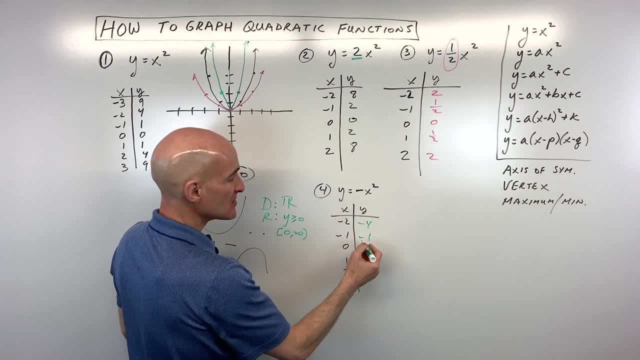 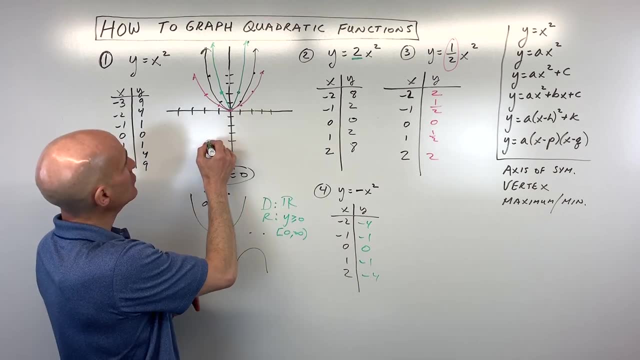 is one times a negative gives us negative one. Zero. squared is zero times a negative is still zero. And then we're getting the same negative one, negative four. So if we plot those negative two, negative four, negative one, negative one, zero, zero one, negative one and two. 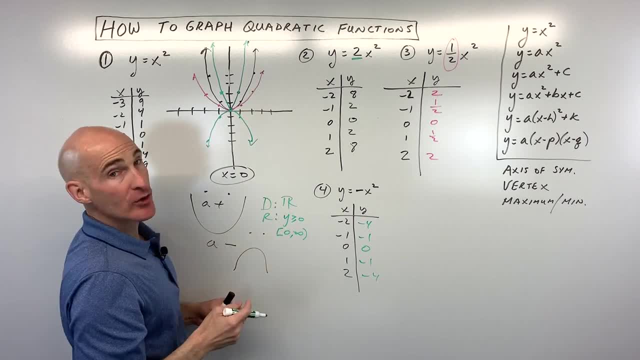 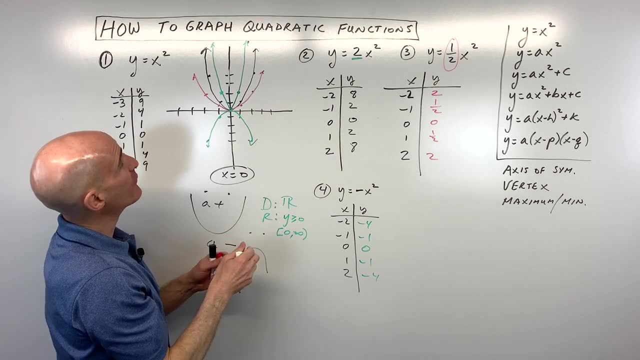 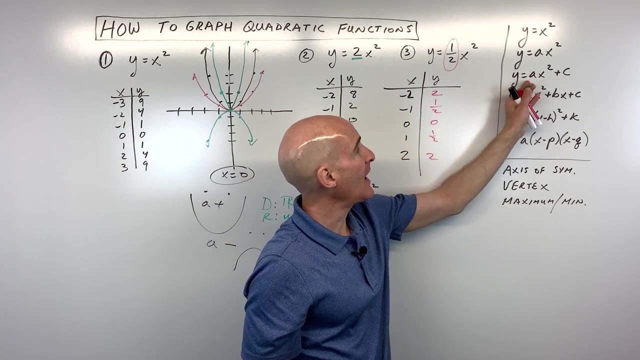 negative four. what you'll notice is that it has the same shape as the original graph. the y equals x squared the parent function: same shape, it's just been reflected over the x axis. All right, so let's dive into some of the ones that involve ax squared plus. 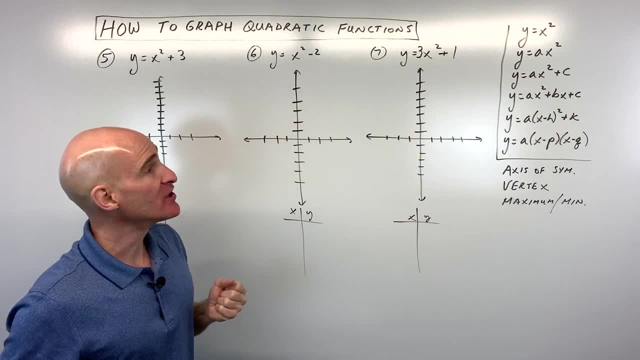 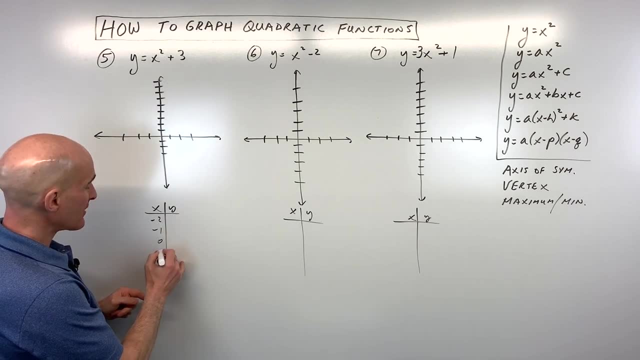 c next. Now, what do you think that c value does to the graph? Well, let's take a look in number five. So I'm going to make a table. I'm going to pick, like I did before, just some small numbers, a couple negative and a couple positive, and let's take a look. 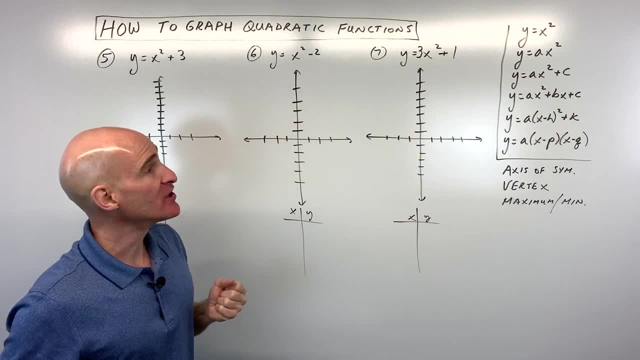 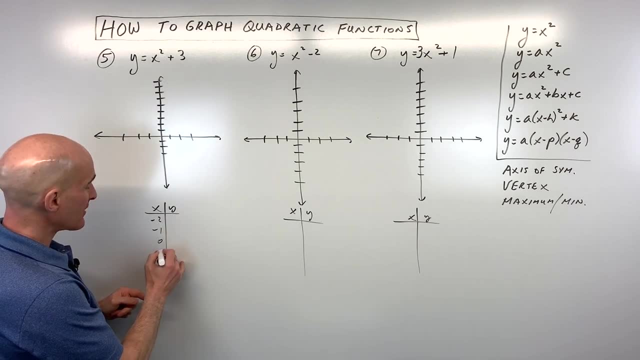 c next. Now, what do you think that c value does to the graph? Well, let's take a look in number five. So I'm going to make a table. I'm going to pick, like I did before, just some small numbers, a couple negative and a couple positive, and let's take a look. 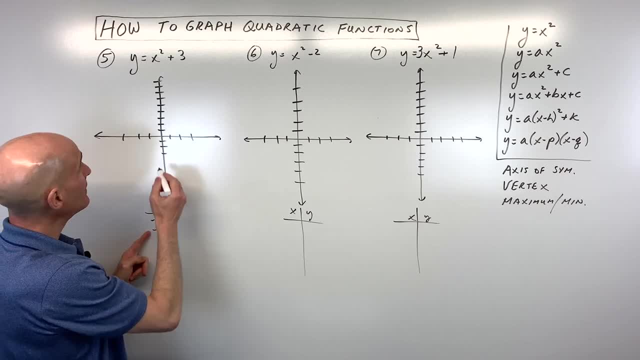 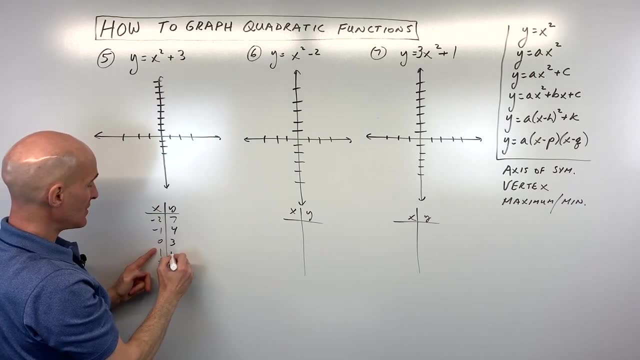 So I put negative two in negative. two squared is four plus three is seven. negative one squared is one plus three is four. zero squared is zero plus three is three. one squared is one plus three is four and two squared is four plus three is seven. Let's go ahead. 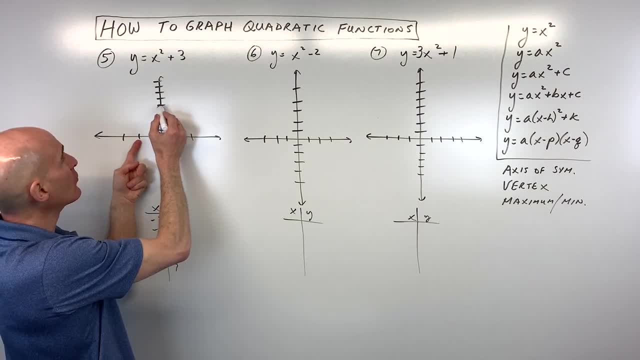 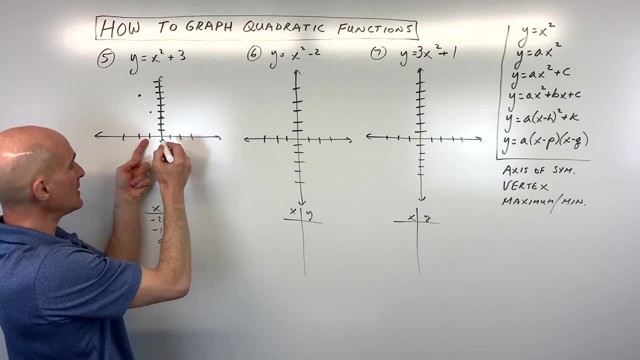 and plot these. We've got negative two, seven, one, two, three, four, five, six, seven right about there, negative one, four right about there, zero, three, one four and two seven. So there's. 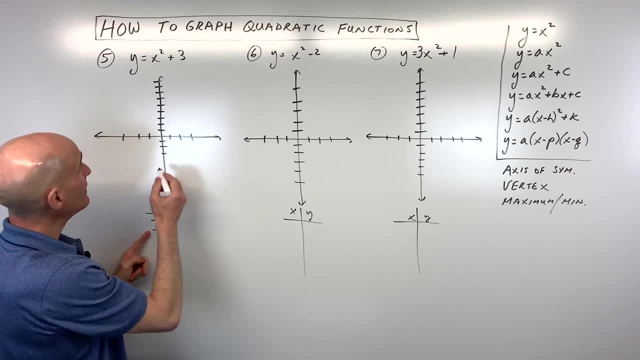 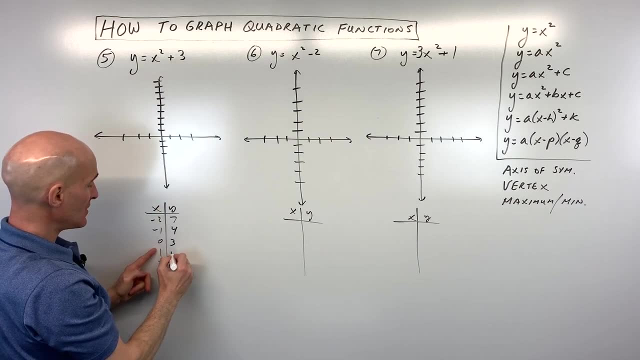 So I put negative two in negative. two squared is four plus three is seven. negative one squared is one plus three is four. zero squared is zero plus three is three. one squared is one plus three is four and two squared is four plus three is seven. Let's go ahead. 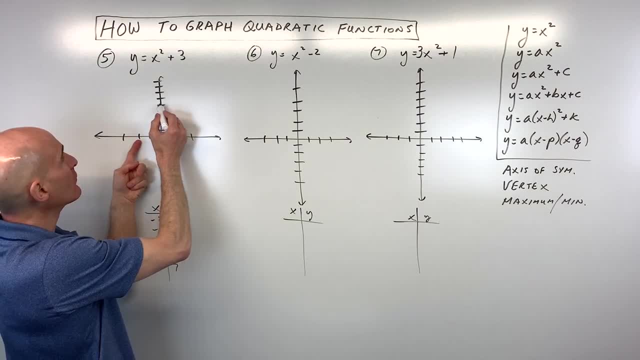 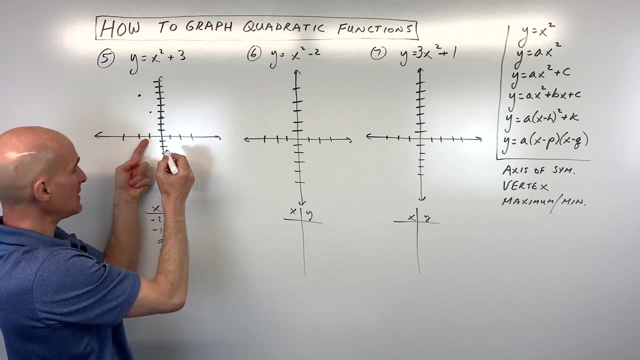 and plot these: Two, seven, one, two, three, four, five, six, seven, right about there. negative, one, four, right about there, zero, three, one, four and two, seven. So there's our graph, and 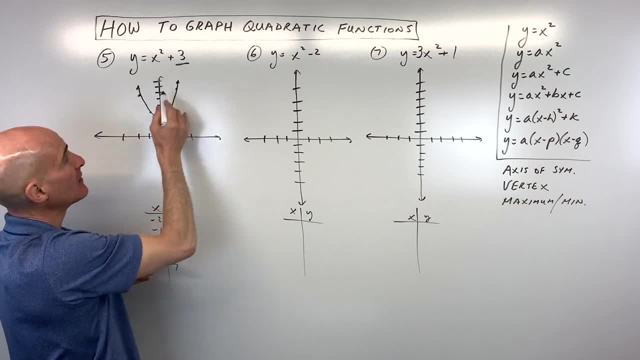 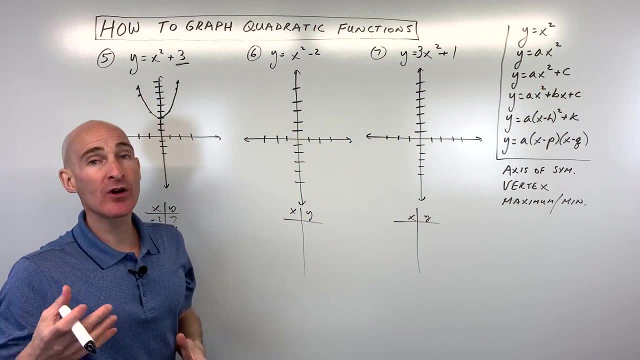 notice this: three: see how it crosses the y axis right at three. So what this did here? the three? the c value picked up the graph and it moved it up three. so that's what we call a translation, or a slide, or a shift. 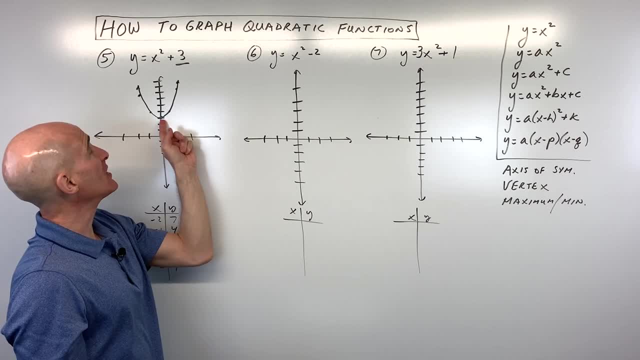 Usually, translation is a translation of a graph, but it's a translation of a graph. probably the more proper term is shifting up three units. Now, if you look at this, y equals x squared. that's our basic parent function that we talked about in the very 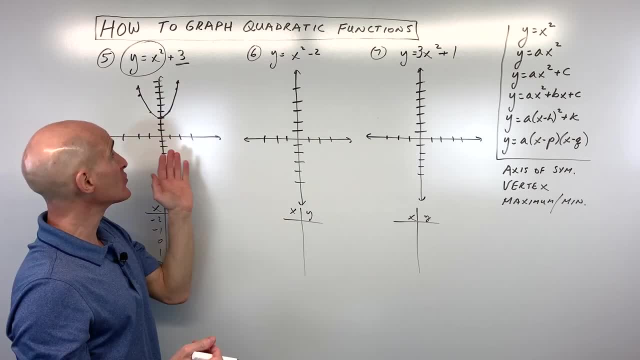 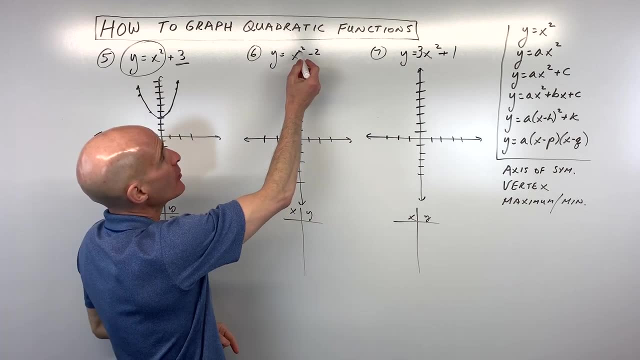 first problem. we just picked it up and moved it up three. So that's for number five. Number six now: what do you think happens here? y equals x squared minus two. Well, you're probably saying, Mario, I see that y equals x squared again, but that minus two is going to shift. 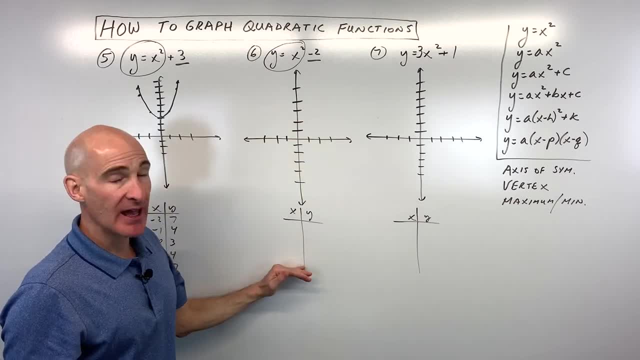 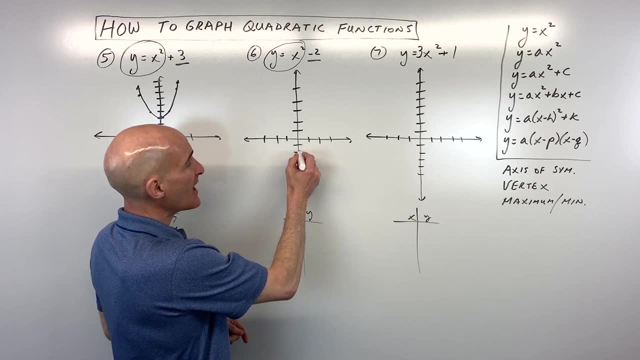 down two, right. So what you can do is you can make a table again. but if you're starting to catch on to the pattern here and say, well, I know this just shifts down two, why don't I just pretend like negative two? here is my new origin, my new starting point- Then I can make a table just using 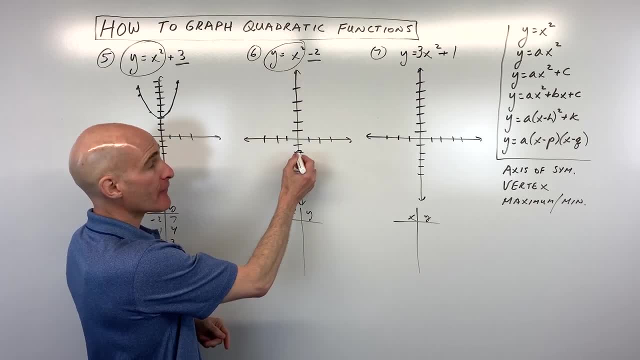 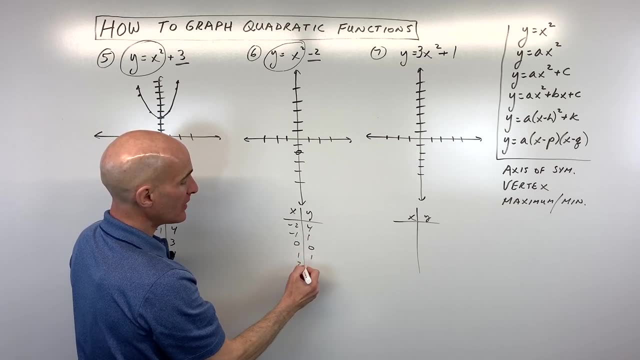 my parent function, y equals x squared and plot from here. So let's go ahead and do that. So this would be negative: two four. negative one. a one, zero, zero one, one and two four. 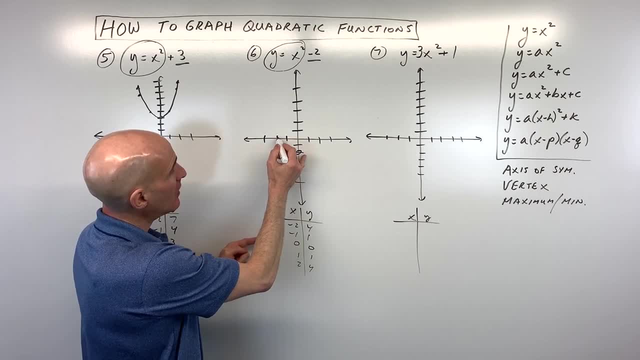 I'm going to plot these points from here now. So I'm going left two up four, left one up one, zero, zero one. I'm going to plot these points from here now. So I'm going left two up four, left one up one, zero, zero one and two four. 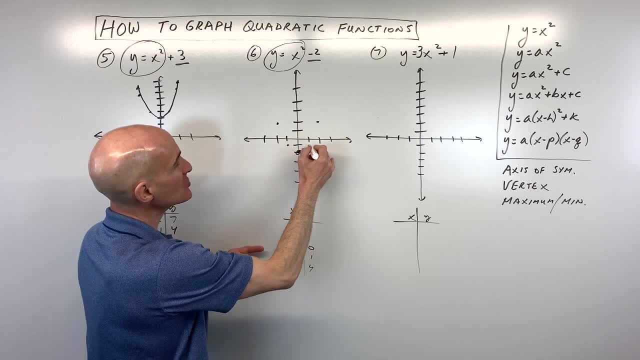 0, 0, write 1 up 1 and write 2 up 4.. Now you don't have to do it this way. If you don't feel comfortable, you can use the whole equation, But just remember when you use the whole equation: 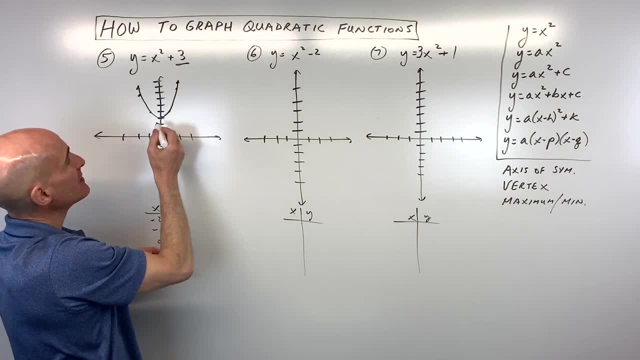 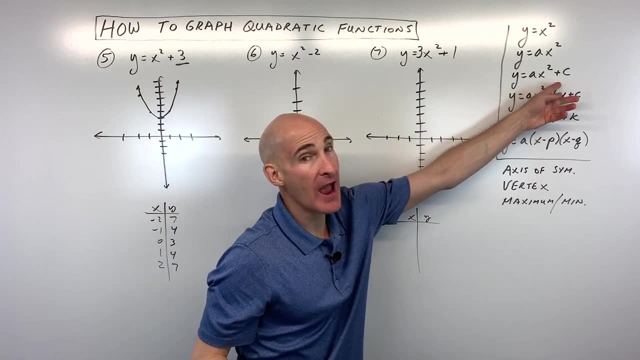 our graph and notice this: three, see how it crosses the y axis right at three. So what this did here? the three, the c value picked up the graph and it moved it up three. so that's what we call a translation, or a slide, or a shift. 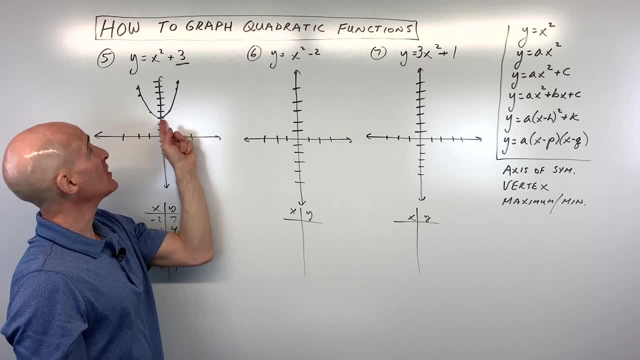 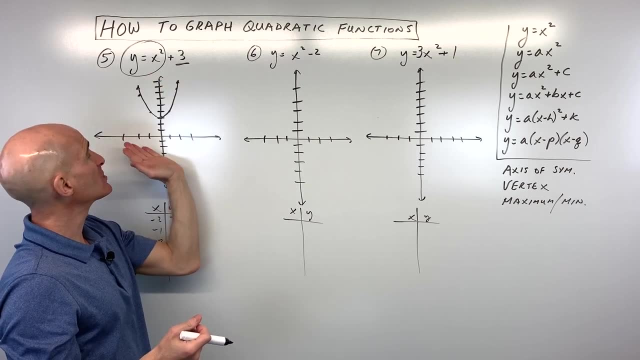 Usually, translation is probably the more proper term. it's shifting up three units. Now, if you look at this, y equals x squared. that's our basic parent function that we talked about in the very first problem. we just picked it up and moved it up three. So that's for. 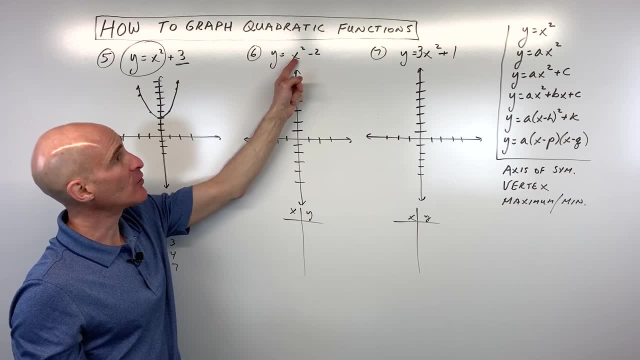 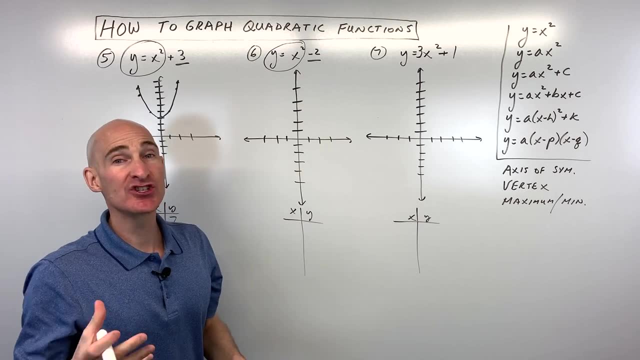 number five, Number six. now, what do you think happens here? Y equals x squared minus two. Well, you're probably saying, Mario, I see that y equals x squared again, but that minus two is going to shift down two, right? So what you can do is you can make a table again. 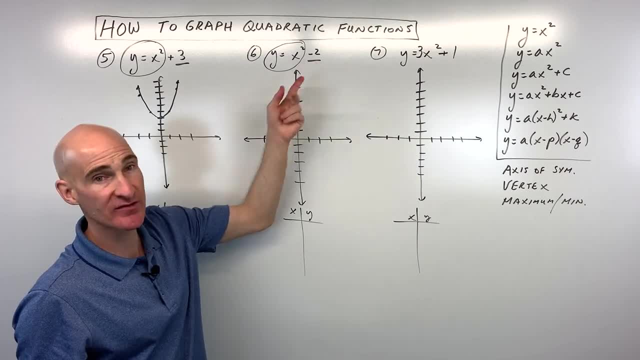 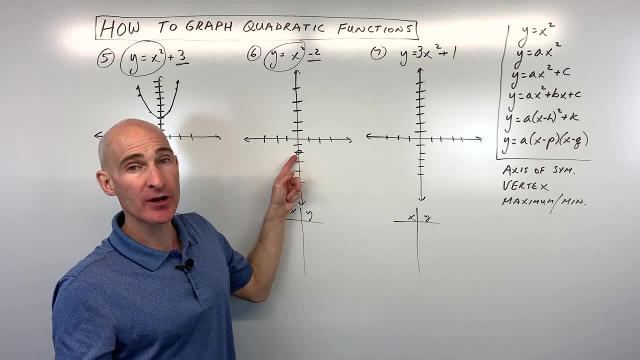 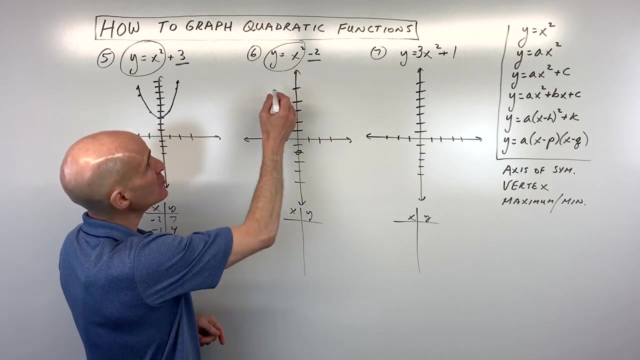 but if you're the pattern here you can say: well, I know, this just shifts down two. Why don't I just pretend like negative two? here is my new origin, my new starting point. Then I can make a table just using my parent function- y equals x squared- and plot from here. So let's go ahead and do that. So this: 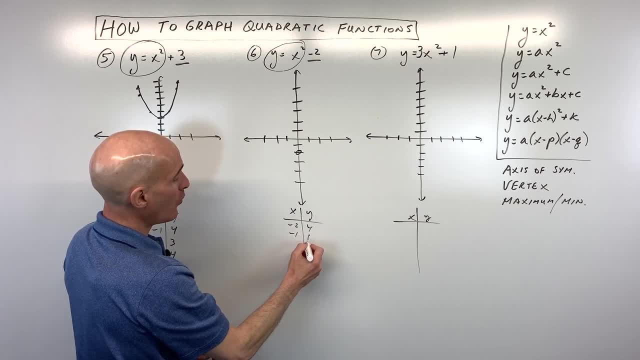 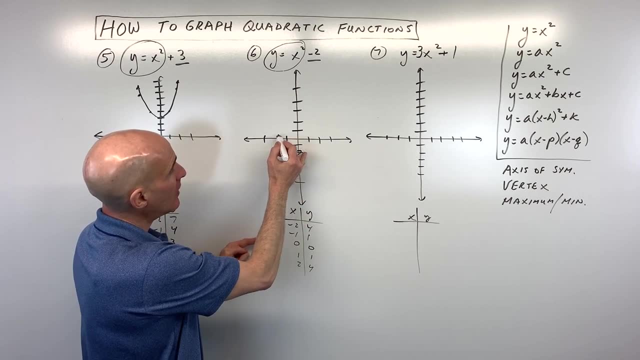 would be negative. two four, negative one a one zero, zero. one, one and two, four. It's just that I'm going to plot these points from here now. So I'm going left two up four. left one up one, zero, zero. 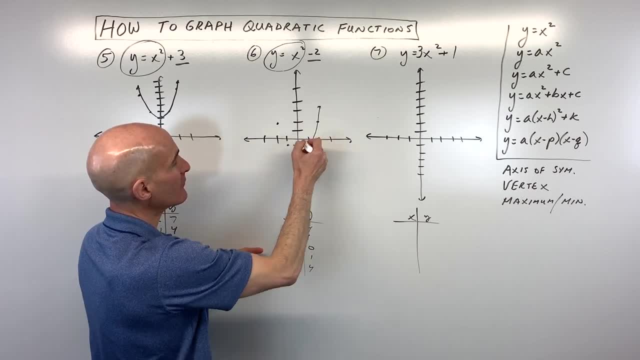 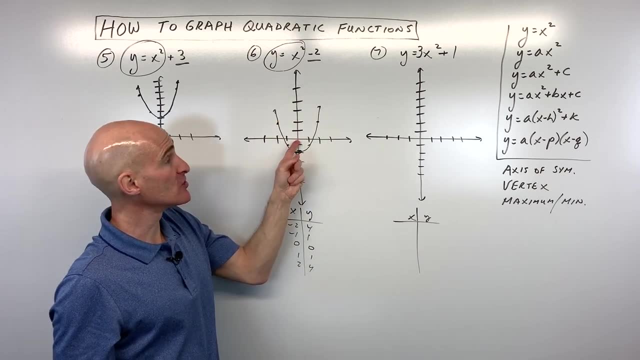 right one up one and right two up four. Now you don't have to do it this way. If you don't feel comfortable you can use the whole equation. But just remember, when you use the whole equation you want to plot from the zero, zero point that origin. If you just use the y, equals ax squared. 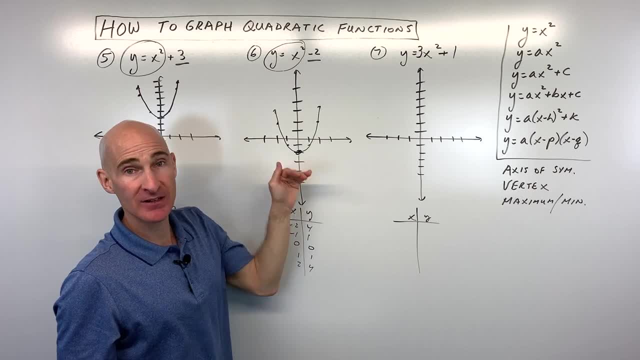 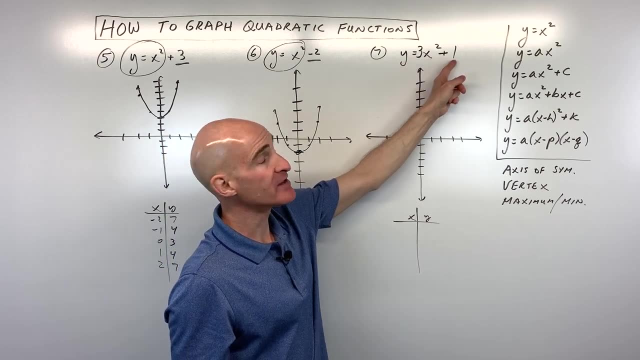 part of the equation. then you can graph from that shifted origin. okay, up or down? Okay, let's look at number seven. Okay, let's look at number seven. Okay, let's look at number seven. Okay, so we're putting together this a value three, with this c value one. So what do you think? 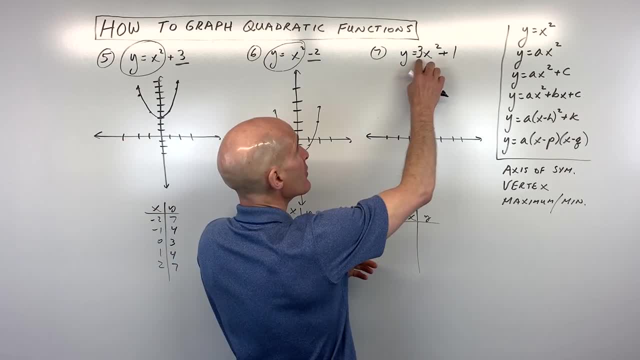 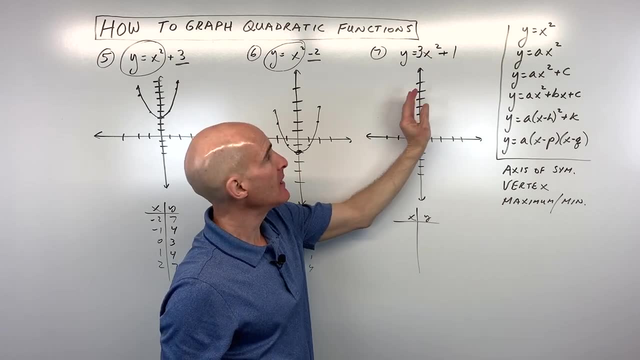 happens here in this problem. Well, the three is going to be a vertical stretch, And we know that when it's a stretch like that, it's going to make the graph look narrower because it's going up faster, right, But the plus one is going to shift it up one, Okay. so again, you can use the whole. 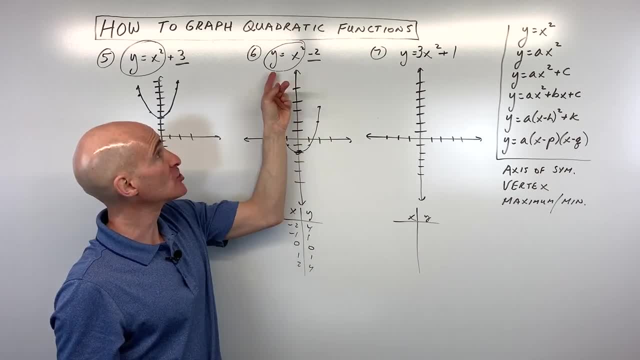 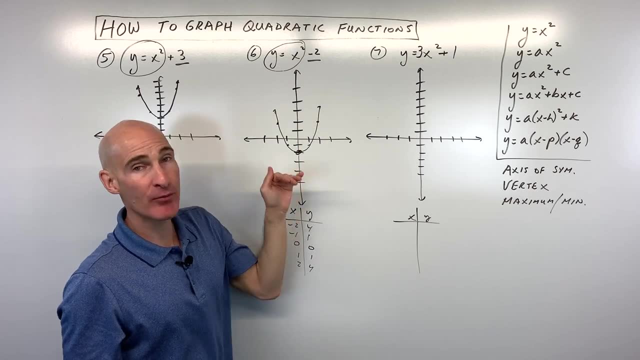 you want to plot from the 0,, 0 point that origin. If you just use the y equals ax, squared part of the equation, then you can graph from that shifted origin. okay, up or down? Okay, let's look at. 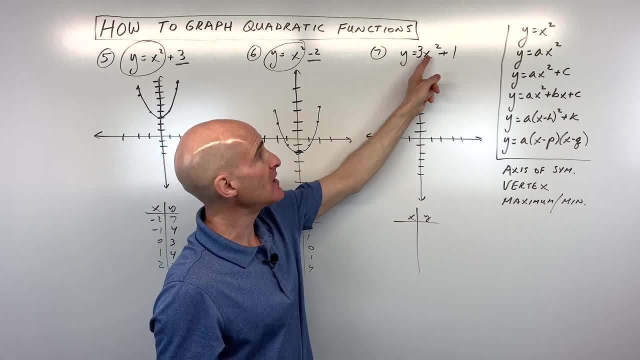 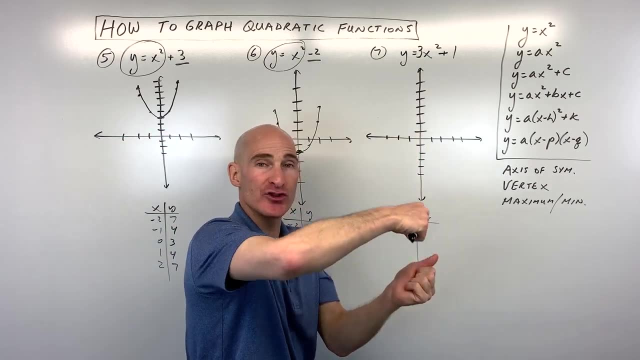 number 7.. Now we're putting together this- a value 3, with this c value 1.. So what do you think happens here in this problem? Well, the 3 is going to be a vertical stretch, And we know that when it's a. 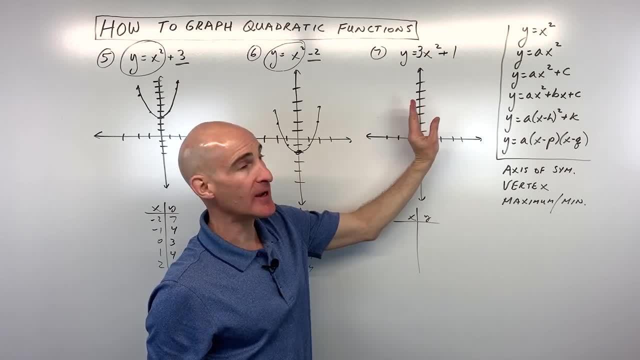 stretch like that. it's going to make the graph look narrower because it's going up faster, right? But the plus 1 is going to shift it up 1.. Okay, so again, you can use the whole equation if you want. 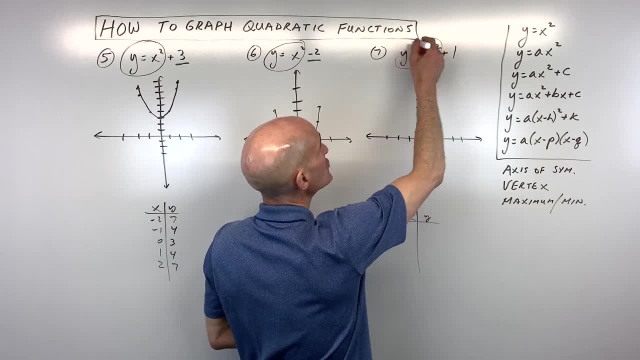 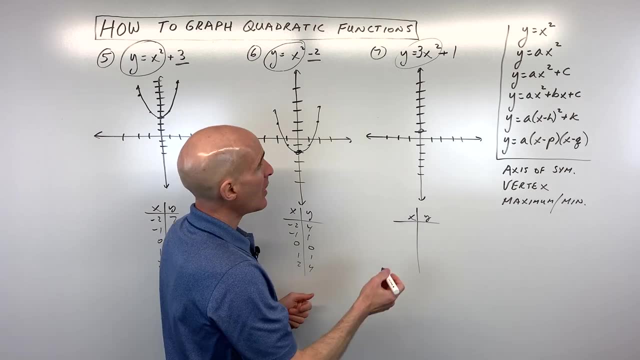 or you can do the little shortcut that I was showing. You could just use the y equals 3x squared and plot from here up 1.. Either way, you're going to get the same graph. So I'm going to use the whole equation this time. So I'm just going to put a negative 2,. 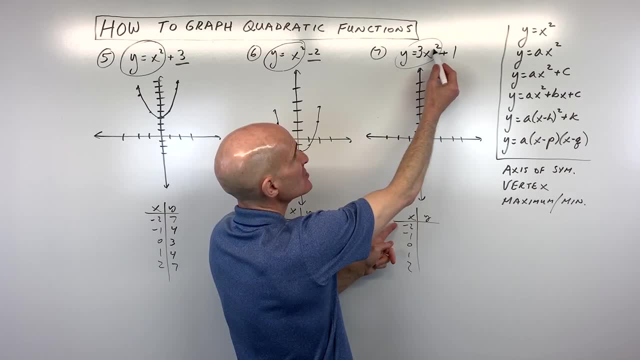 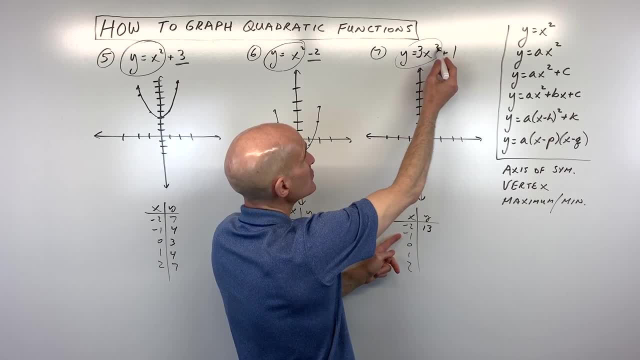 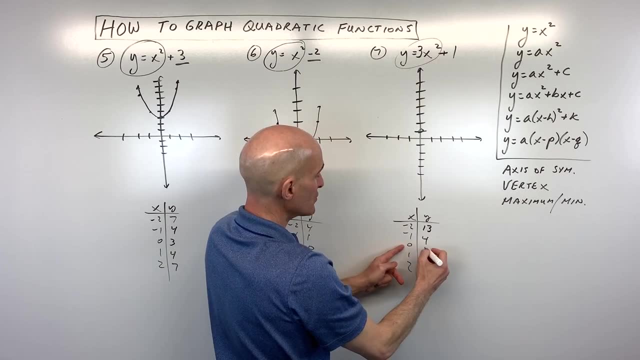 plus 1 is 13.. Negative: 1 squared is 1 times 3 is 3 plus 1 is 4.. 0 is going to give you 0 squared times 3 is 0 plus 1 is 1.. And then it's going to be the same on the other side, because it's. 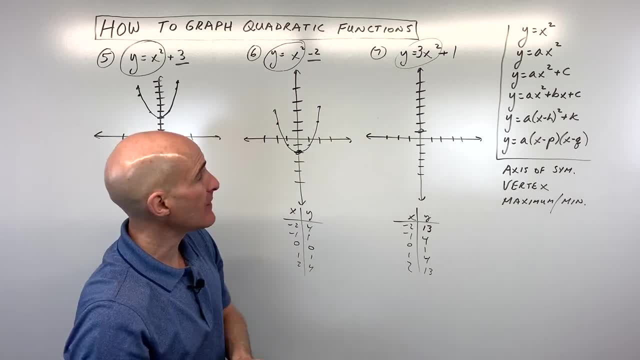 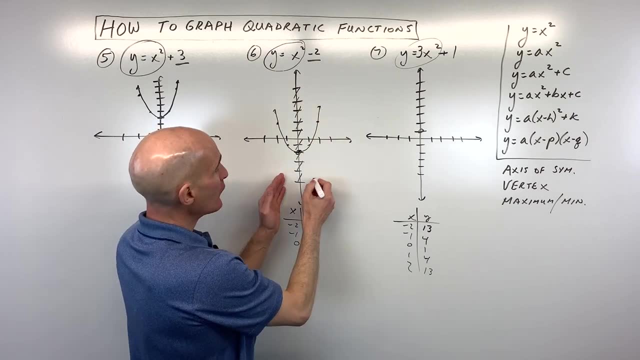 symmetric about this axis of symmetry. Now, sometimes what you can do when you draw this, you can draw it as kind of like a dashed or dotted line, that axis of symmetry. so far all the problems we've worked with that axis of symmetry is: x equals 0, right on the y axis. 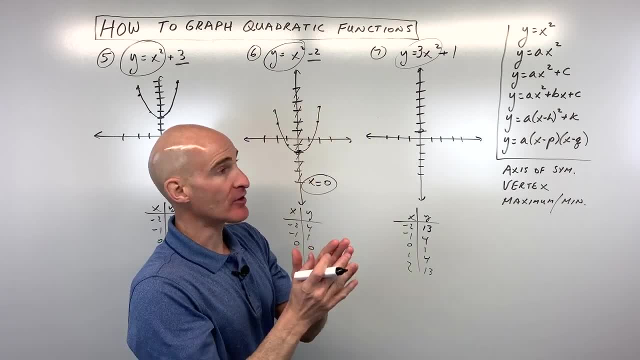 there. If you fold it over that line, it's going to match to itself. The graph is going to pair up like that. So now let's go ahead and graph this. So we've got negative 2, 13.. That's way off the. 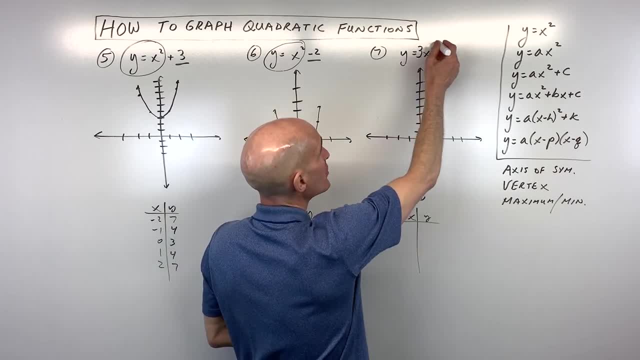 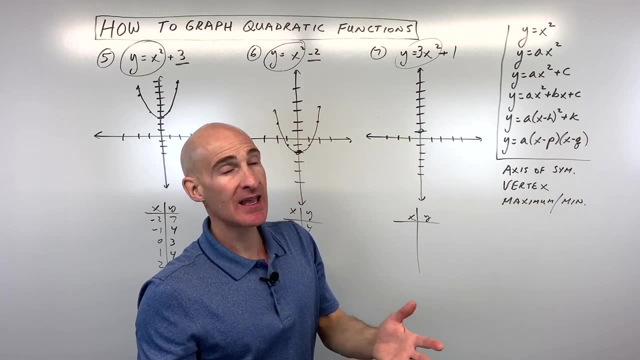 equation if you want, Or you can do the little shortcut that I was showing. you could just use the y equals three x squared and plot from here up one. Either way, you can do the whole equation this time. Okay, you're going to get the same graph, So I'm going to use the whole equation, this. 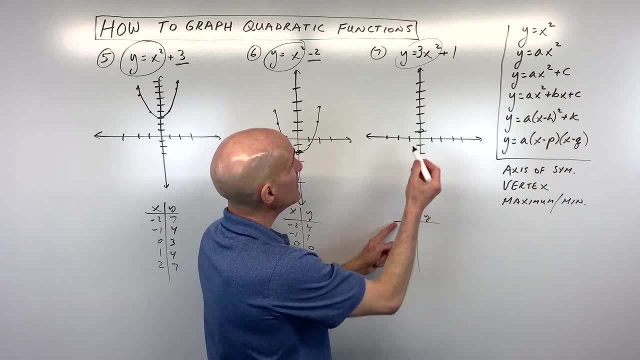 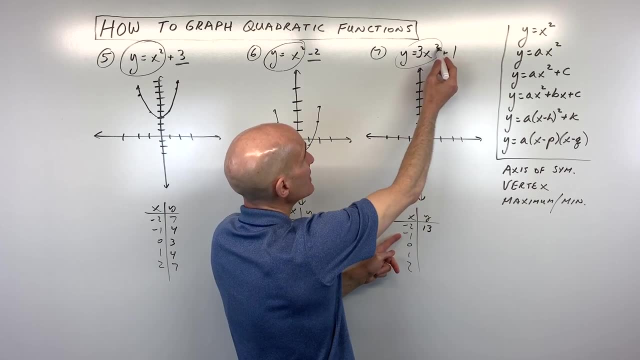 time. So I'm just going to put a negative two, negative one, zero, one and two. Remember the order of operations. negative two squared is four times three is 12 plus one is 13.. Negative one is negative. one squared is one times three is three plus one is four. Zero is going to give you zero. 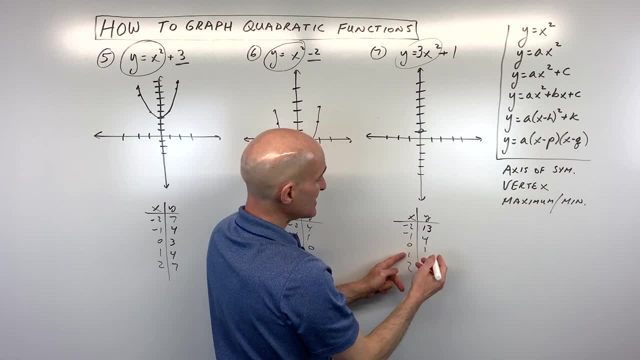 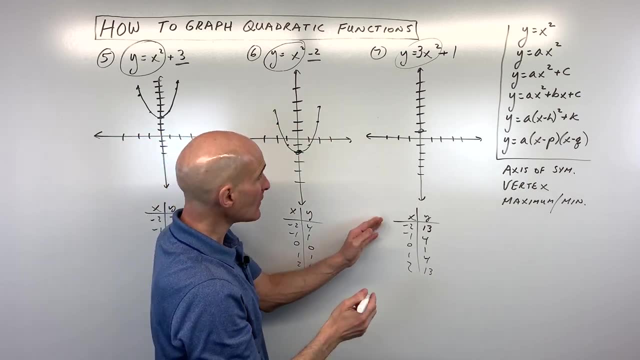 squared times three is zero plus one is one, And then it's going to be the same on the other side, Because it's symmetric about this axis of symmetry. Now, sometimes what you can do when you draw this, you can draw it as kind of like a dashed or dotted line. 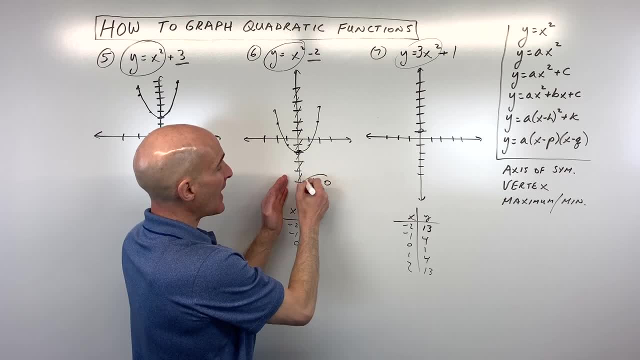 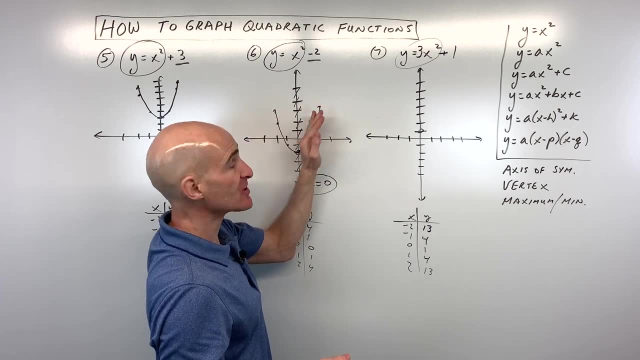 that axis of symmetry. So far all the problems we've worked with that axis of symmetry is: x equals zero, right on the y axis there, If you fold it over that line, it's going to match to itself. the graph is going to pair up like that. So now let's go ahead and graph this. So we've got. 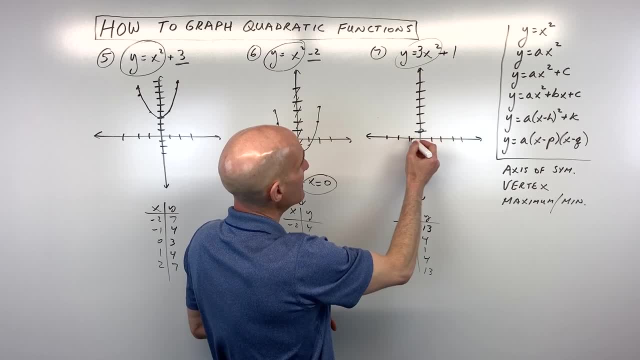 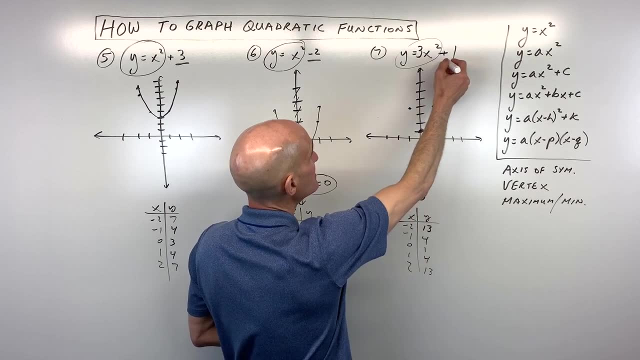 negative 213, that's way off the graph. negative one four, which is right here: zero one one: 213.. Now you're probably saying, Mario, why is it going way off the graph like that? Well, 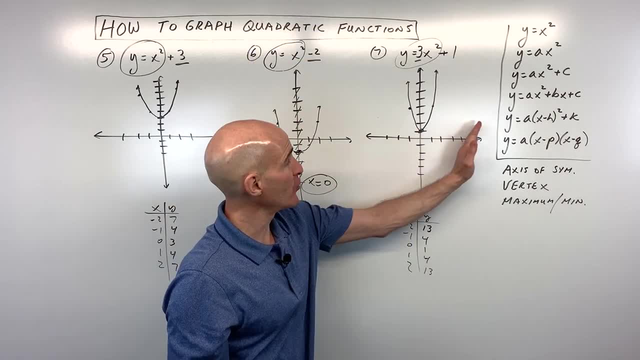 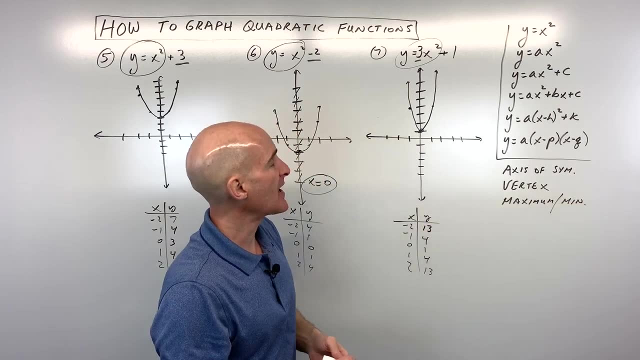 because, remember, the three is stretching it right, So the further you go out, it's going to go up really fast right Now. the one thing we haven't talked about yet is the maximum and the minimum. So what does that mean? maximum and minimum? Well, when the a value is positive, 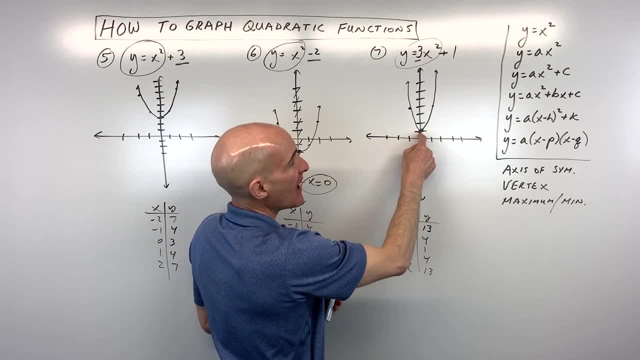 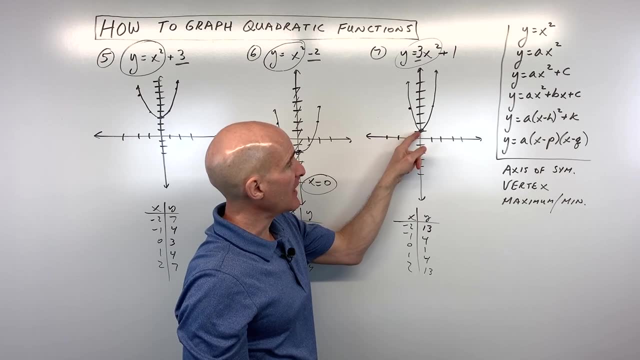 remember positive, smiling. it's opening up like this: you actually have a minimum, a low point, but you don't have a maximum. See how it keeps going up to infinity, forever and ever. So when it opens up a is positive, you have a minimum, you have a minimum, you have a minimum, you have a. 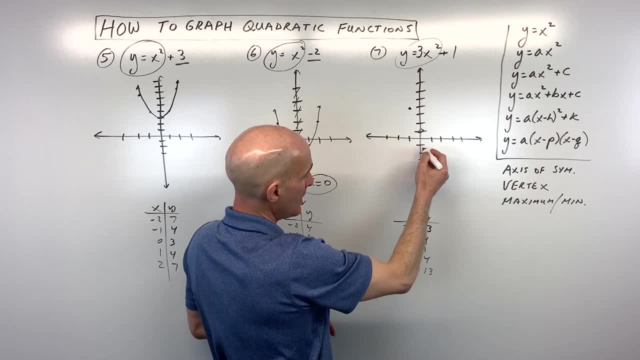 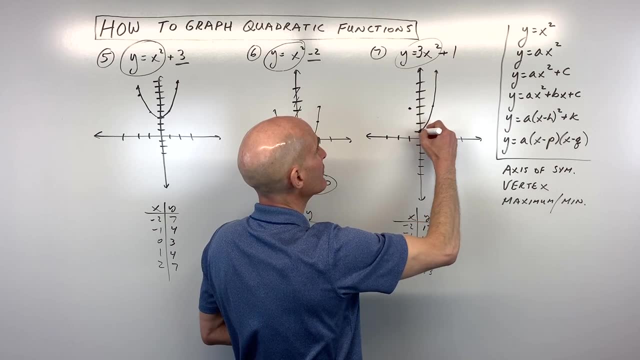 graph Negative: 1,, 4, which is right here? 0, 1,, 1,, 4,, 2, 13.. Now you're probably saying, Mario, why is it going way off the graph like that? Well, because, remember, the 3 is stretching. 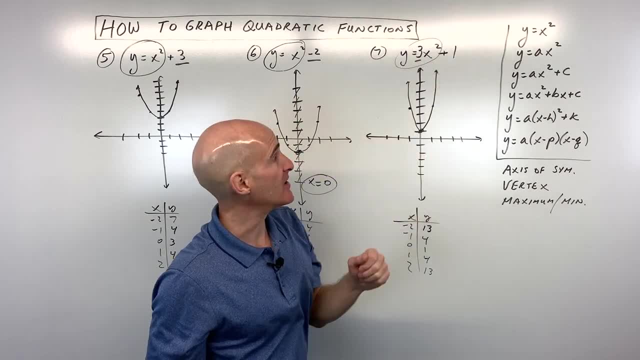 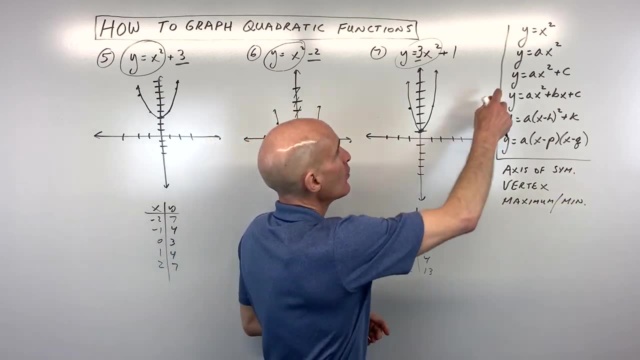 right. So the further you go out, it's going to go up really fast right Now. the one thing we haven't talked about yet is the maximum and the minimum. So what does that mean? maximum and minimum? Well, when the a value is positive- remember positive, smiling- it's opening up like 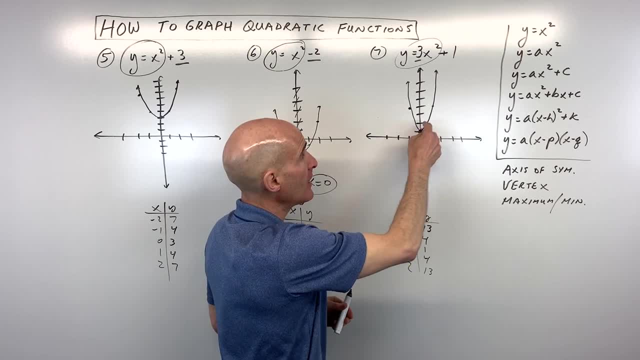 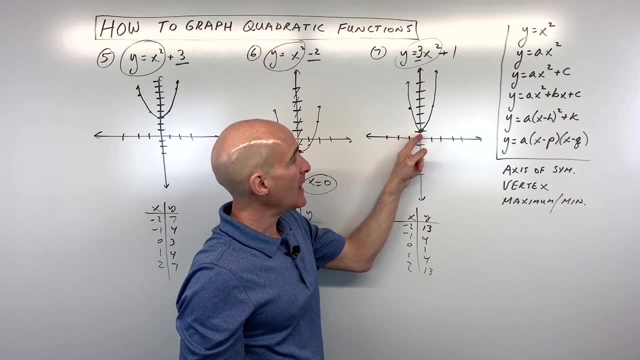 this. you actually have a minimum, a low point, but you don't have a maximum. See how it keeps going up to infinity, forever and ever. So, when it opens up, a is positive, you have a minimum. And what is the minimum value? meaning, what is the lowest that this graph goes to? Well, the lowest. 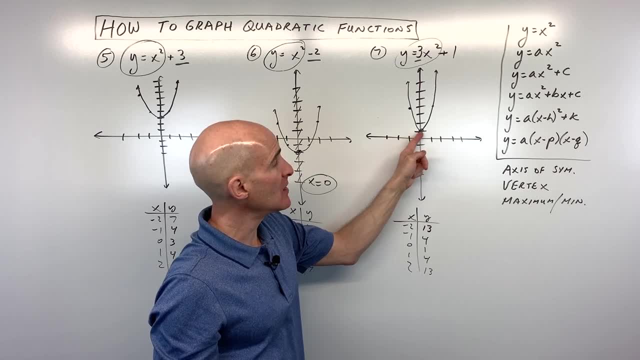 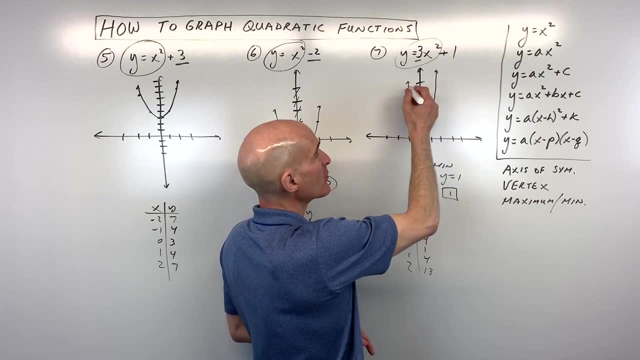 is going to be the y-coordinate here, okay- of this point, which is going to be y equals 1.. So in here, this case, the minimum is y equals 1, or you could just say 1.. This point where the graph bends. 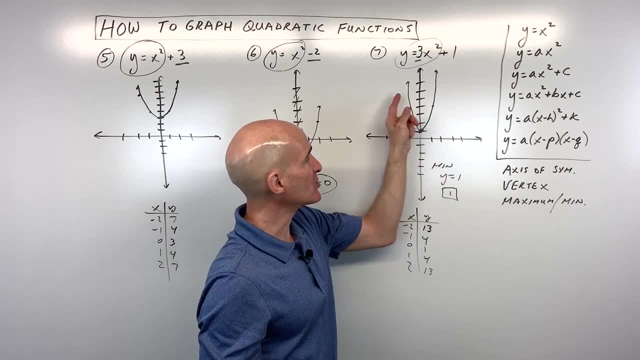 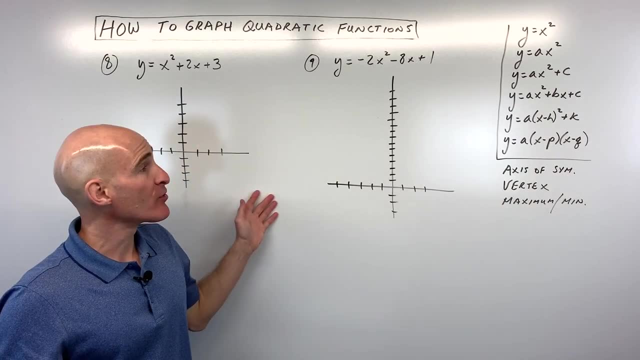 okay? we haven't talked about this yet. is the vertex okay? So this point where it's changing direction, it's going to be either the low point or the high point. with these parabolas, we call our vertex Okay, number 8 and number 9, we're going to be working with this standard form y. 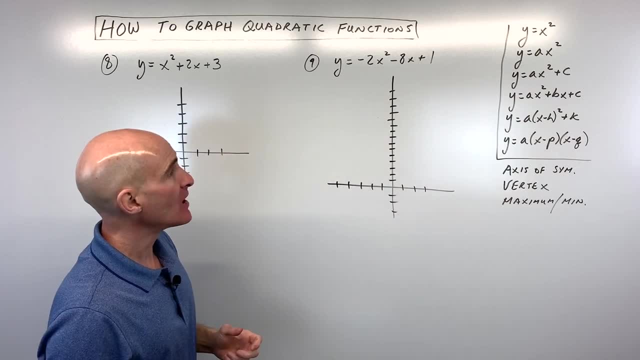 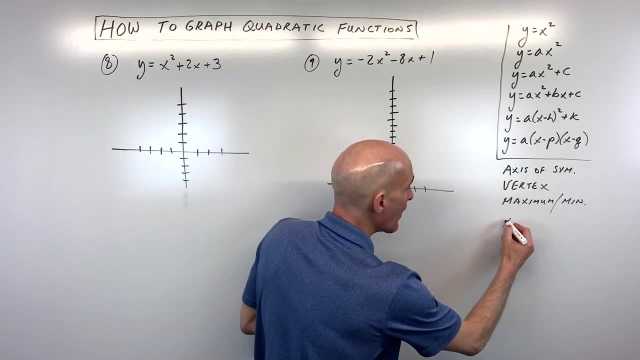 equals ax squared plus bx plus c. okay, of a quadratic. The question here now is how do we figure out where that vertex is? And we're going to introduce a formula here now: x equals the opposite of b, or negative b divided by 2 times a. Now remember: 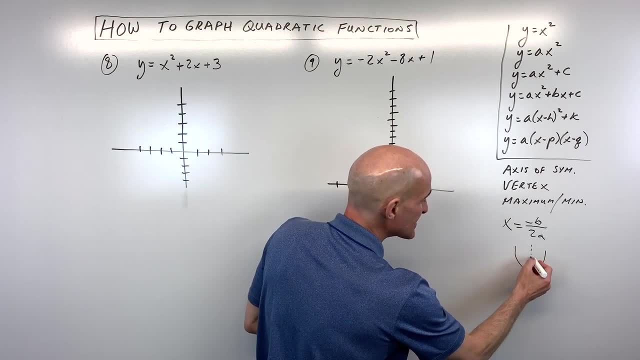 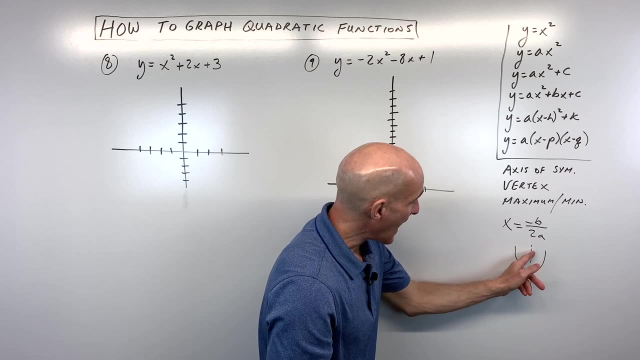 when you graph these parabolas, remember how they always have that symmetry and that line of symmetry. It divides the parabola in half. If you fold over that line, it matches to itself This axis of symmetry. the formula for that axis of symmetry will be: x equals negative b over 2a. 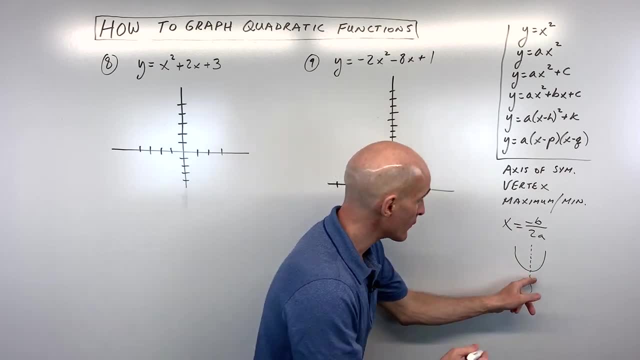 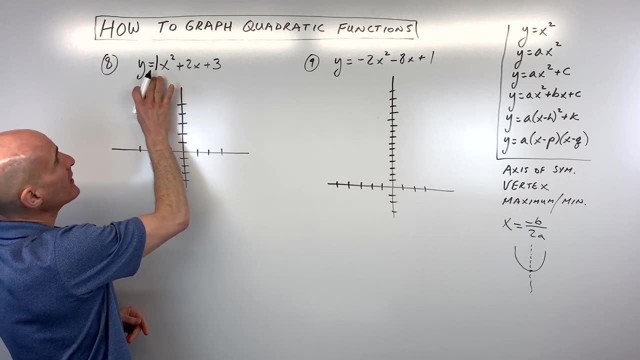 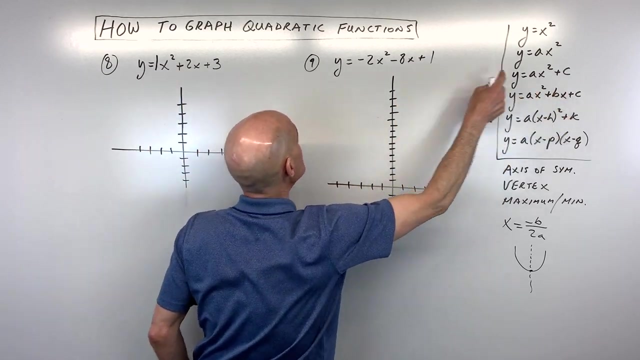 will also be the x coordinate of this vertex point right here. So let me show you how that works with number 8.. Notice that the a value here is 1, because 1x squared is the same as x squared. so a equals 1, b is equal to 2, see positive 2, and c is equal to 3.. So what we're going to do is: 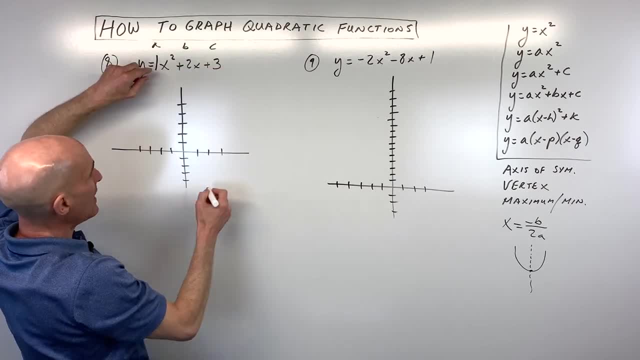 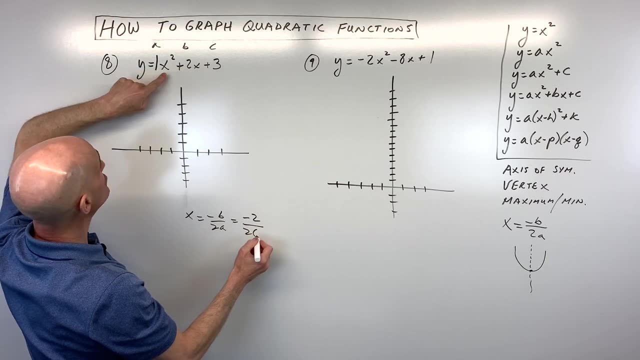 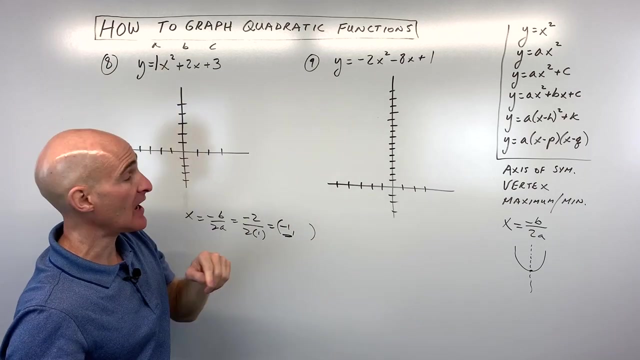 we're going to do. let's write it up here: a, b and c. so we have: x equals the opposite of b over 2a. so the opposite of b is going to be negative 2 over 2a. So negative 2 over 2 comes out to negative 1, that's the x coordinate of our vertex. 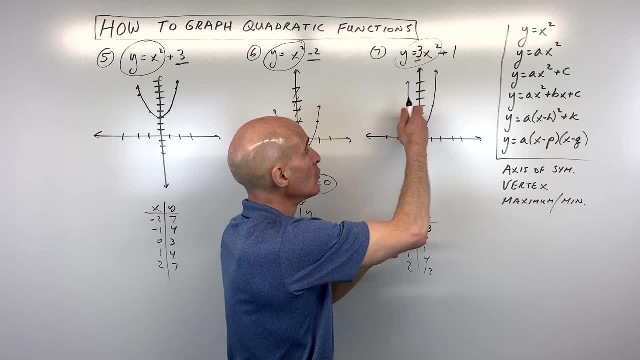 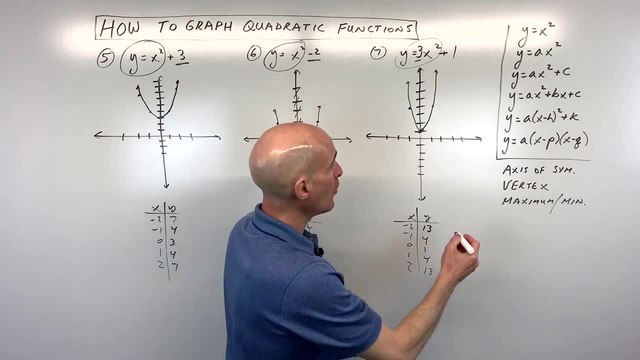 minimum. And what is the minimum value, Meaning what is the lowest that this graph goes to? Well, the lowest is going to be the y-coordinate here, okay, of this point, which is going to be y equals one. So in here, this case, the minimum is y equals one, or you could just say one, This point. 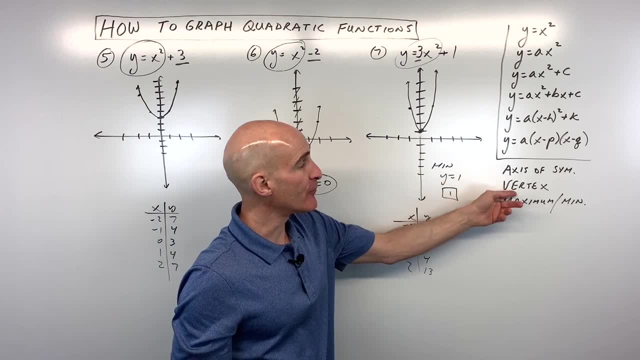 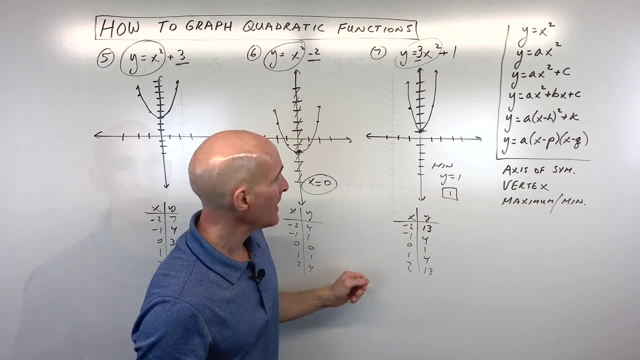 where the graph bends- okay, we haven't talked about this yet- is the vertex? okay? So this point where it's changing direction, it's going to be either the low point or the high point. with these parabolas, we call our vertex: Okay, number eight and number nine, we're going to be working. 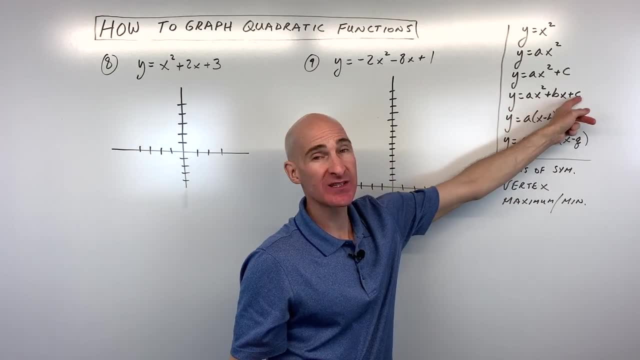 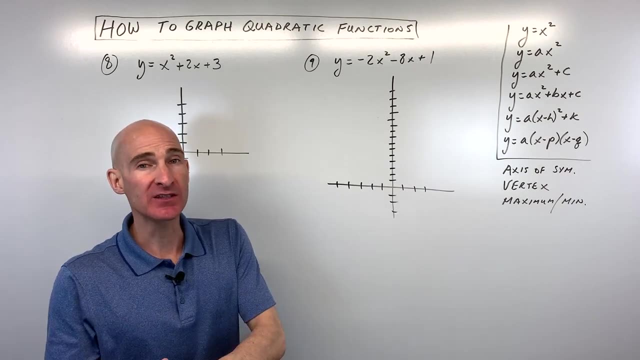 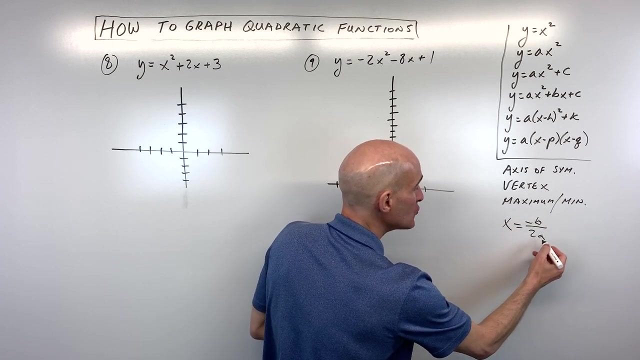 with this standard form, y equals ax squared plus bx plus c, okay, of a quadratic. And the question here now is: how do we figure out where that vertex is? And we're going to introduce a formula here now: x equals the opposite of b, or negative b divided by two times a. Now remember. 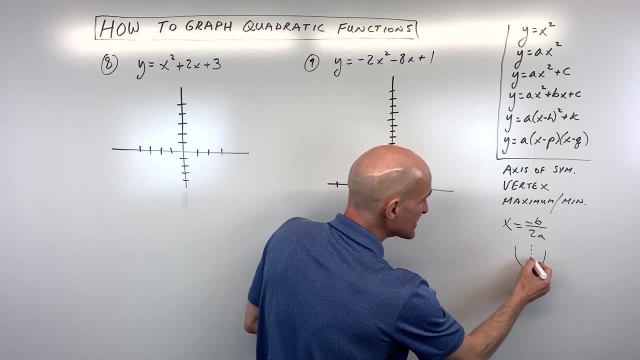 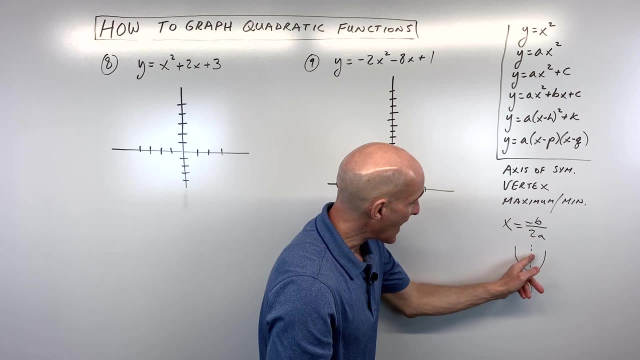 when you graph these parabolas, remember how they always have that symmetry and that line of symmetry divides the parabola in half. If you fold over that line, it matches to itself This axis symmetry. the formula for that axis of symmetry will be: x equals negative b over two a and the 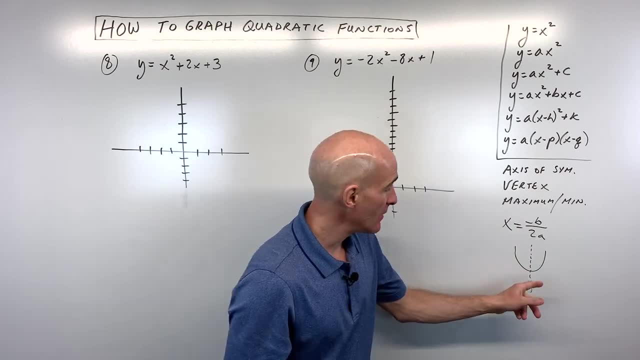 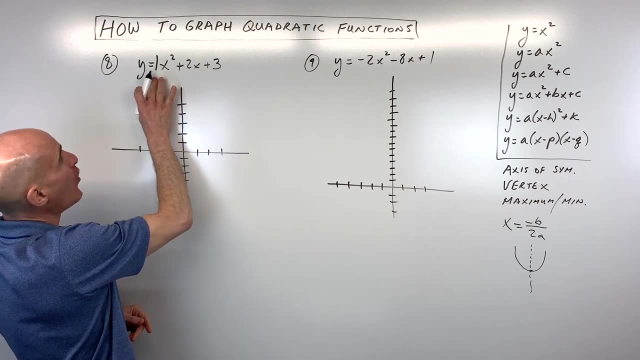 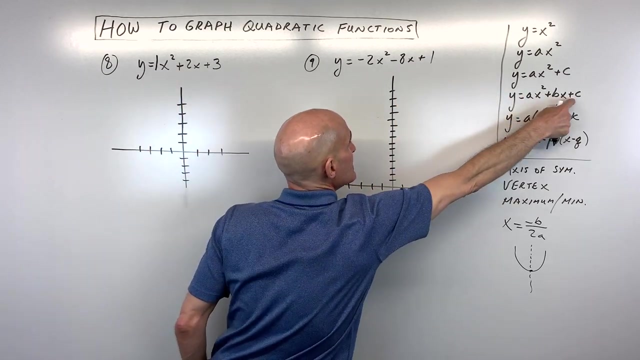 negative b over two. a will also be the x coordinate of this vertex point right here. So let me show you how that works with number eight. Notice that the a value here is one, because one x squared is the same as x squared, so a equals one, b is equal to two- see positive two- and c is equal to three. 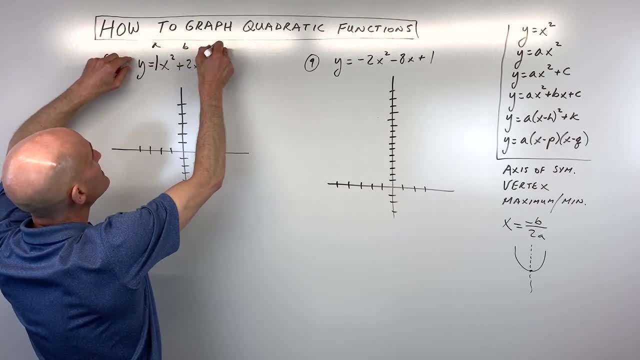 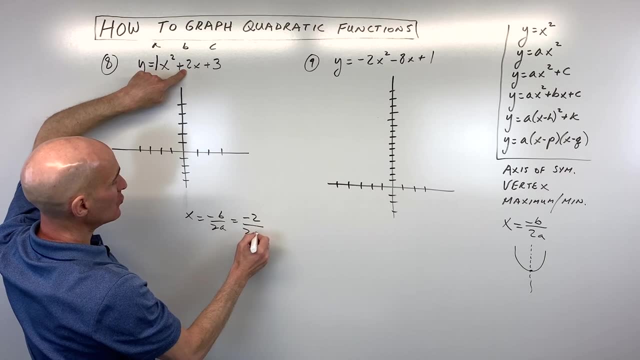 So what we're going to do is we're going to do- let's write it up here: a, b and c, So we have: x equals the opposite of b over two. a, so the opposite of b is going to be negative: two over two. 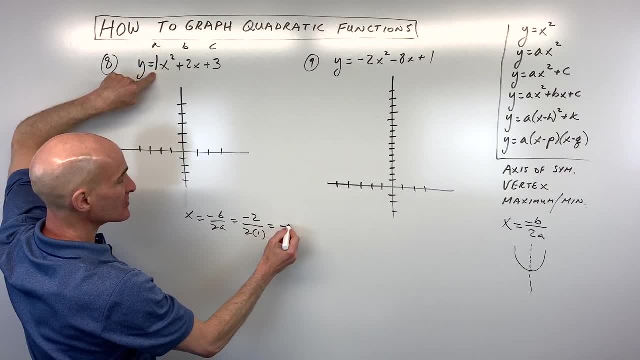 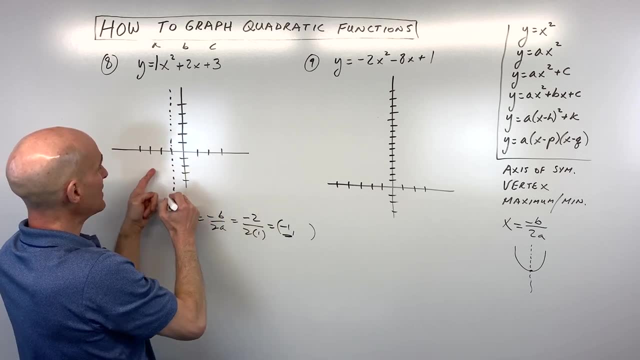 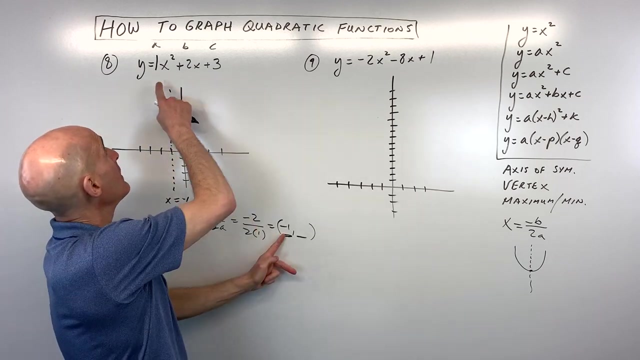 times one, So negative two over two comes out to negative one. that's the x coordinate of our vertex. It's also the line of symmetry right here. x equals negative one. Now how do we find the y coordinate of the vertex? We have to take this negative one, put it back in for x and that'll. 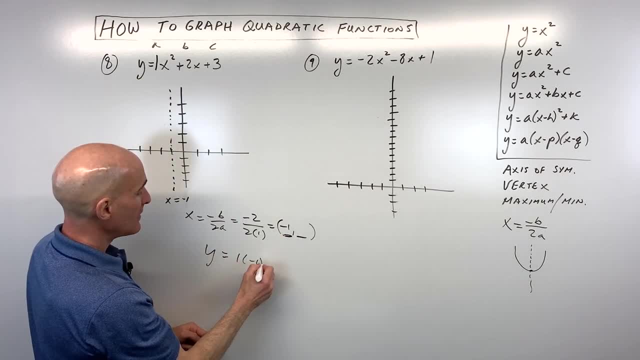 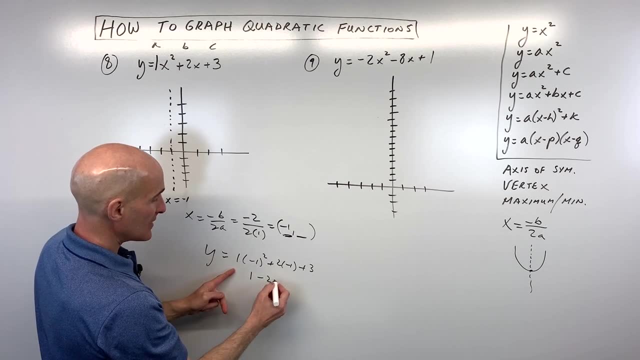 give us our y value. So let's go ahead and do that. We have y equals one times two, so that's negative one squared plus two times negative one plus three, So this comes out to one minus two plus three, which that's four minus two, which is two, So negative one. two is our vertex. Let's plot: 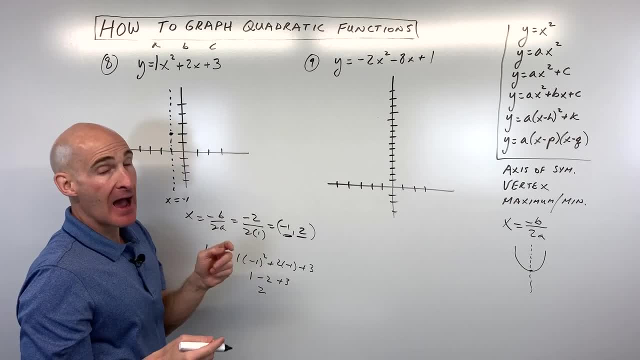 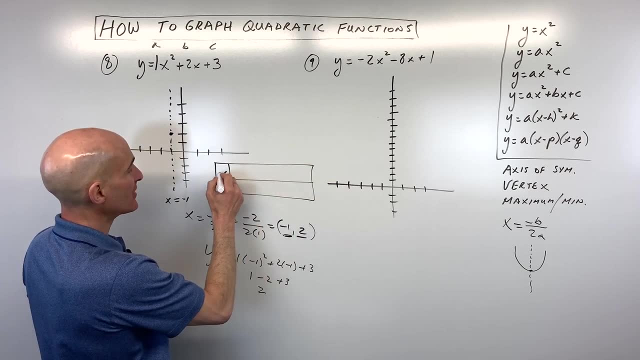 that on the graph, right here And now. what students like to do to get a good graph is sometimes they'll make a table like this- okay, kind of like a horizontal fashion, like this, And what they like to do is put the vertex in the middle. So you see, our vertex is negative one, two and the 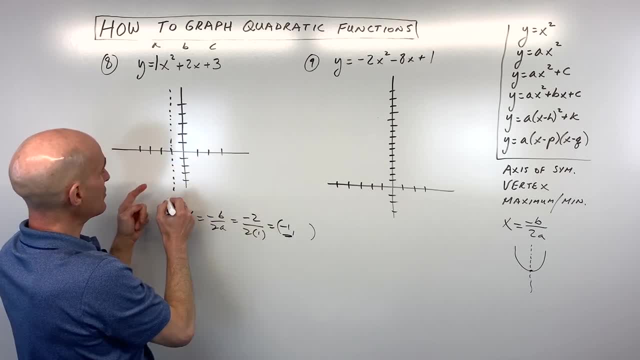 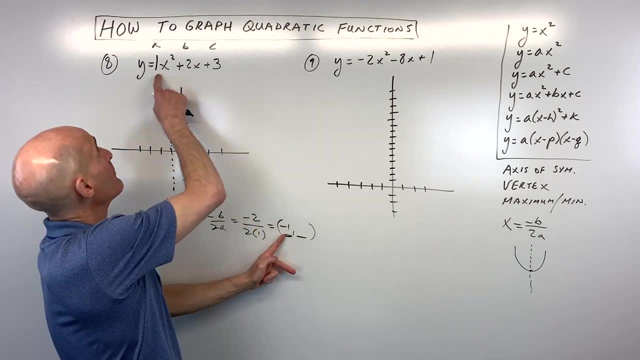 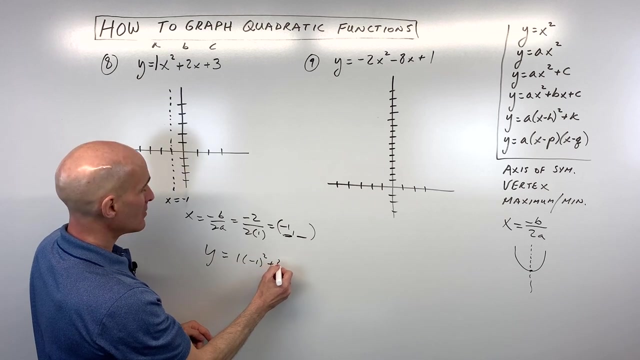 It's also the line of symmetry right here. x equals negative 1.. Now how do we find the y coordinate of the vertex? We have to take this negative 1, put it back in for x and that'll give us our y value. So let's go ahead and do that. We have y equals 1 times negative 1 squared. 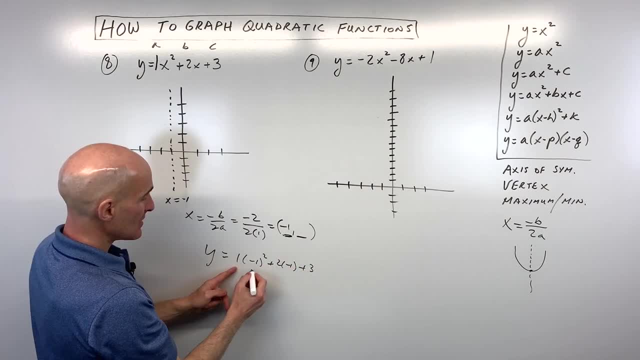 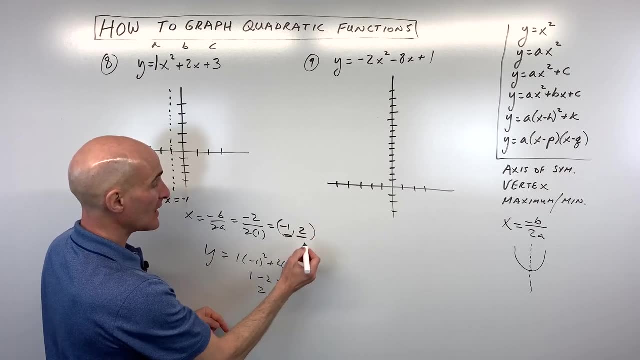 plus 2 times negative, 1, plus 3.. So this comes out to 1, minus 2, plus 3,, which that's 4, minus 2,, which is 2.. So negative 1, 2 is our vertex. 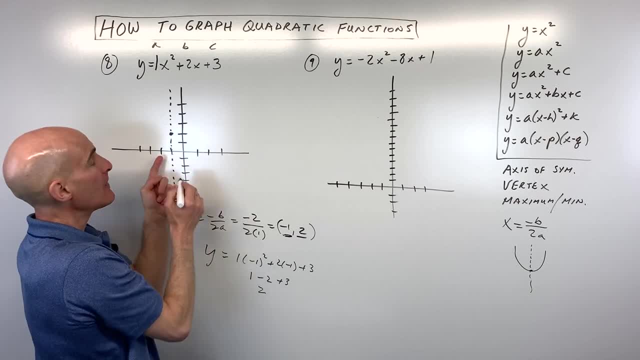 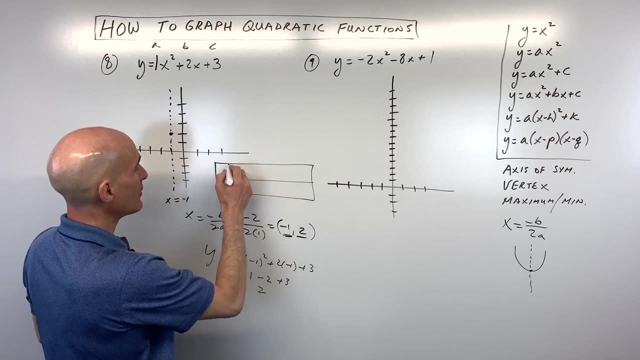 let's plot that on the graph right here And now. what students like to do to get a good graph is: sometimes they'll make a table like this- okay, kind of like a horizontal fashion, like this, and what they like to do is put the vertex in the middle. So you see, our vertex is negative. 1,, 2,. 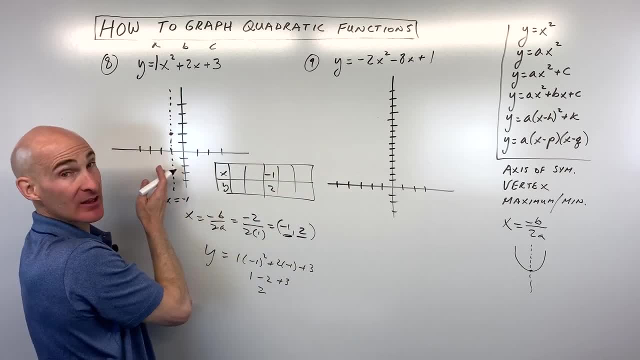 and then what we're going to do is we're going to pick some points on either side, okay, of this axis of symmetry, like negative 2, negative 3, 0,1.. So all I'm doing is I'm adding 1,. 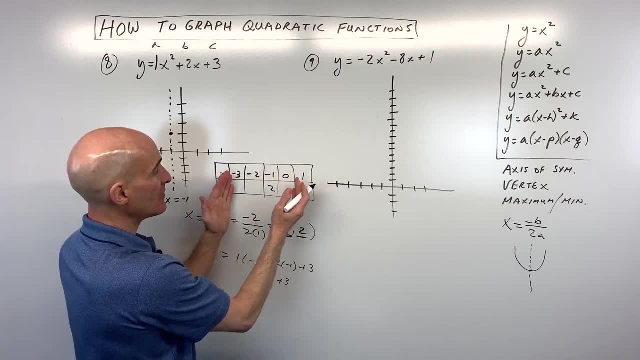 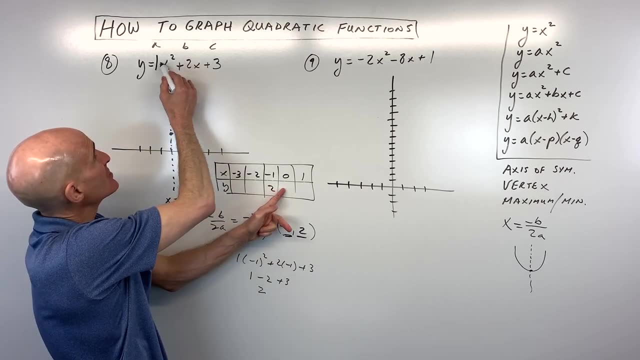 subtracting 1, or adding 2,, subtracting 2, and the idea is it's going to be the same on both sides of this line. So if I put 0 in 0, squared is 0 times 1 is 0,. 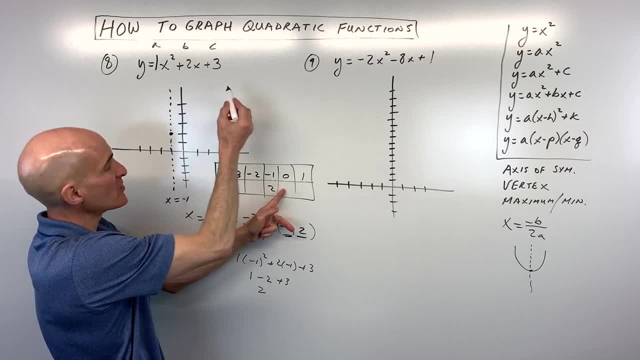 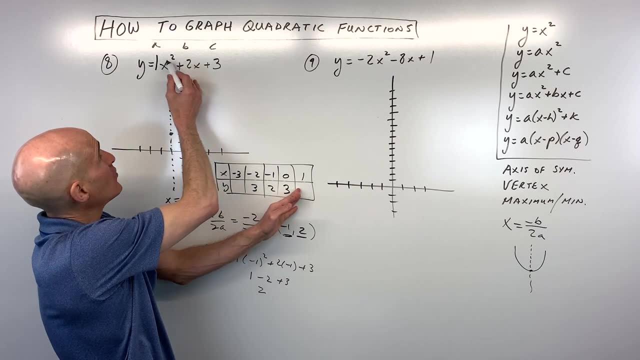 plus 3 times 0 is 0, so these all come out to 0, plus 3 more, that's 3, but then I also know that this one on the other side is also 3.. If I put 1 in, 1 squared is 1,. 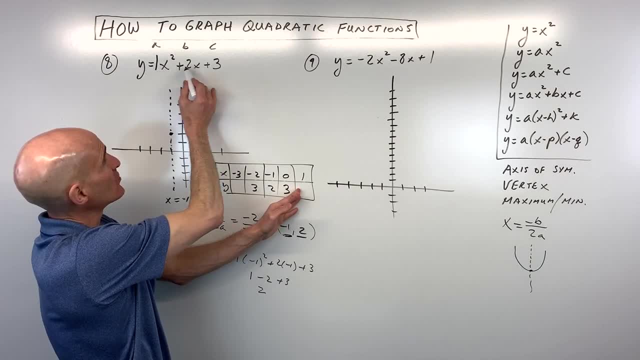 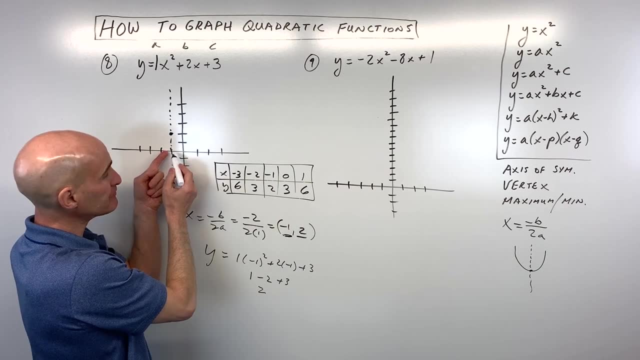 times 1 is 1, plus 2 times 1 is 2, plus 1 is 3, plus 3 is 6, this one here will also be 6.. It's the same on both sides. So let's go ahead and plot that We've got. 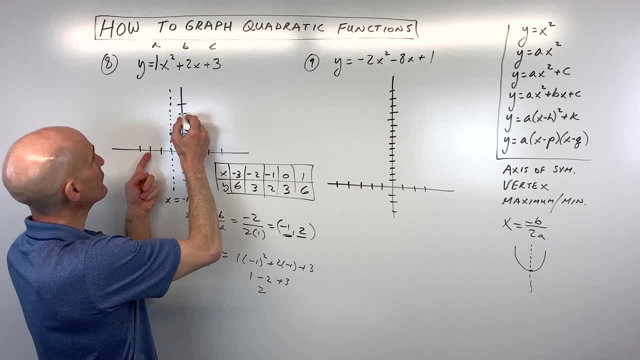 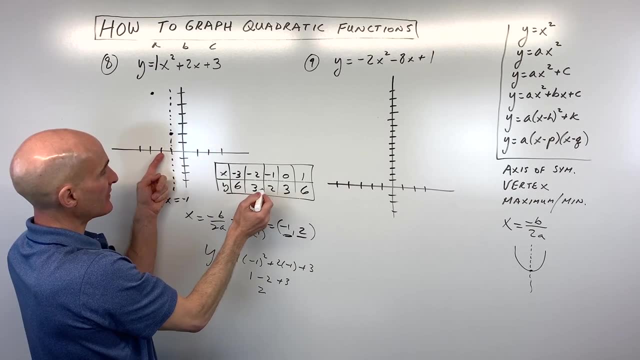 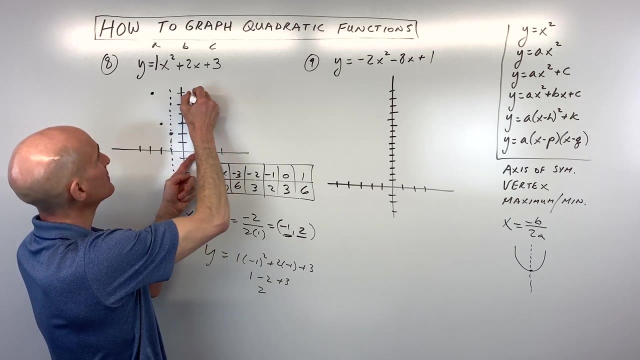 let's see negative 3, 6,, 1, 2, 3,, 4,, 5, 6, and we've got negative 1, 2, let's see I got that and negative 2, 3,, which is right there, and 0, 3, and 1, 6.. So there we go. 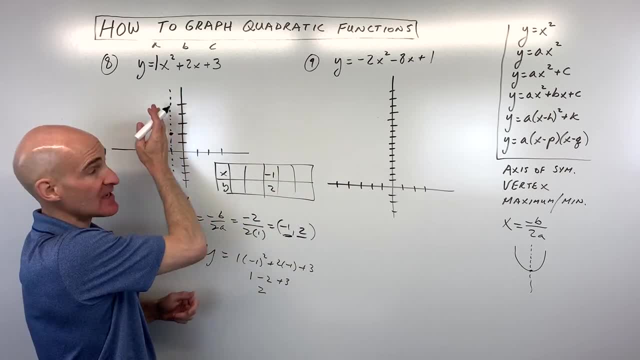 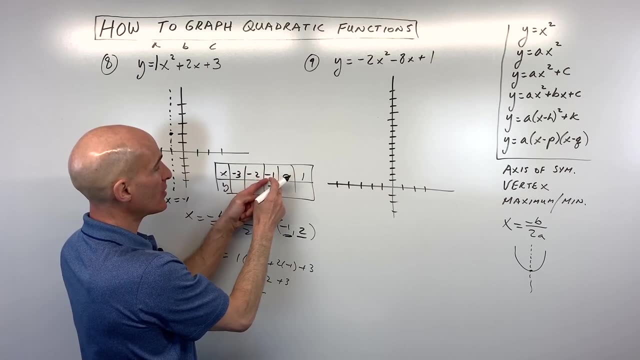 vertex is negative one, two, And what we're going to do is we're going to pick some points on either side, okay, of this axis of symmetry, like negative two, negative three, zero one. So all I'm doing is I'm adding one, subtracting one, or adding two subtracting two, And the idea is it's going to be: 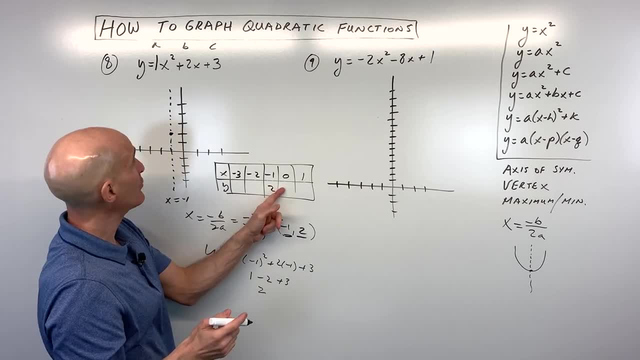 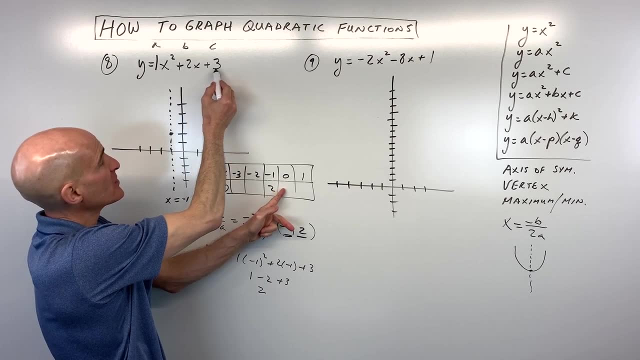 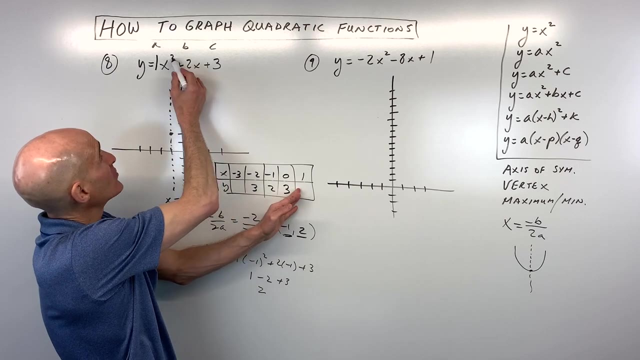 the same on both sides of this line. So if I put zero in zero, squared is zero times one is zero plus two times zero is zero. So these all came out to zero plus three more, that's three. But then I put one in one squared is one times one is one plus two times one is two plus one is three plus. 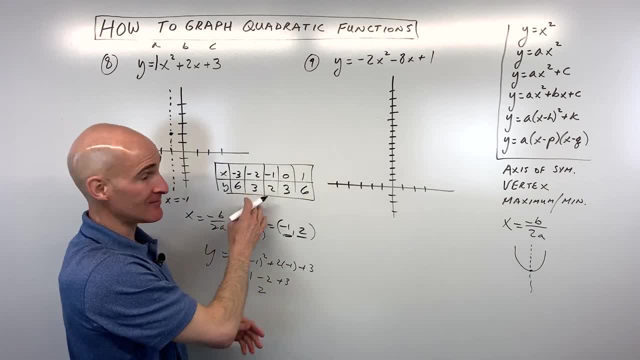 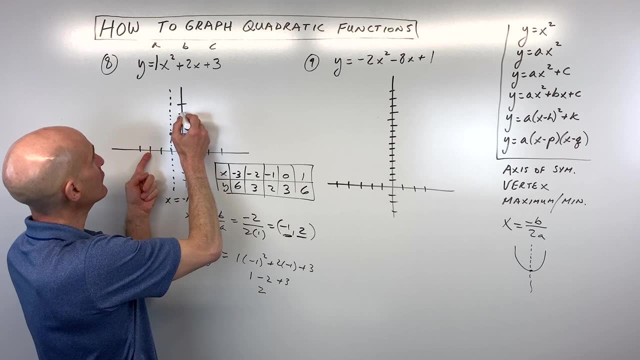 three is six. This one here will also be six. It's the same on both sides. So let's go ahead and plot that We've got. let's see negative three, six, one, two, three, four, five, six And we've got. 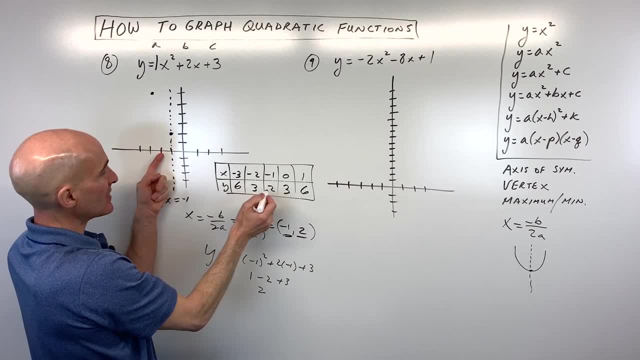 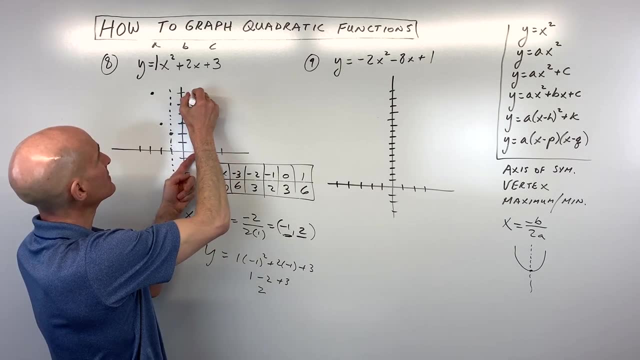 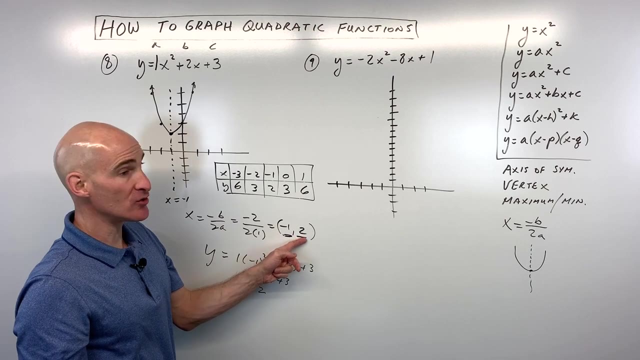 negative one, two- let's see, I got that- and negative two three, which is right there, and zero three and one six. So there we go, We've got our graph. This graph has a minimum. The minimum value is two. Let's see what. 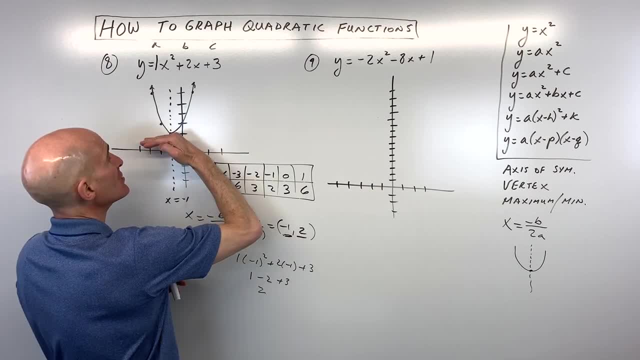 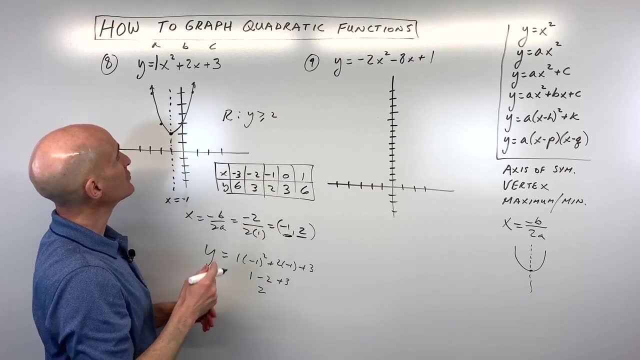 else we have. The domain is all real numbers. The range: what can y be? Well, y can be two or greater. So we would say our range is: y is greater than or equal to two. Domain is all real numbers, we said. 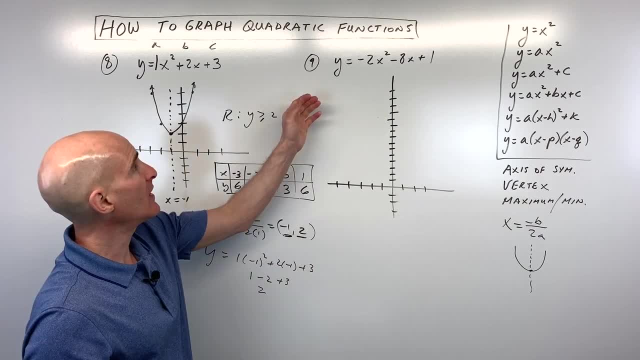 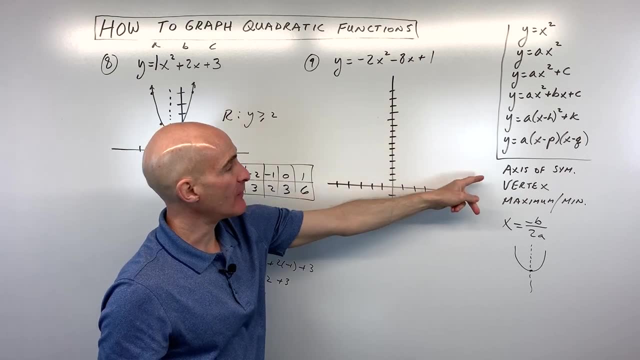 And that's it. So you've got a good graph. So now let's jump over to number nine. Same idea. we have: y equals ax squared plus bx plus c. Okay, but we need to find that vertex using our formula: negative b over 2a. Notice: the a value is 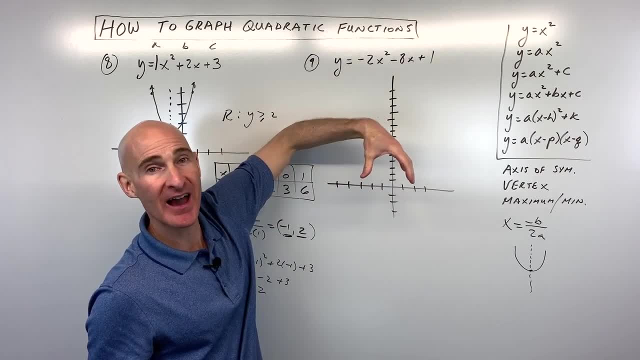 negative. What does that tell us? The parabola is going to open down like that. Okay, so let's go ahead and do this. We've got. this is a here, b here and c here. Now make sure you capture that. 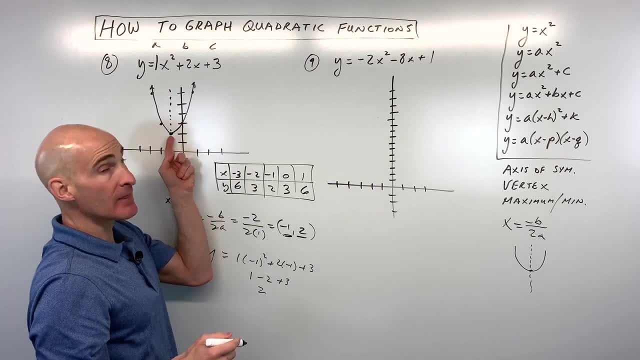 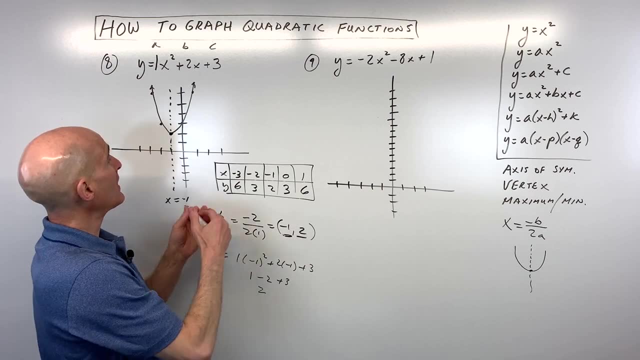 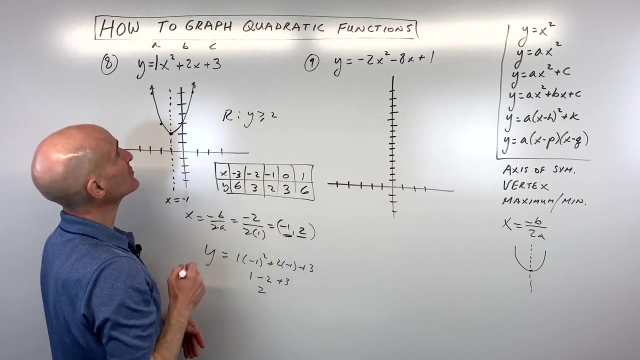 We've got our graph. This graph has a minimum. The minimum value is 2.. Let's see what else we have in the domain is all real numbers. The range: what can y be? Well, y can be 2 or greater. so we would say our range is: y is greater than or equal to 2.. Domain is all. 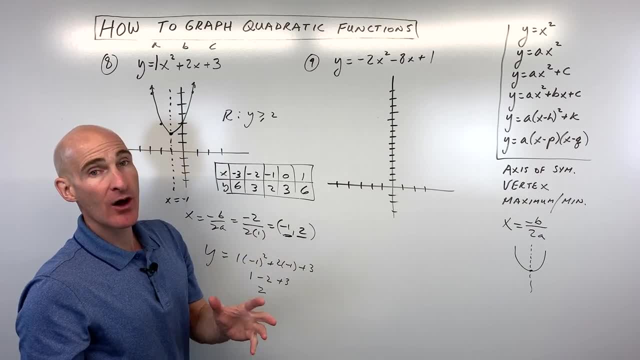 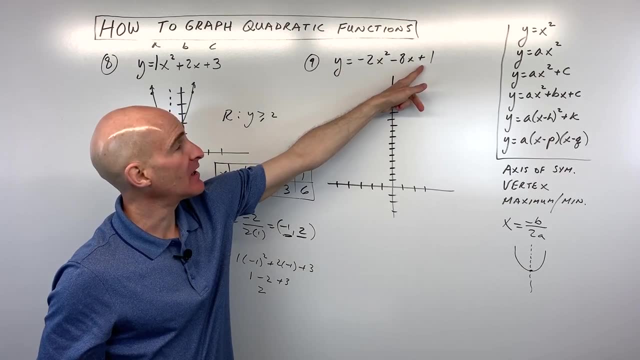 real numbers. we said: and that's it. So you've got a good graph. So now let's jump over to number 9.. Same idea we have. y equals ax squared plus bx plus c. okay, we need to find that vertex using our formula: negative b over 2a. Notice: the a value is: 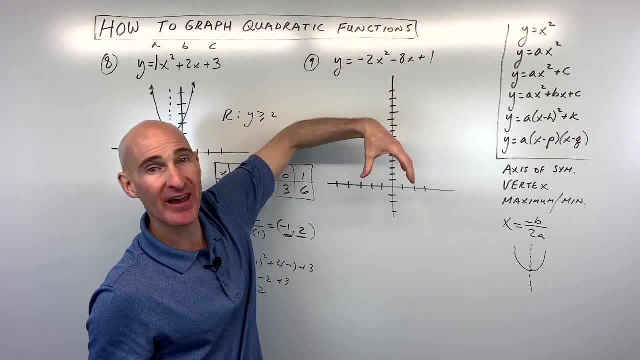 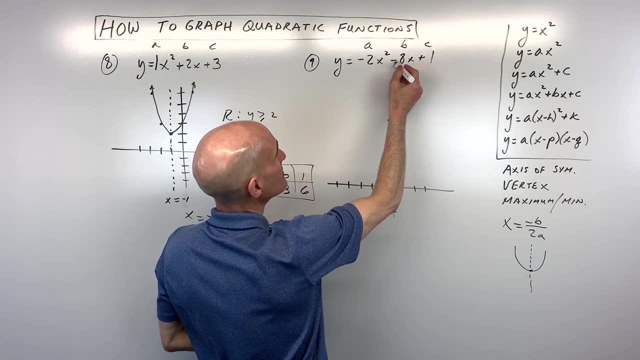 negative. what does that tell us? The parabola is going to open down like that, So let's go ahead and do this. We've got this is a here, b here and c here. Now make sure you capture that sign to the left or in front. So we have the opposite of negative 8, which 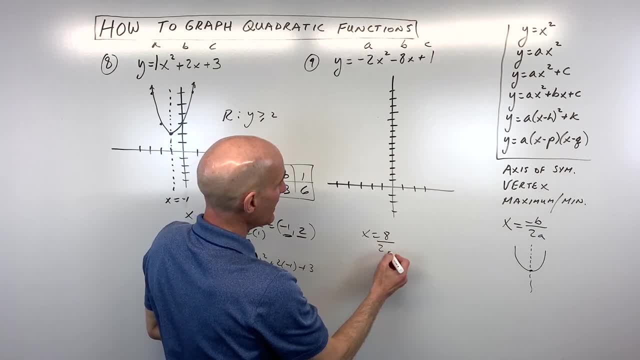 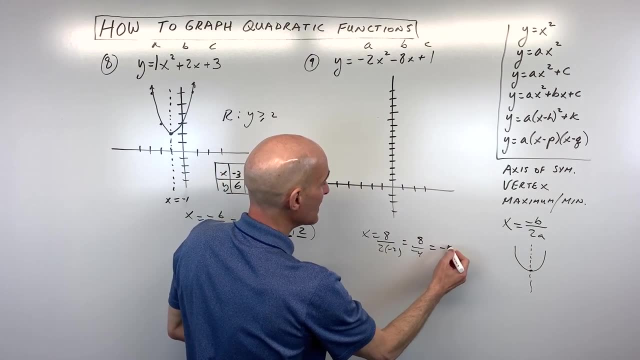 is positive 8, divided by 2 times a, which is 2 times negative 2.. So this becomes 8 over negative 4, which is negative 2.. So negative 2, that's the x coordinate of our vertex. 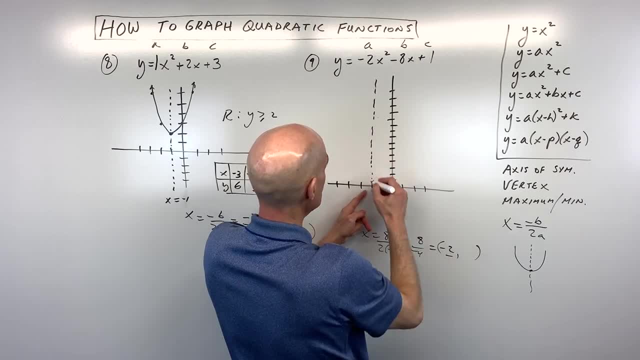 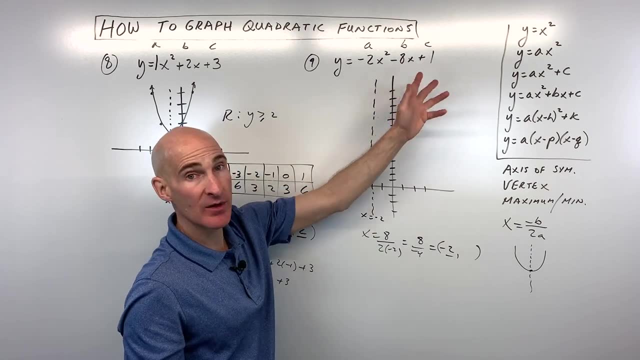 it's also the x equals negative. 2 is our axis of symmetry And if we want to find the y coordinate of the vertex, we have to take that negative 2 and put it back in. Now be careful: when you put it back in you do your order of operations. So negative 2 times negative. 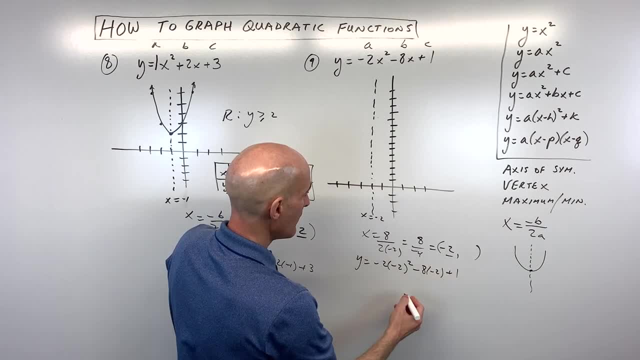 2 squared minus 8 times negative, 2 plus 1. So that's going to be 4 times negative. 2 is negative 8. These two negative 2's are negative 2.. These two negative 2's are negative 2.. 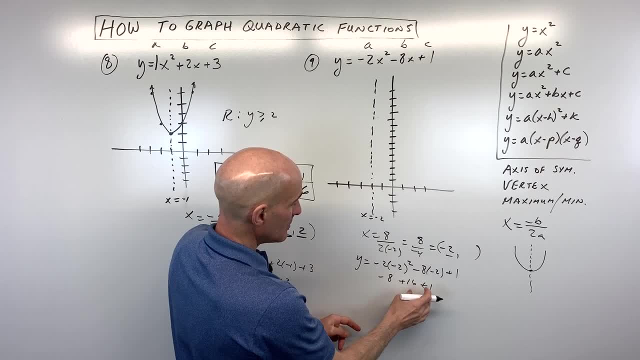 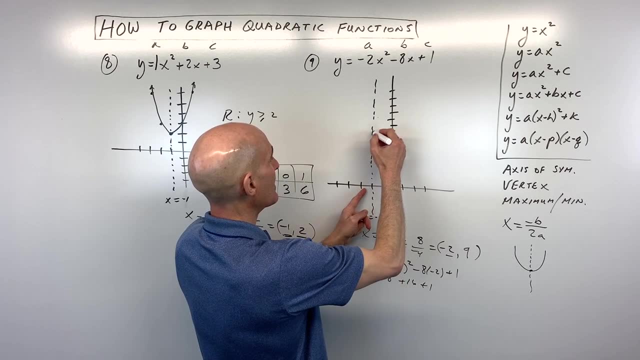 These two negative 2's give us positive 16. So we get 8 plus 1,, which is 9.. So our vertex is going to be: let's see: 1,, 2,, 3, 4, 5, 6,, 7,, 8, 9, right there, Okay. v for 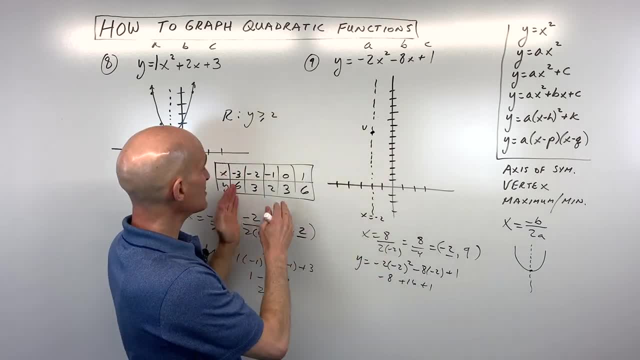 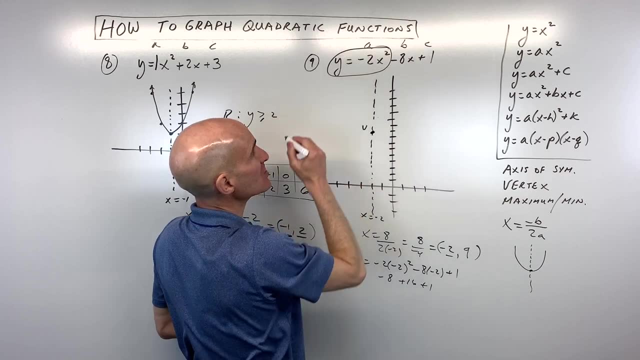 vertex, And now I'm going to show you another method here. You can do this table method, okay, but what you can also do is, once you find that vertex, you can focus in on the parent function. that y equals ax squared. That gives us the basic shape of the graph. 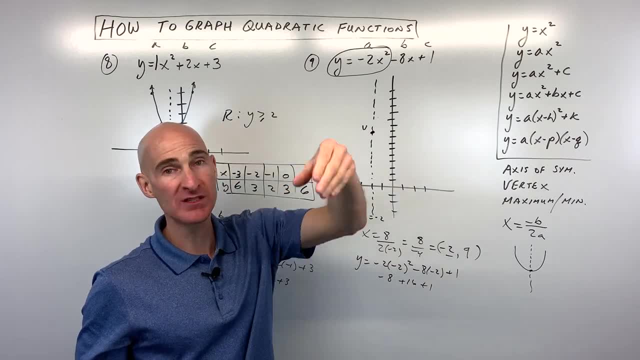 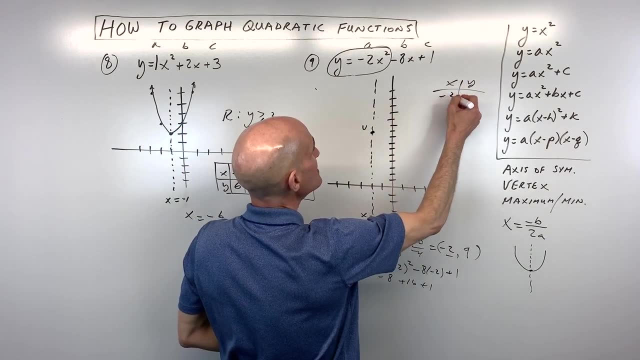 how wide it is or how narrow it is and whether it opens Up or opens down. So I'm just going to make a table on this part right here. Let's do it over here And let's pick just a couple easy values: negative 2, negative 1,, 0,, 1,. 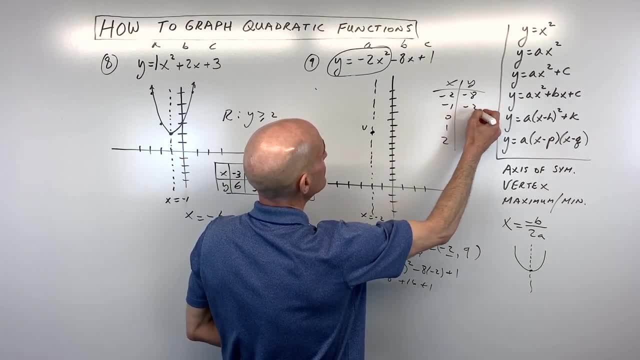 2. And this comes out to negative 8, negative 2, 0, negative 2, and negative 8.. And now what I'm going to do is I'm going to plot from this point. I'm going to pretend like 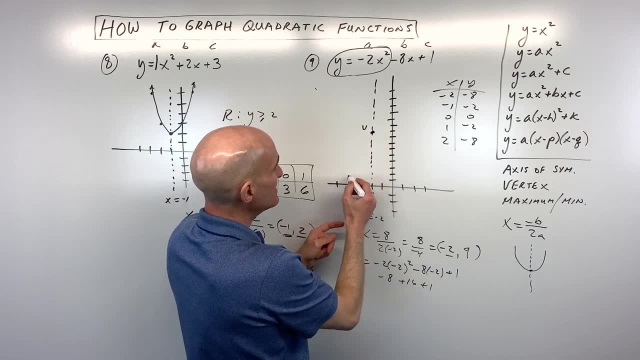 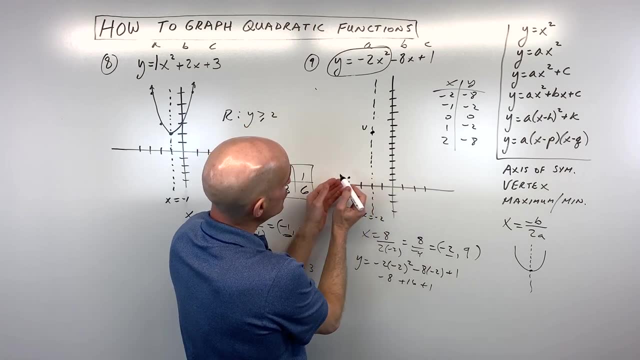 this is our origin. I'm going to go left 2, down 8,. okay, So let's see that would be right about here. And then the thing is, you can then reflect it over this line of symmetry. So see how I'm two units away If I go two units on the other side of the axis. 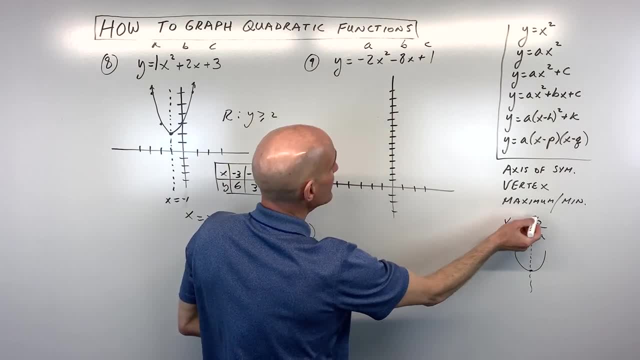 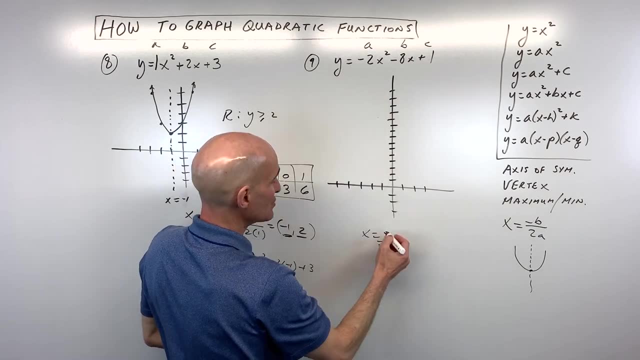 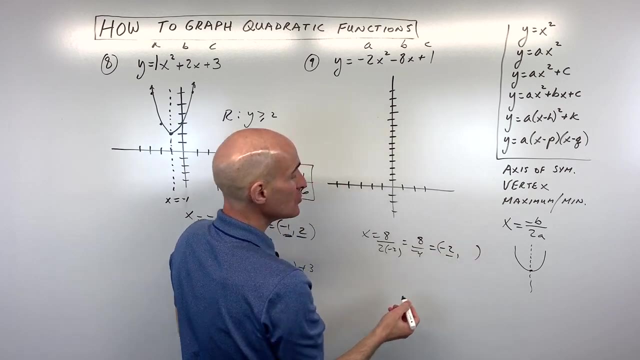 sign to the left or in front. So we have the opposite of negative eight, which is positive eight, divided by two times a, which is two times negative two. So this becomes eight over negative eight. So we have our negative four, which is negative two, So negative two. that's the x coordinate of our 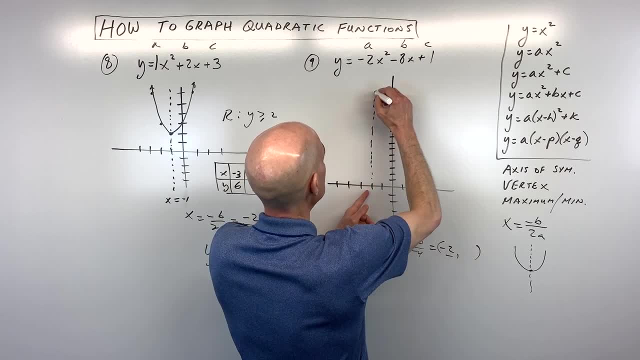 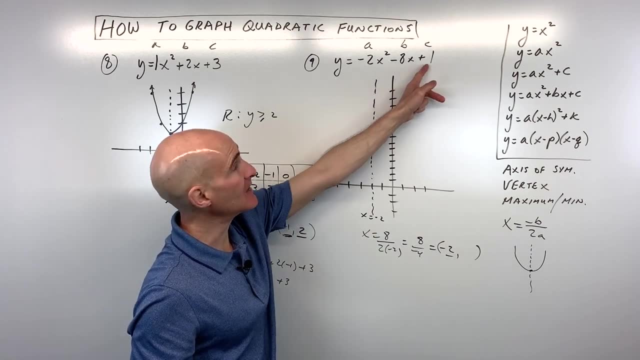 vertex. It's also the x equals negative two is our axis of symmetry And if we want to find the y coordinate of the vertex we have to take that negative two and put it back in. Now be careful: when you put it back in you do your order of operation So negative two times negative two. 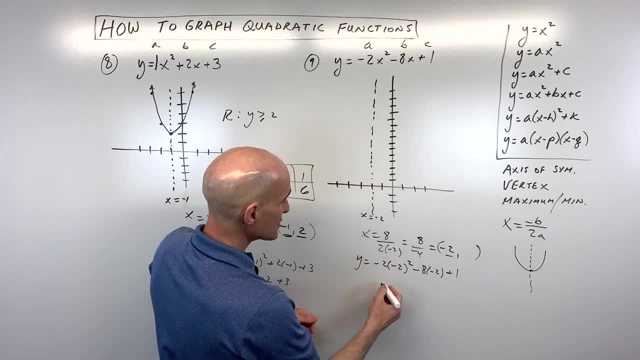 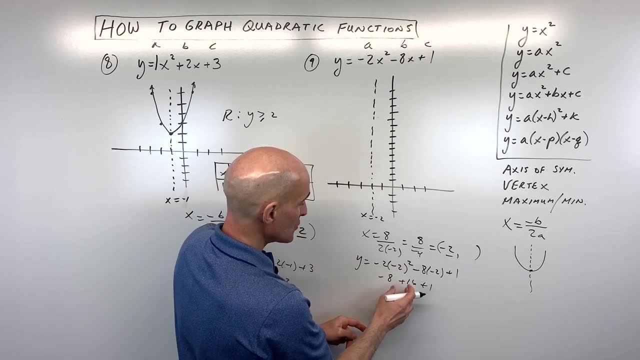 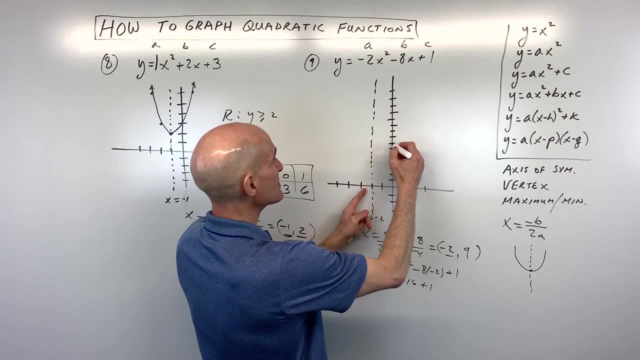 squared minus eight, times negative two plus one, So that's going to be four times negative. two is negative eight. These two negatives give us positive 16. So we get eight plus one, which is nine. So our vertex is going to be: let's see: one, two, three, four, five, six, seven, eight, nine. right there, Okay. v for. 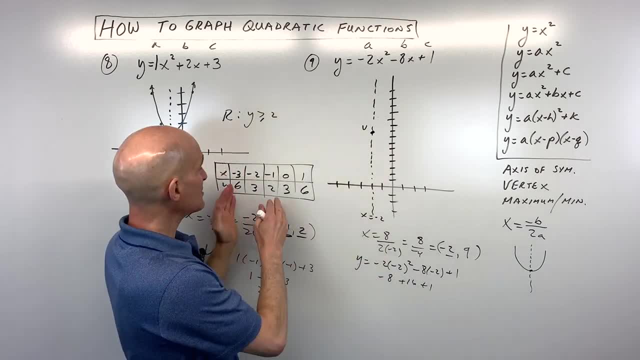 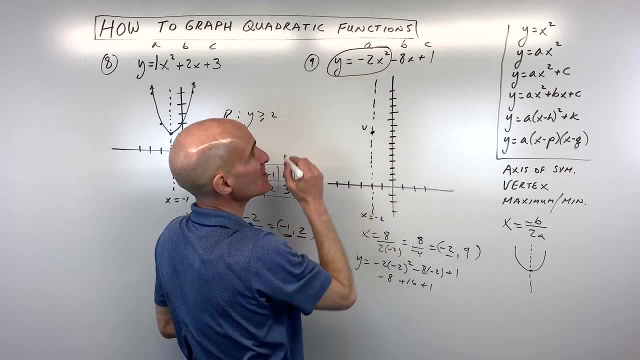 vertex, And now I'm going to show you another method here. You can do this table method, Okay, But what you can also do is, once you find that vertex, you can focus in on the parent function that y equals ax squared. That gives us the basic shape of the graph, how wide it is or how narrow it. 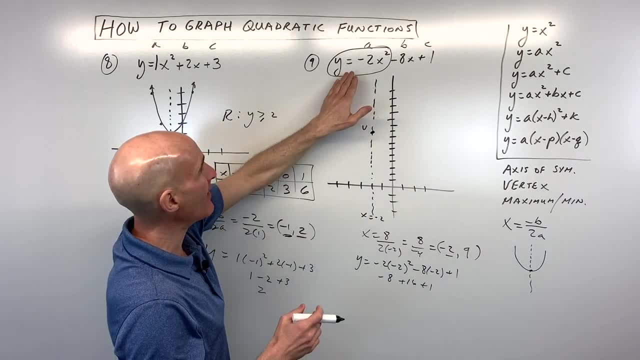 is, And then you can do this table method, And then you can do this table method, And then you can do this table method, And whether it opens up or opens down. So I'm just going to make a table on this part, right here. 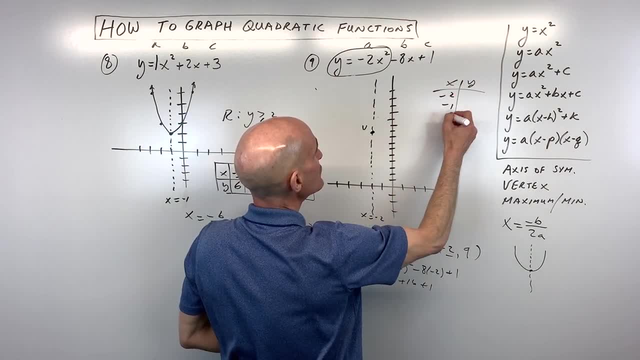 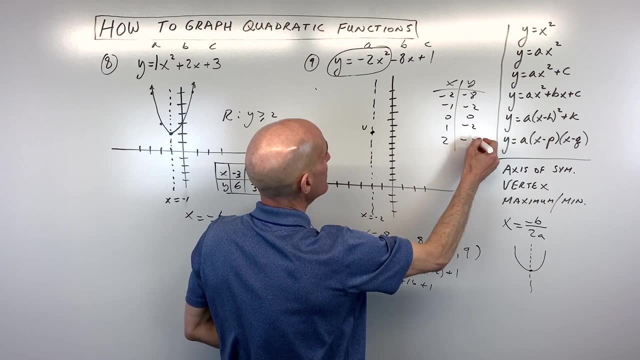 Let's do it over here And let's pick just a couple of easy values: negative two, negative one, zero one, two- And this comes out to negative eight, negative two, zero, negative two and negative eight. And now what I'm going to do is I'm going to plot from this point, I'm going to pretend like 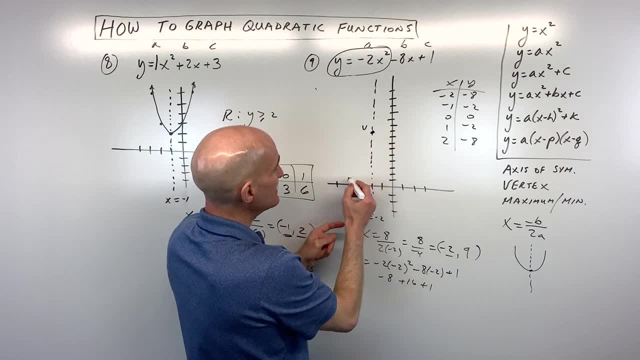 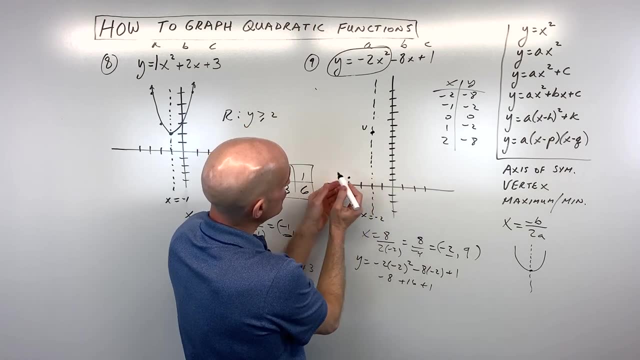 this is our origin. I'm going to go left two, down eight. Okay. So let's see, that would be right about here. And then the thing is, you can then reflect on that. So I'm going to go left two. 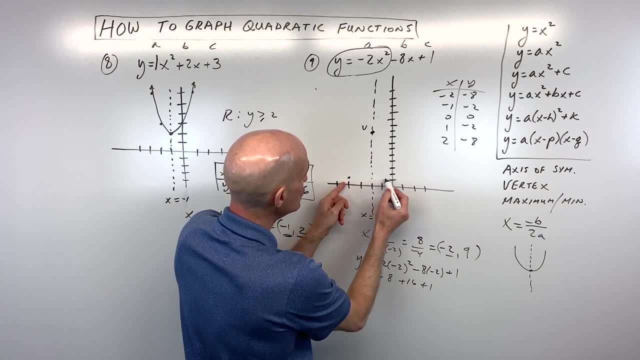 down eight. Okay, So let's see that would be right about here. And then the thing is, you can then reflect it over this line of symmetry. So see how I'm two units away If I go two units on the other side of. 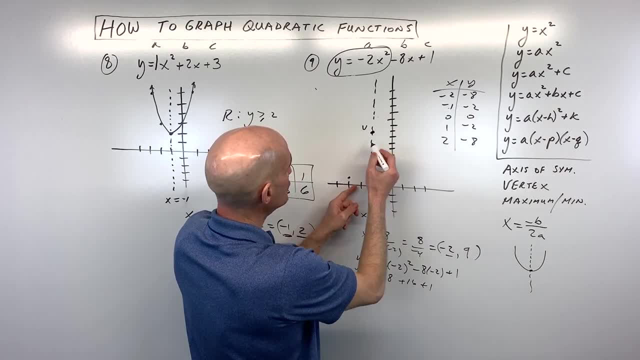 the axis of symmetry. I have another point And negative one, negative two. So from here I'm going left one down two And see how I'm one unit away If I go one unit, on the other side I have another. 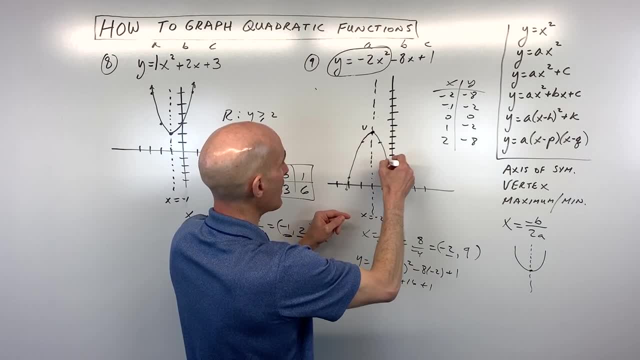 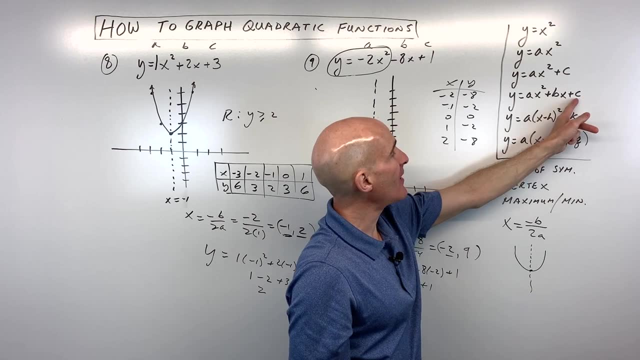 point, And now we have our graph. Now, another key point you want to pay attention to is when you're working with either this form or this form, see the c value. The c value is the y-intercept. It's where it crosses the y-intercept And it's where it crosses the y-intercept And it's where it crosses the. 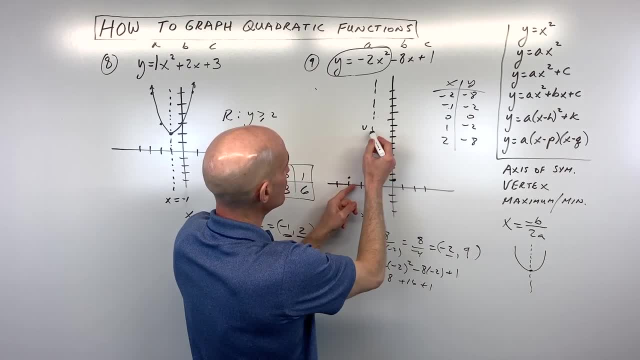 of symmetry. I have another point And negative 1, negative 2, so from here I'm going left 1, down 2.. And see how I'm one unit away. If I go one unit on the other side, I have. 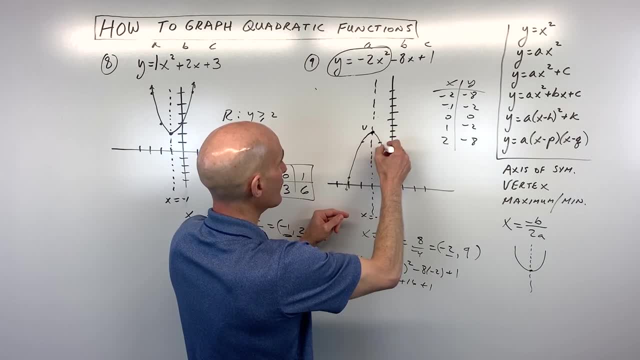 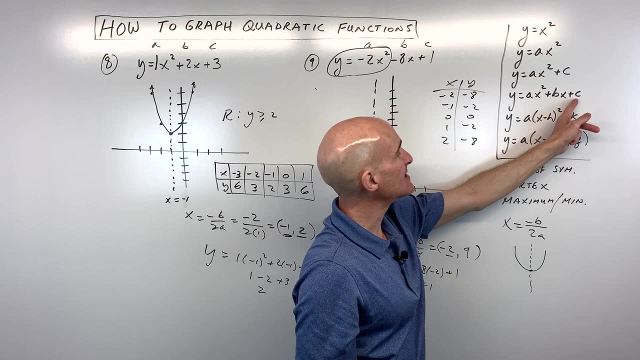 another point, And now we have our graph. Now, another key point that you want to pay attention to is when you're working with either this form or this form, see the c value. The c value is the y intercept. It's where it. 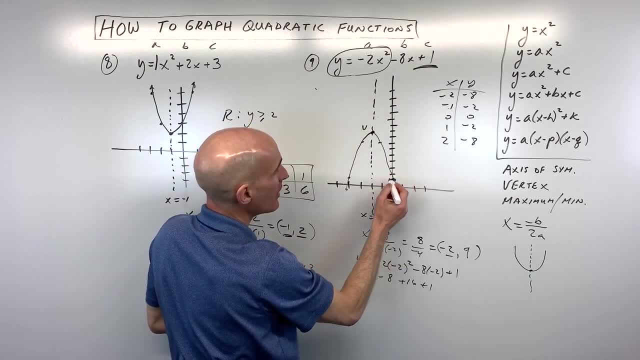 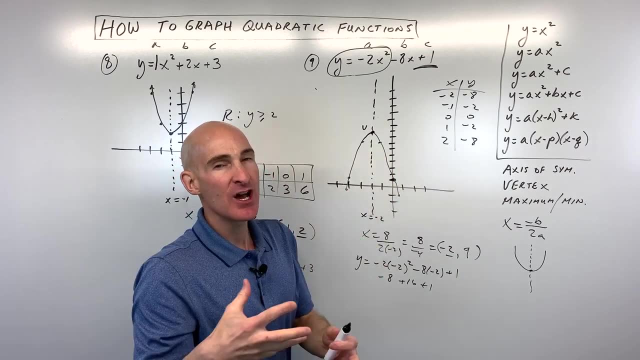 crosses the y axis. Now this is 1.. See how it's crossing right here at 1?. So it's an easy point to locate And then, once you know that point, you can then reflect it over the line of symmetry to get another point. Usually you want to have 3 points, ideally 5 points to get a nice. 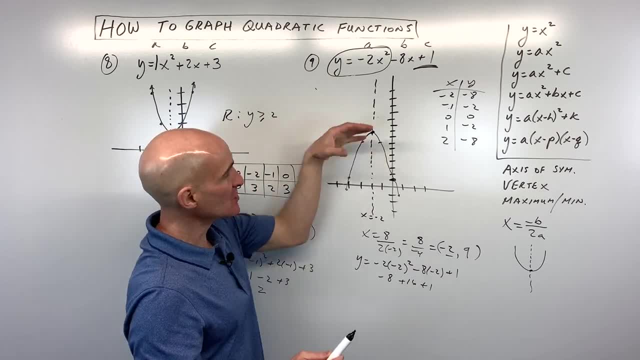 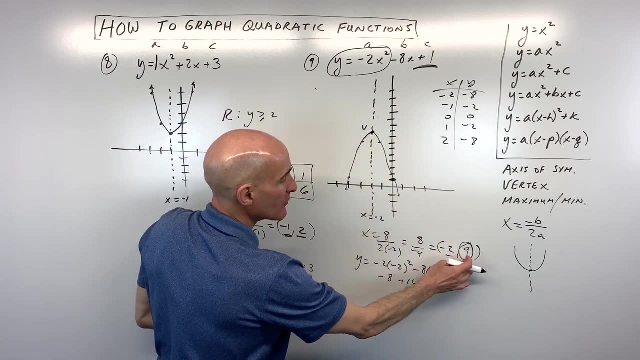 smooth graph. Now, this graph has a maximum right because it's opening down. It has a high point. It's like top of the hill here. And what is the maximum? Well, it's going to be the y coordinate of the vertex. It's going to be 9.. The range is going to be y. 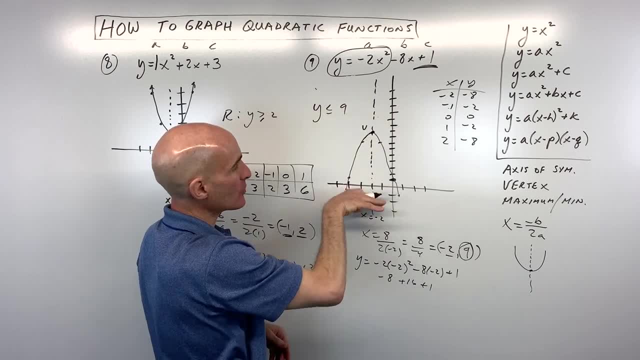 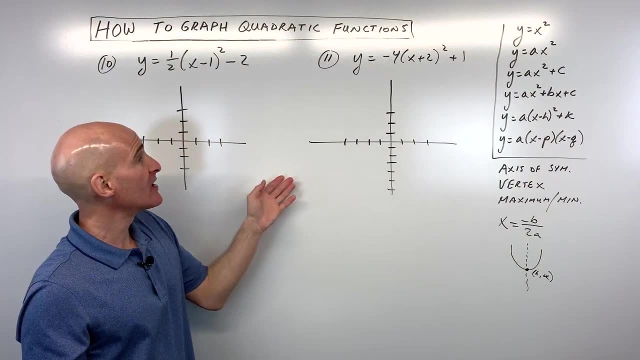 is less than or equal to 9.. See, it's 9 or below. And the domain, because this graph gradually goes to the left and right forever and ever. the domain is again all real numbers. Okay, number 10 and number 11,. we're going to talk about the vertex form now. That's. 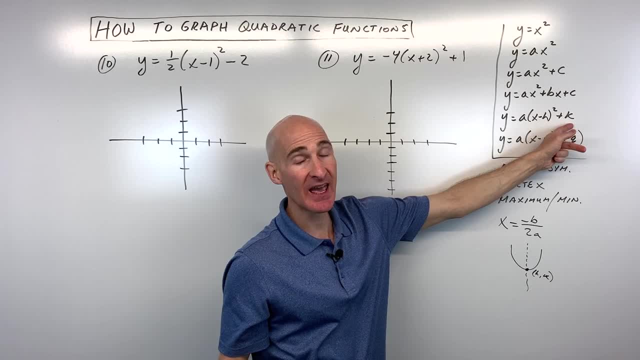 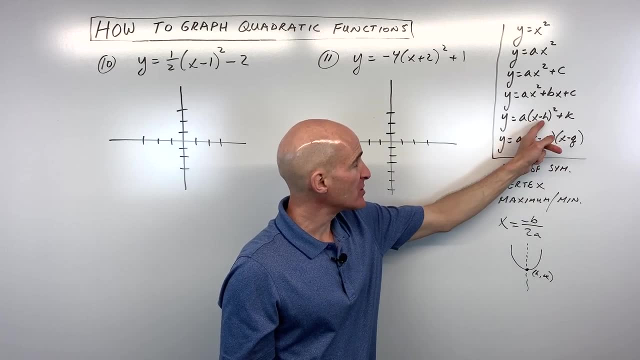 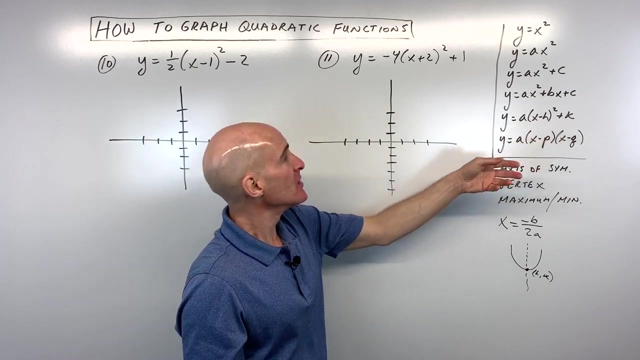 this: y equals a times the quantity x minus h squared plus k, And the vertex, that point where the graph bends, you know the maximum or the minimum point. that vertex point is going to be at h comma k. Now where students sometimes get a little bit confused is see how this is x minus h. 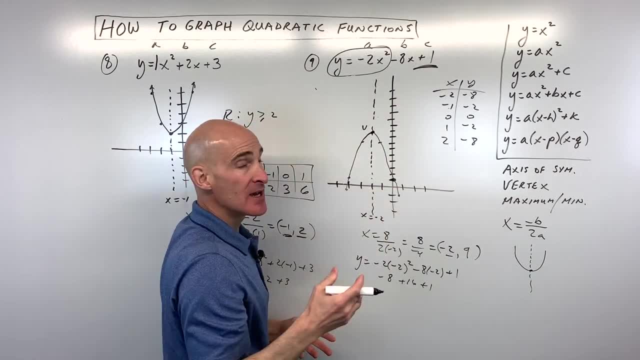 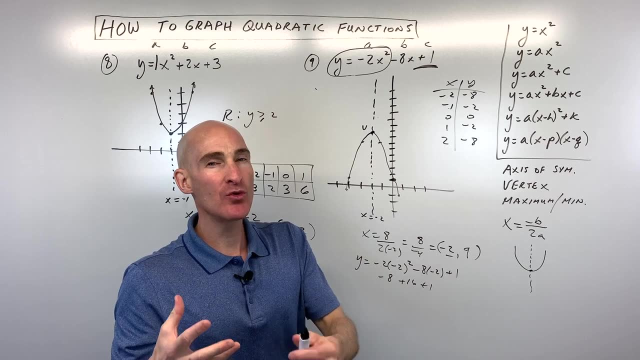 y-axis. So see how this is one, See how it's crossing right here at one. So it's an easy point to locate. And then, once you know that point, you can then reflect it over the line of symmetry to get another point. Usually you want to have three points, ideally five points to get a nice smooth. 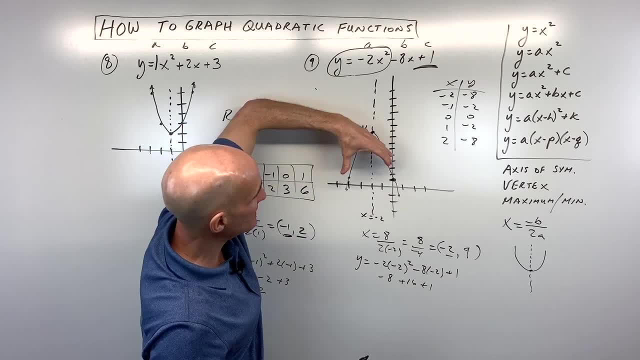 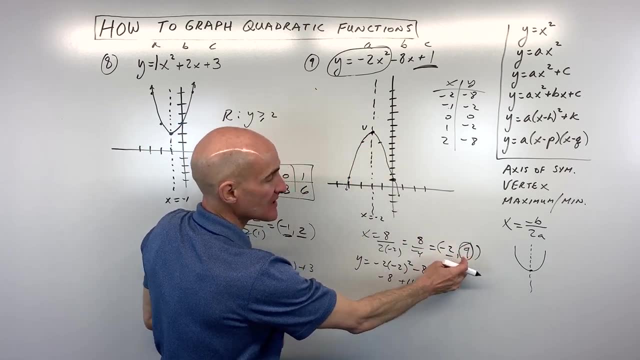 graph. Now, this graph has a maximum right Because it's opening down. It has a high point, It's like top of the hill here. And what is the maximum? Well, it's going to be the y-coordinate of the vertex. It's going to be nine, The range is going to be: y is less than or equal. 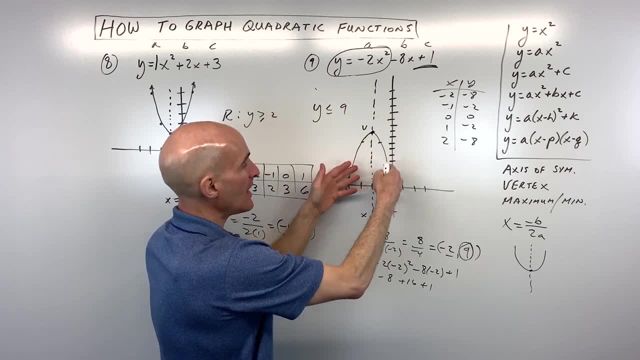 to the y-coordinate of the vertex, And that's going to be the y-coordinate of the vertex. So it's going to be: y is less than or equal to nine. See, it's nine or below, And the domain, because this graph gradually goes to the left and right, forever and ever, the domain- is again. 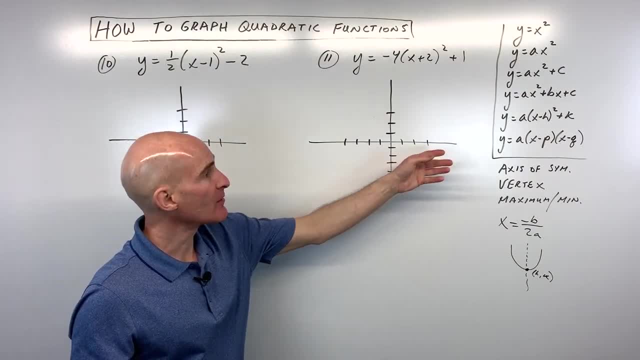 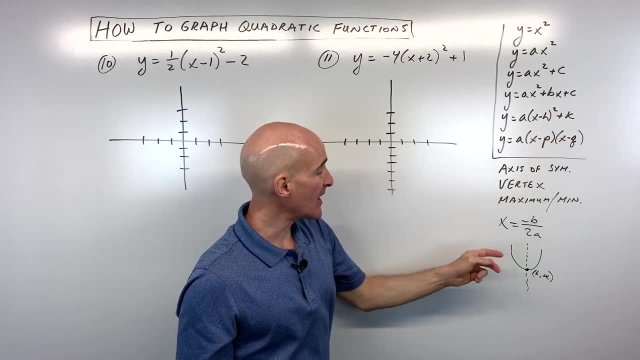 all real numbers. Okay, number 10 and number 11, we're going to talk about the vertex form now. That's this: y equals a times the quantity x minus h squared plus k, And the vertex, that point where the graph bends. you know the maximum or the minimum point. that vertex point is going to be. 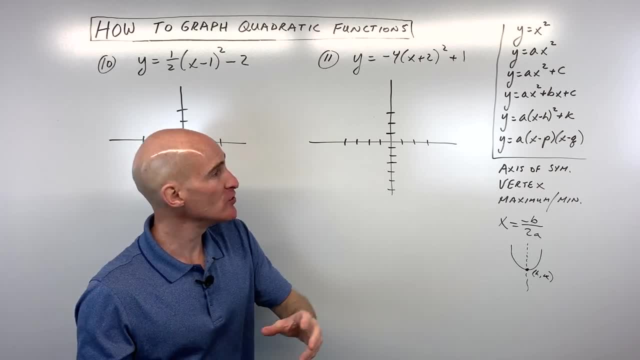 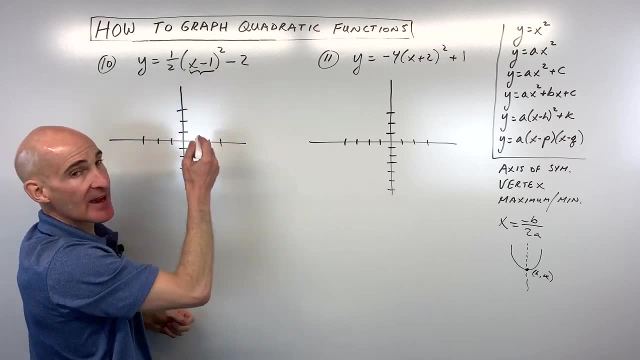 at h comma k. Now where students sometimes get a little bit confused is see how this is x minus h. So what you want to pay attention to is this number here, that's in the parentheses with the x. That number, that h value is going to be the opposite from this sign. So see, this looks like. 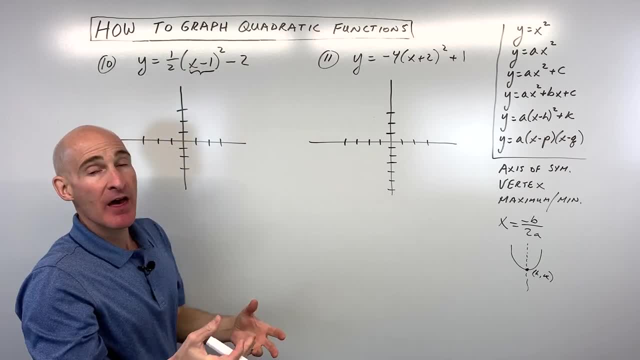 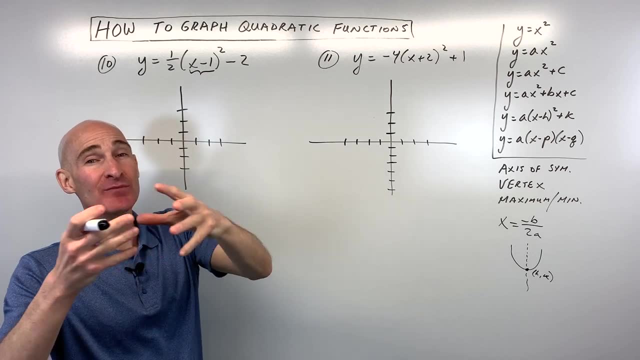 What we want to pay attention to is this number here that's in the parentheses with the x. That number, that h value, is going to be the opposite from this sign. So see, this looks like it's negative 1? It's actually going to be the opposite: It's going to be positive. 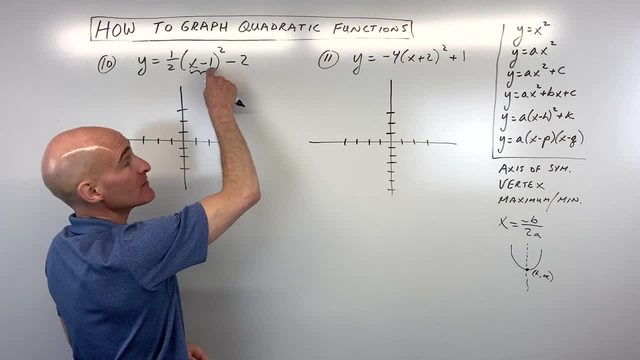 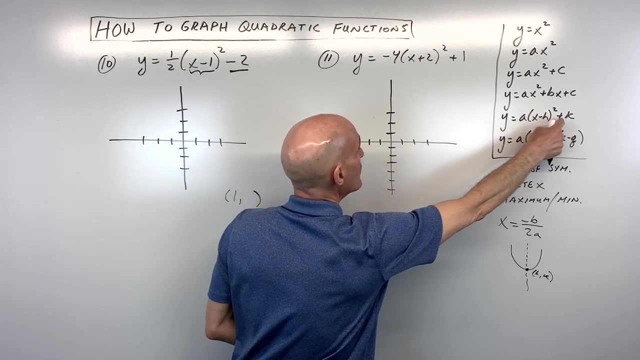 1.. It's actually x minus and then h is actually positive 1.. So that's our vertex: 1.. And then the k value. this is going to be the same sign. So see, this is minus 2 or negative 2.. 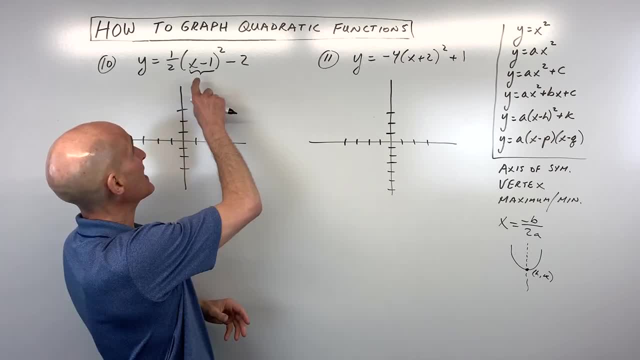 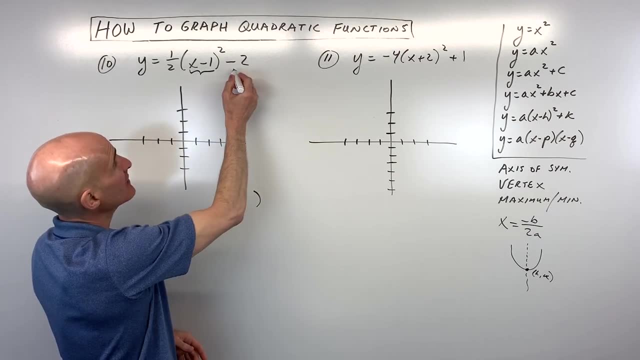 it's negative one. It's actually going to be the opposite: It's going to be positive one. It's actually x minus, and then h is actually positive one. So that's our vertex one, And then the k value. this is going to be the same sign. So see, this is minus two or negative two. It's going to. 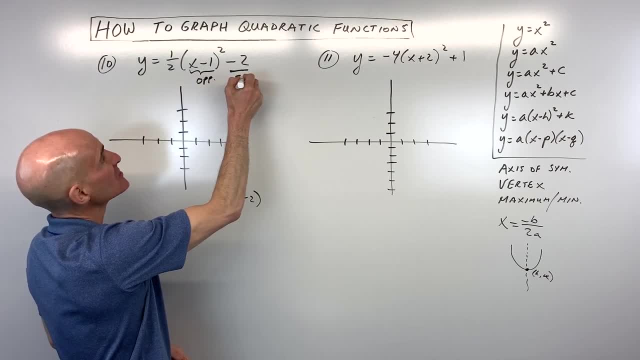 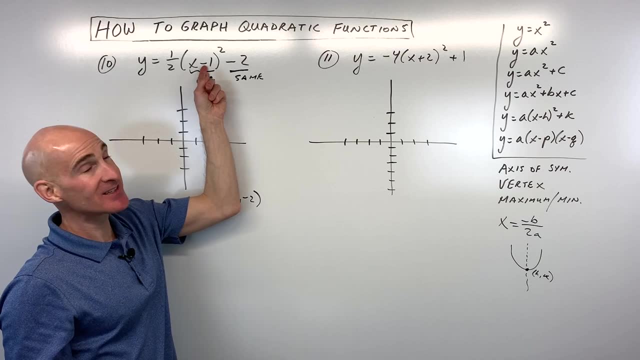 be negative two. So just remember: this one is the opposite. And then the k value: this is going to be negative one And this one here is the same as the sign. Some students that I tutor their teacher will say: well, this one lies and this one tells the truth. And I find that kind of 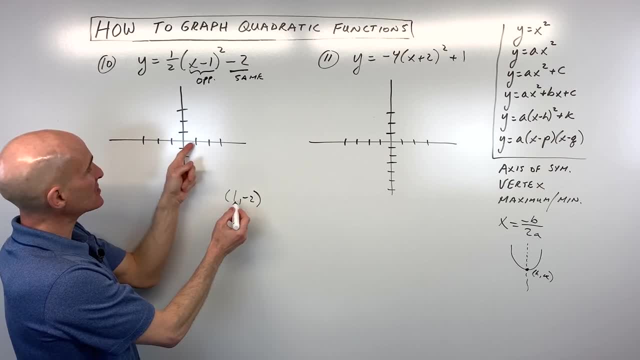 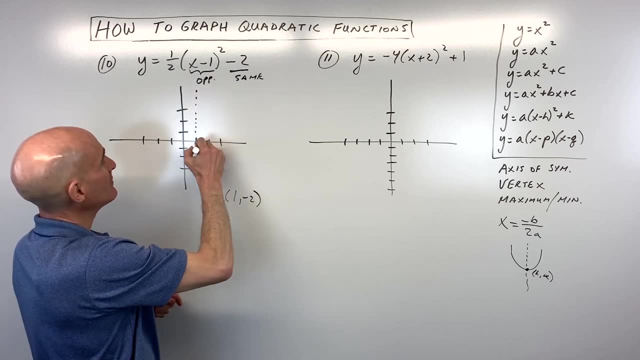 humorous, But if it helps you remember, that's always good. So let's see. So the vertex here is right. one down two. Okay, so that's your vertex. And then here's your line of symmetry, right, that divides the parabola in half. If you fold it over that line, it matches to itself. And now 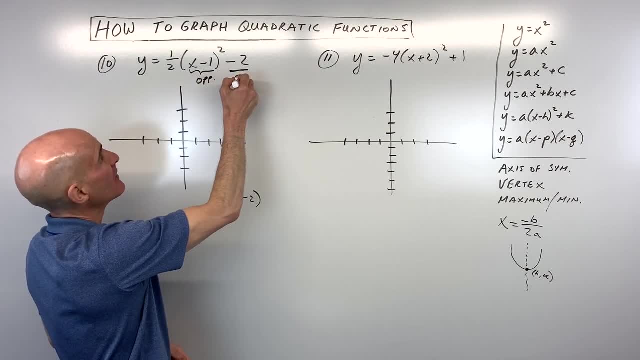 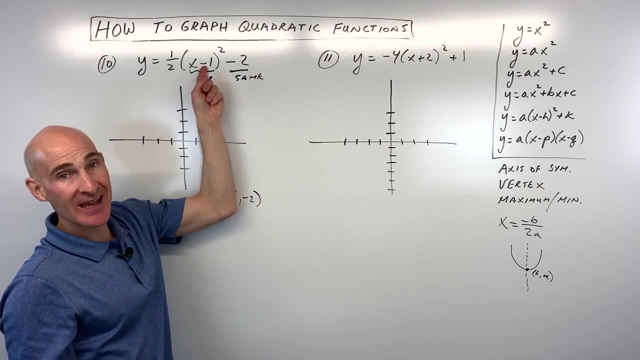 It's going to be negative 2.. So just remember, this one is the opposite and this one here is the same as the sign. Some students that I tutor their teacher will say: well, this one lies and this one tells the truth, And I find that kind of humorous. But if it helps you remember, that's always. 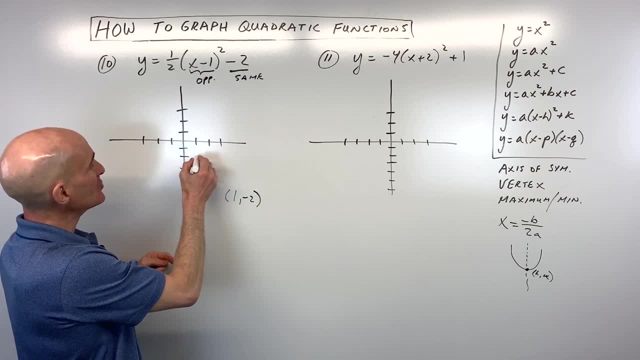 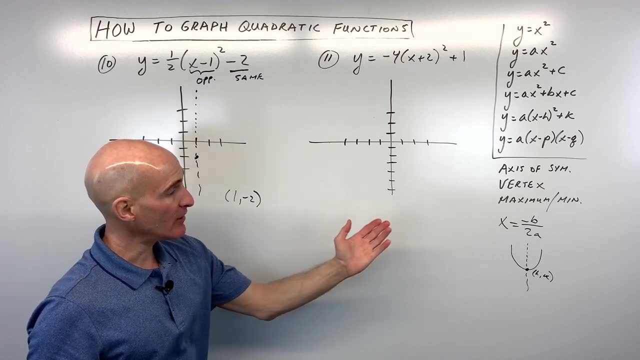 good, So let's see. So the vertex here is: right 1, down 2.. Okay, so that's your vertex. And then here's your line of symmetry, right. that divides the parabola in half. If you fold it over that line, it matches to itself, And now you have a lot of different options. 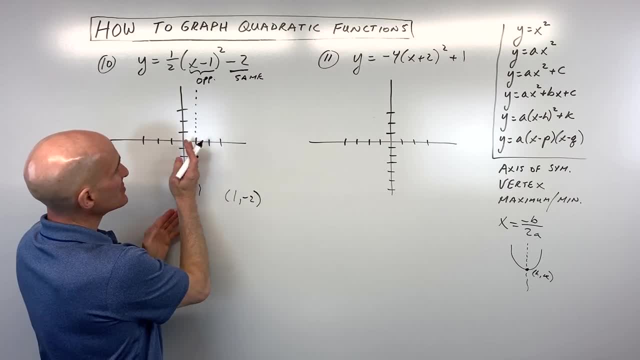 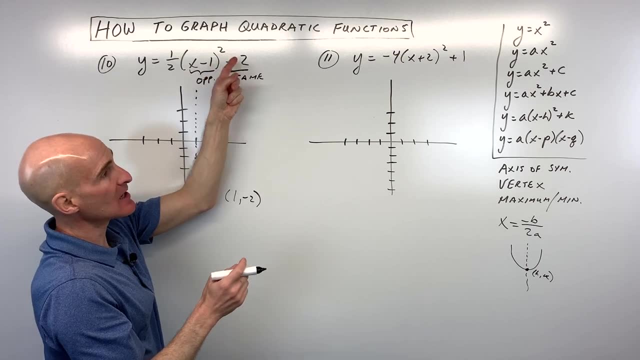 One option is you could say: well, let me just pick some points on either side of this point, Okay. Or let me look at the parent function: y equals 1 half x squared. See, I'm basically looking at this: y equals ax squared, form and graph from here as if it's the origin. 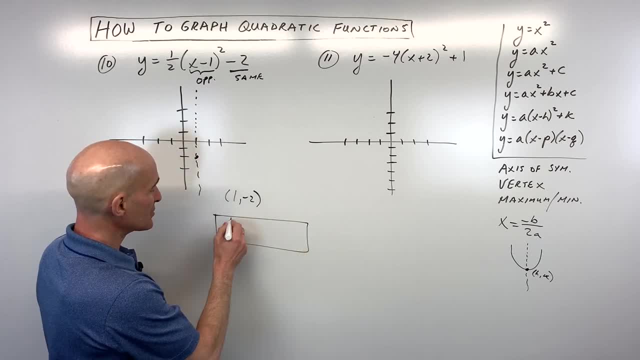 A lot of different options. I'm just going to make a table. I think this is a student's most favorite method: Put the vertex in the middle and then pick some points on either side. So I'm going to put 0 and negative, 1 and 2 and 3.. So all I'm doing is adding 1. 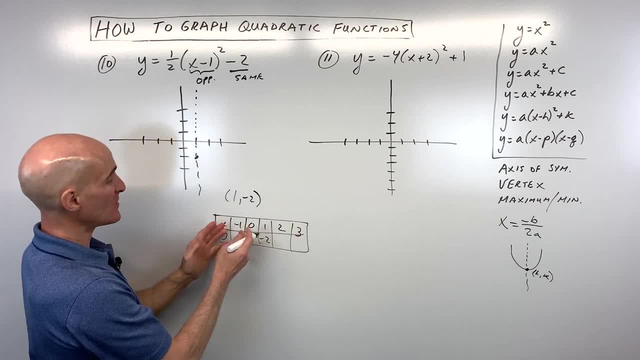 or subtracting 1, adding 2 or subtracting 2.. So it's basically it's the same on both sides. So let's put 0 in. 0 is usually easy to work with. 0 minus 1 is negative 1.. Negative 1. 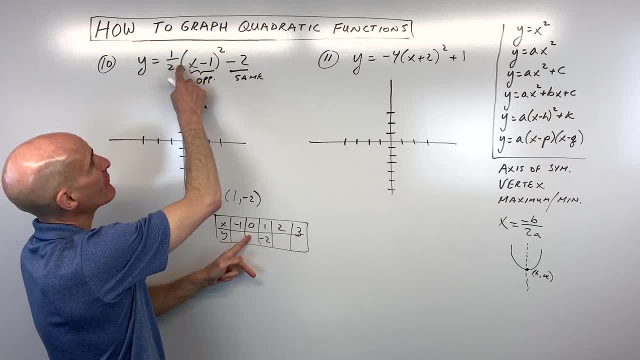 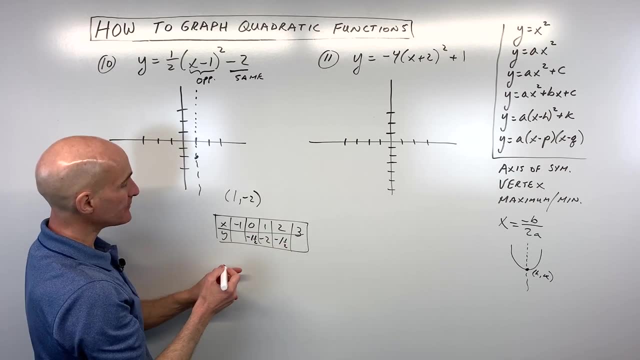 squared is positive 1. Times a half is a half, Minus 2 is negative 1 and a half. So that means this one over here is also negative 1 and a half, And if we put in, let's say 3. 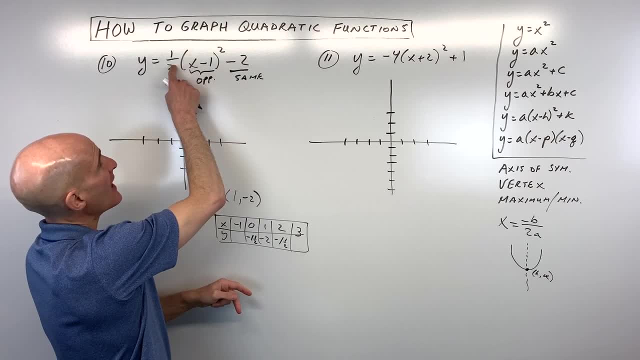 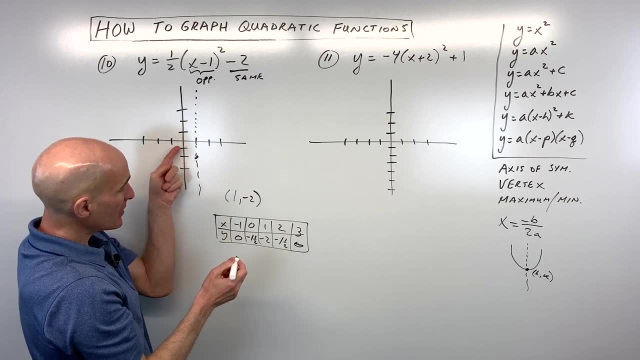 now, 3 minus 1 is 2.. 2 squared is 4.. Times a half is 2.. Minus 2 is 0. So that means this one over here will also be 0.. It's the same on both sides. So now we can graph, If you. 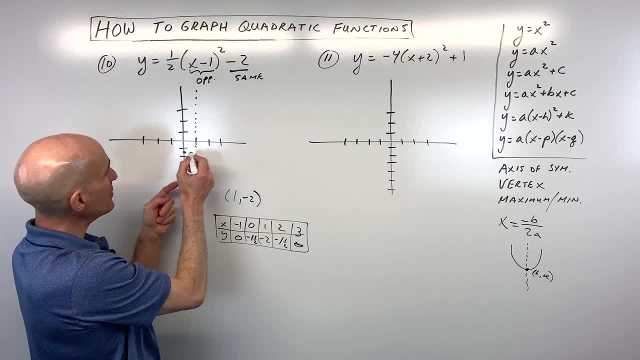 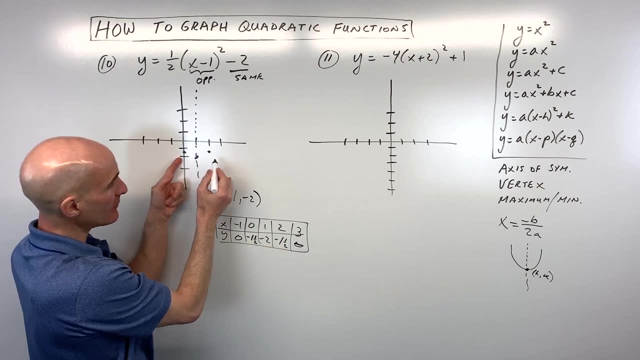 got 0, negative 1 and a half, which is right here. Fold it over that line of symmetry- See, it's going to be right there- which is the same as 2, and then comma negative 1 and a half, And then we have 3, 0. And again I can reflect it over that line of symmetry. 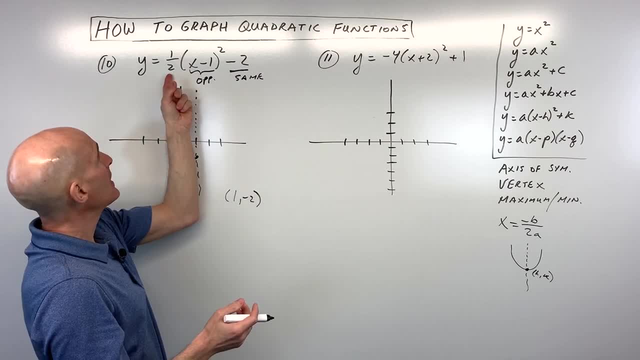 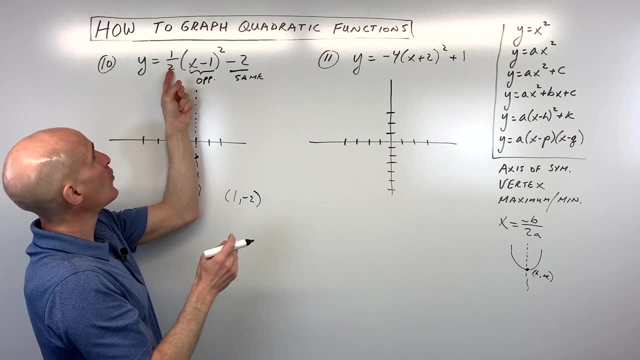 you have a lot of different options. One option is you could say, well, let me just put this in the middle and pick some points on either side of this point, Okay. Or let me look at the parent function: y equals one half x squared. See, I'm basically looking at this: y equals ax squared form. 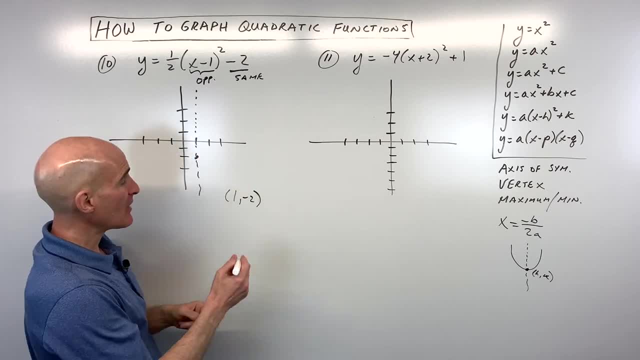 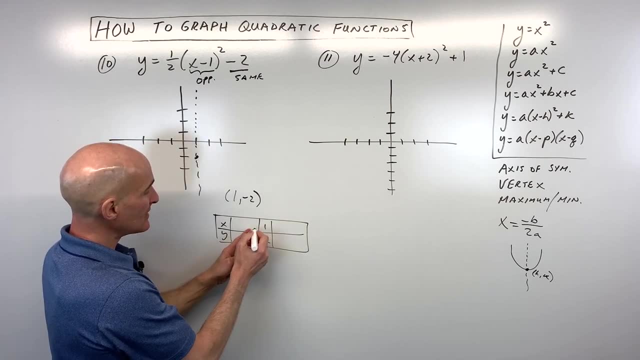 and graph from here as if it's the origin A lot of different options. I'm just going to make a table. I think this is a student's most favorite method: Put the vertex in the middle and then pick some points on either side. So I'm going to put zero and negative, one and two and three. So 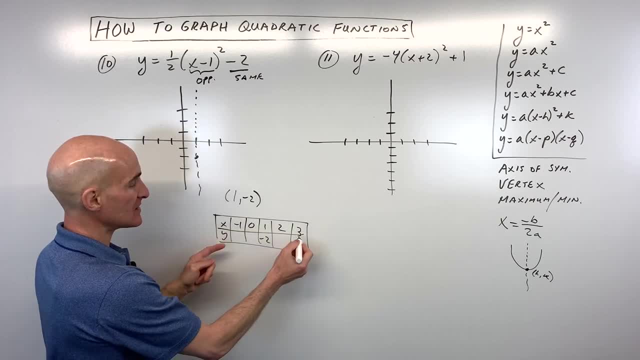 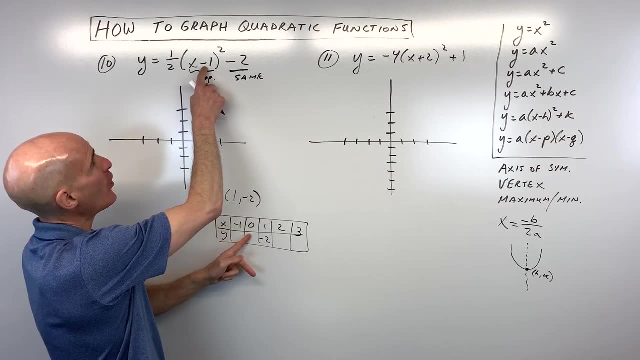 all I'm doing is adding one or subtracting one, adding two or subtracting two. So I'm going to. basically it's the same on both sides. So let's put zero in. Zero is usually easy to work with. Zero minus one is negative, one Negative, one squared is positive. one times a half is a half. 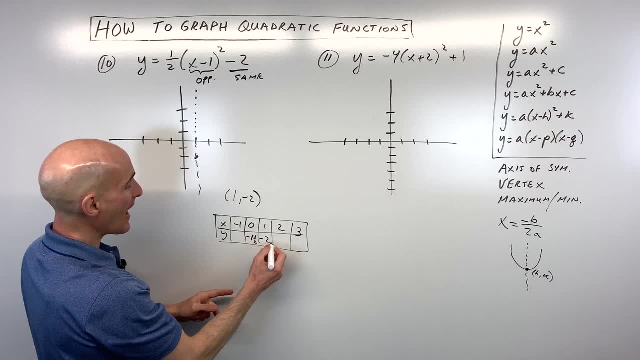 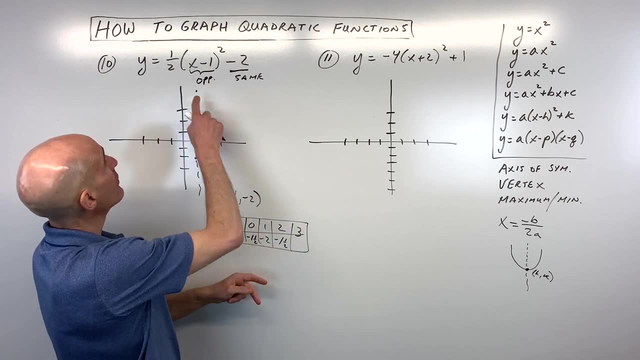 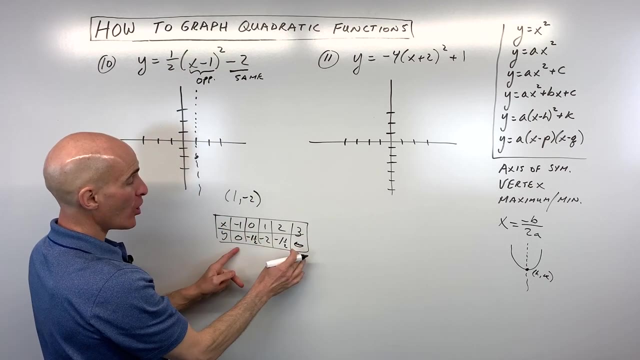 minus two is negative one and a half. So that means this one over here is also negative one and a half. And if we put in, let's say, three: now three minus one is two. Two squared is four times a half is two minus two is zero. So that means this one over here will also be zero. It's. 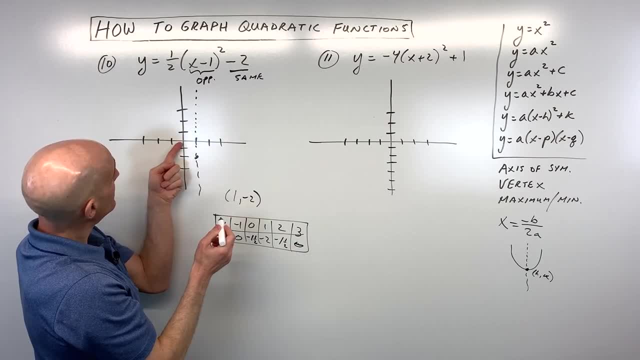 the same on both sides. So now we can graph. We've got zero, negative one and a half, which is right here, And I fold it over that line of symmetry. See, it's going to be right there, which is the. 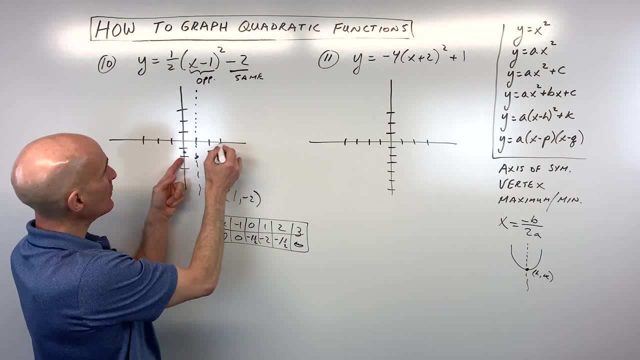 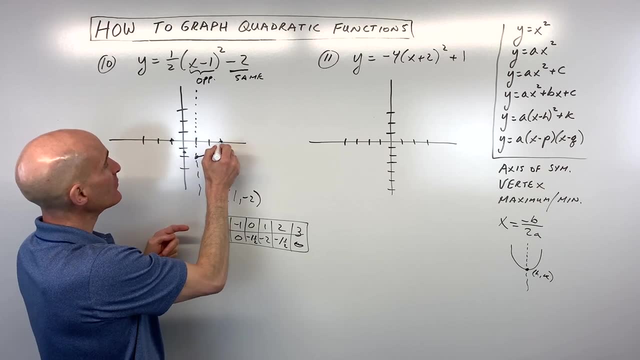 same as two, and then comma negative one and a half, And then we have three zero, And again I can reflect it over that line of symmetry. or negative one zero right here. And one thing you'll be noticing about this graph is that because of the one half it's a little bit wider. 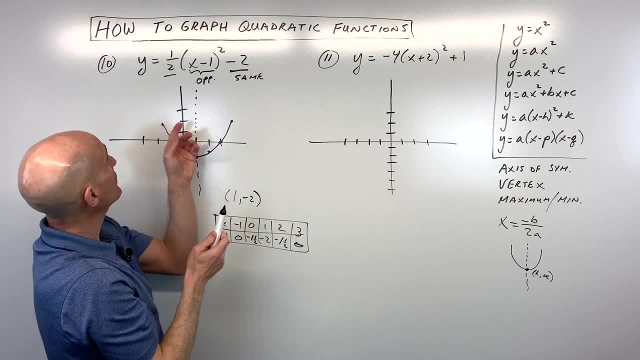 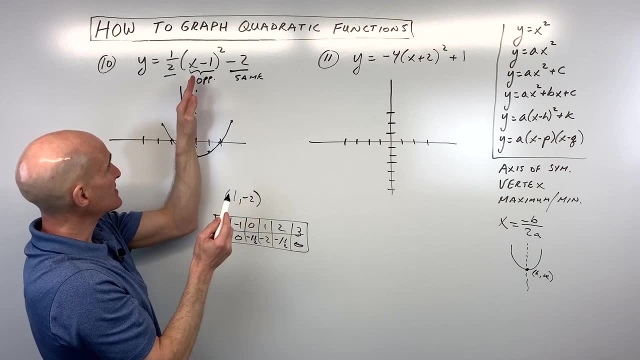 right. So it's opening up wider And what else? We know that it's opening up because a value is positive. This has a minimum value. That minimum value is going to be at negative two. The axis of symmetry is going to be right here through the x coordinate of the. 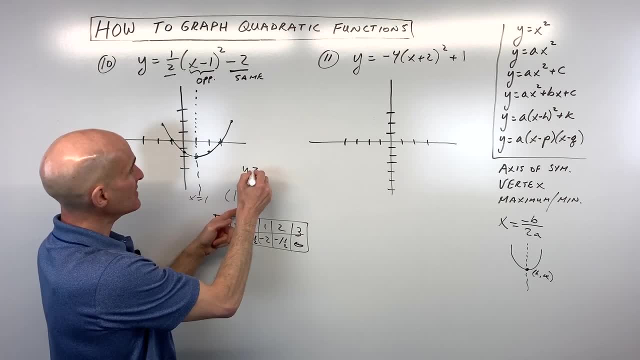 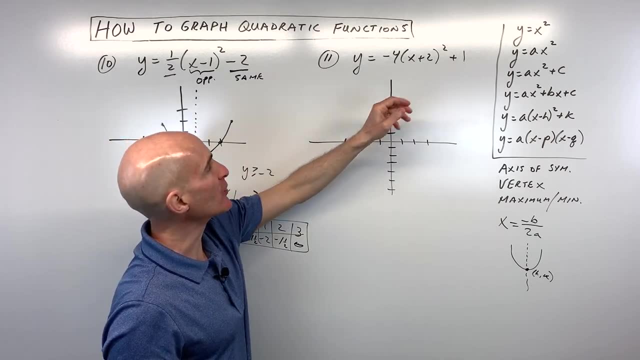 vertex x equals one And the range is going to be: y is greater than or equal to negative two, And we covered it right. So let's look at number 11.. A little bit different here. See if you can do this one on your own. What's the vertex? What do you think the vertex is of this quadratic? 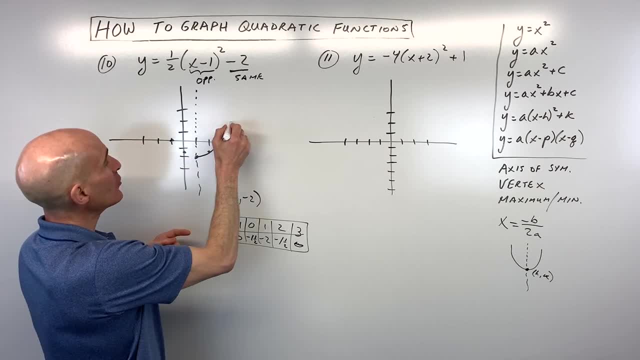 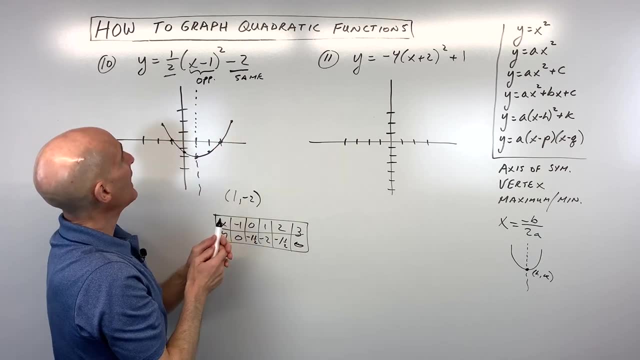 or negative, 1, 0 right here. And one thing you'll be noticing about this graph is that because of the 1 half, it's a little bit wider Right, So it's opening up wider And what else. We know that it's opening up because the a value is positive. This half is going. 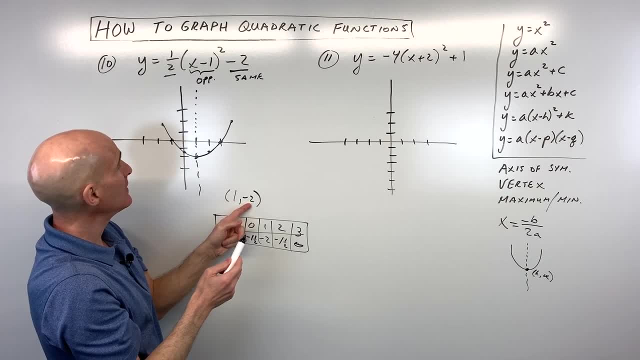 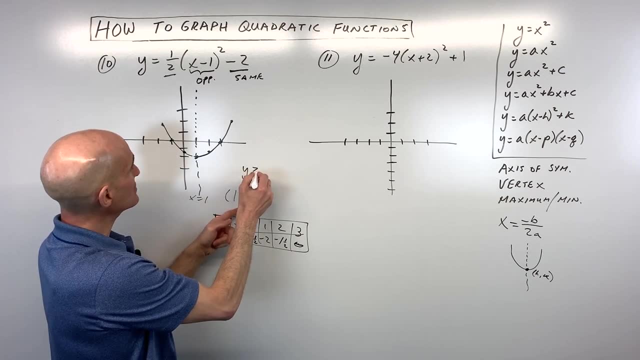 to be positive. This has a minimum value. That minimum value is going to be at negative: 2.. The axis of symmetry is going to be right here, through the x coordinate of the vertex. x equals 1. And the range is going to be: y is greater than or equal to negative, 2. And 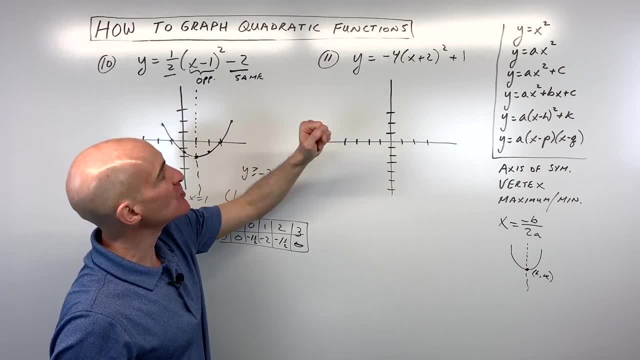 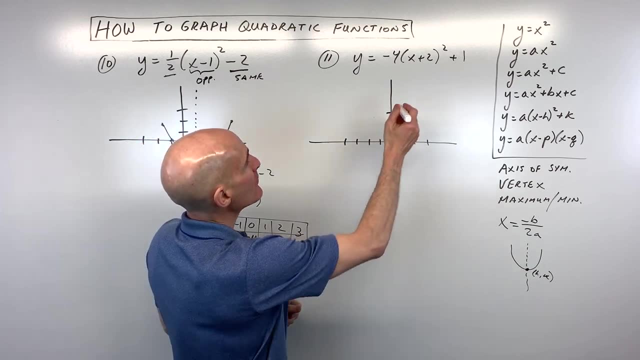 we covered it right, So let's look at number 11.. A little bit different here. See if you can do this one on your own. What's the vertex? What do you think the vertex is of this quadratic? Well, remember this one. we said it lies right, Or it's the opposite right. The plus 2 is: 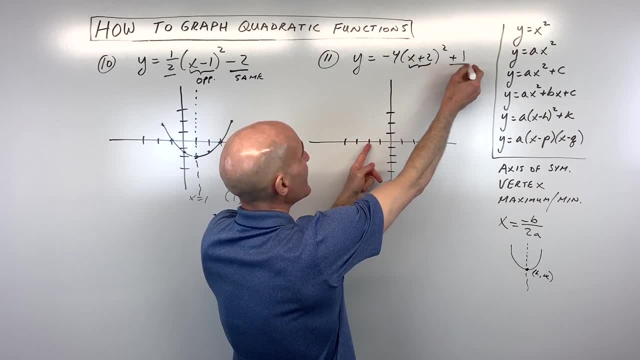 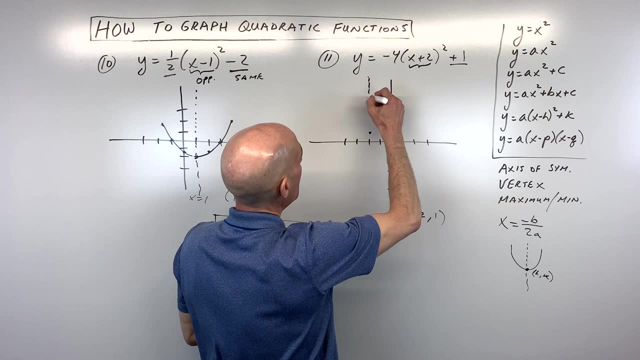 actually going to shift left 2.. Plus 1 is the same, So it's going to go positive 1, up 1.. So there's our vertex right there, at negative 2, positive 1.. Here's our axis of symmetry. I just like to draw it as a dashed. 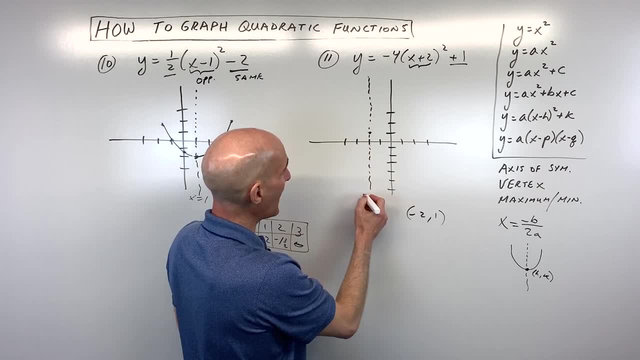 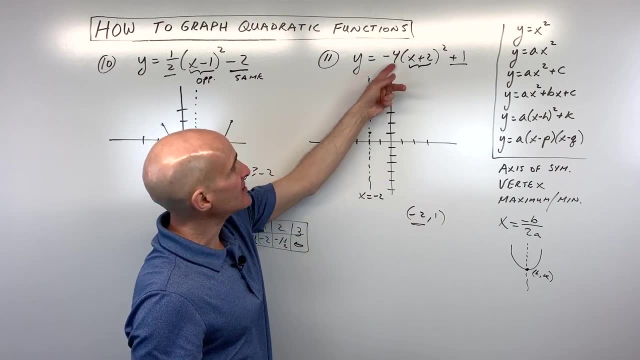 or dotted line. You won't really see that when you graph the parabola. We're just using it as a guide. Our axis of symmetry is: x equals negative 2. Same as x coordinate of the vertex. The a value is negative. That tells us the parabola is going to be opening down right. 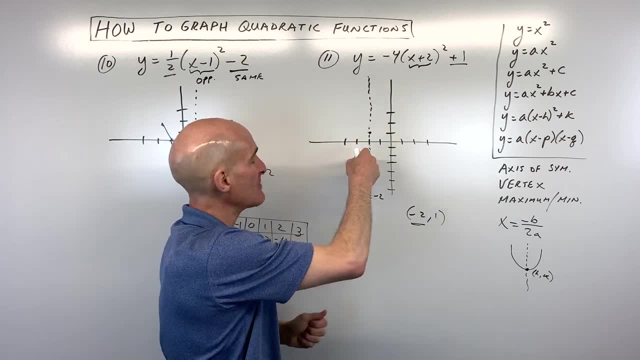 Negative, like frowning right, And the 4 is going to stretch it, So that means it's going to be very narrow. But now what we can do is we can use the same table method. I think again, like I said, 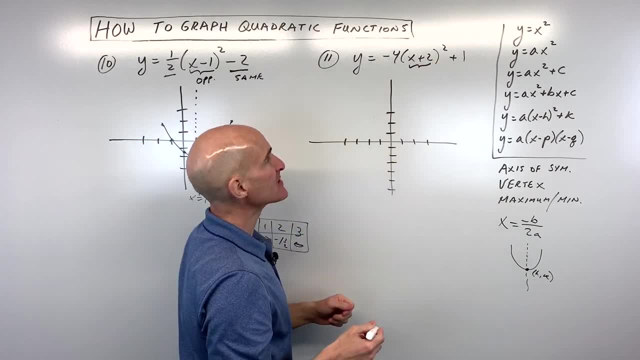 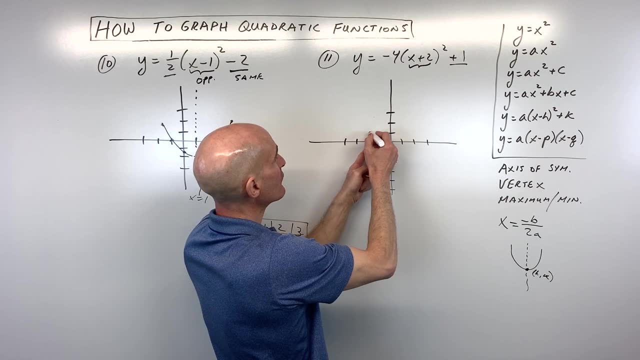 Well, remember this one. we said it lies right Or it's the opposite: right. The plus two is actually going to shift. left two And the plus one is the same, So it's going to go positive one up one. So there's our vertex, right there, at negative two, positive one. Here's our axis of. 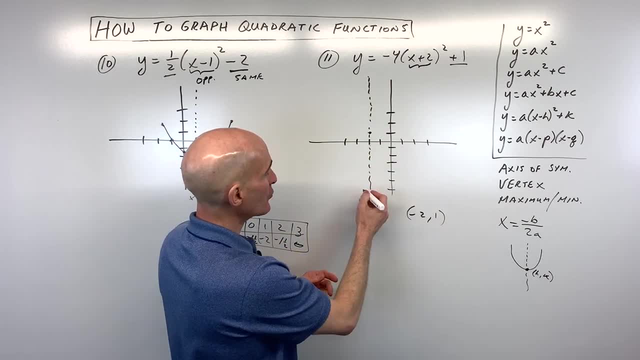 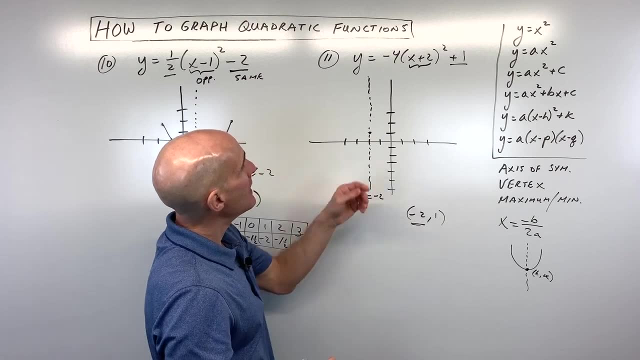 symmetry. I just like to draw it as a dashed or dotted line. You won't really see that when you graph the parabola. We're just using it as a guide. Our axis of symmetry is: x equals negative. two same as x. coordinate of the vertex, The a value is negative. That tells us the parabola. 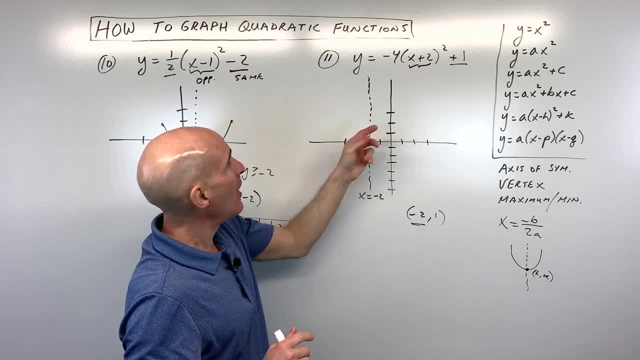 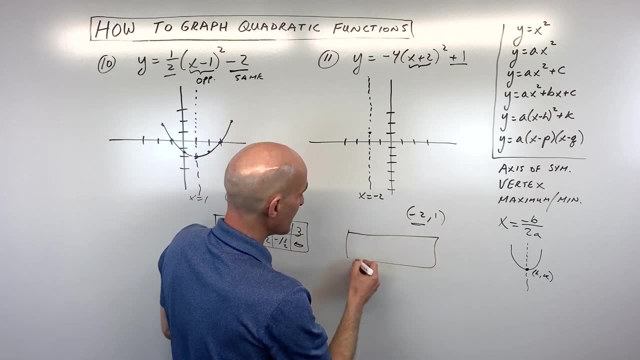 is going to be opening down right Negative, like frowning right, And the four is going to be very narrow. But now what we can do is we can use the same table method. I think again, like I said, this is probably students' favorite way of doing it. Put that vertex in the middle. 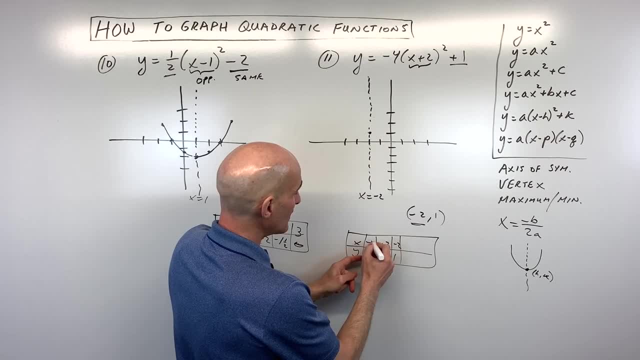 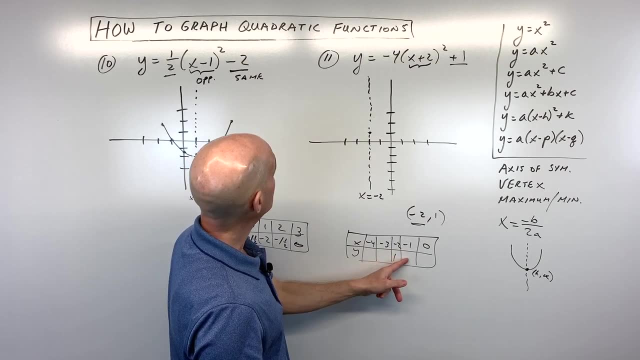 negative, two, one And let's pick some points on either side. So negative three, negative four, negative one and zero. So if we put in: let's see negative one, that would be pretty easy. Let's see negative one plus two is one. One squared is one times negative. four is negative. 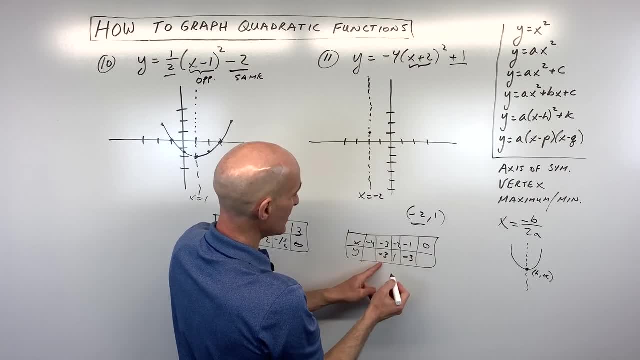 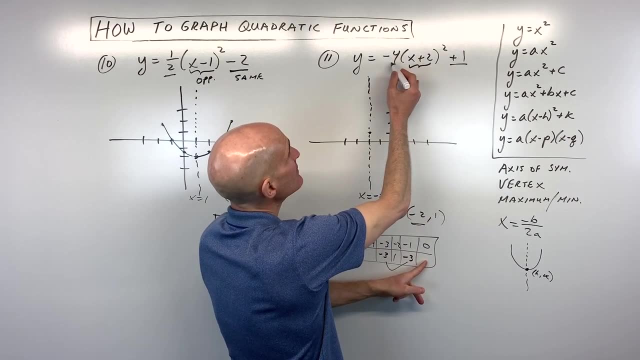 four plus one is negative three. So that means this one here is also negative three, right Same. If we put zero in zero, is easy to work with. Zero plus two is two. Two squared is four, Four times negative. four is negative. 16 plus one is negative 15.. That means this one over here is: 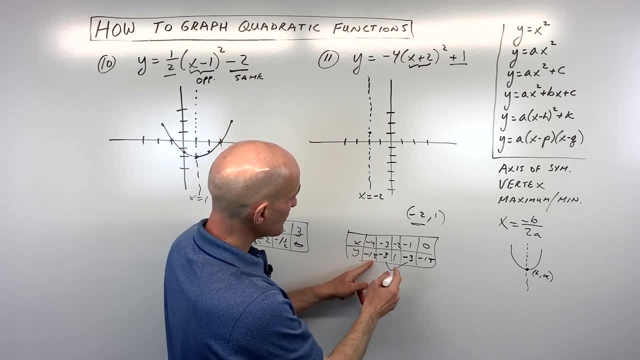 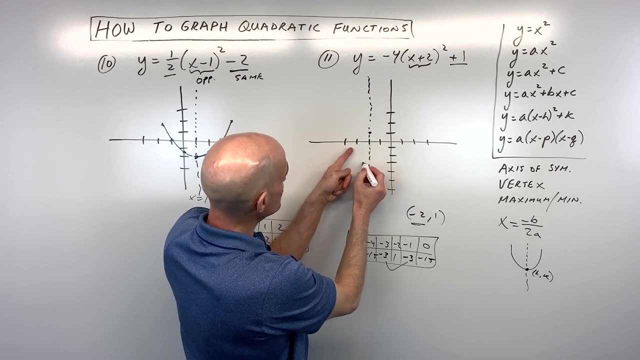 also negative 15.. These ones are probably going to go way off the graph, So let's just do these ones. in the middle We've got negative three, negative three, which is right here, And then we have negative one- negative three, which is right here. So you can see it's opening down. 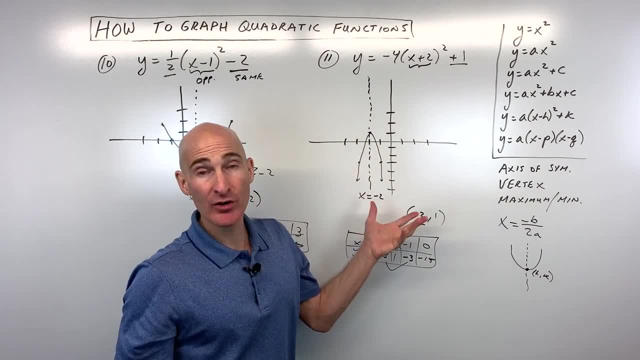 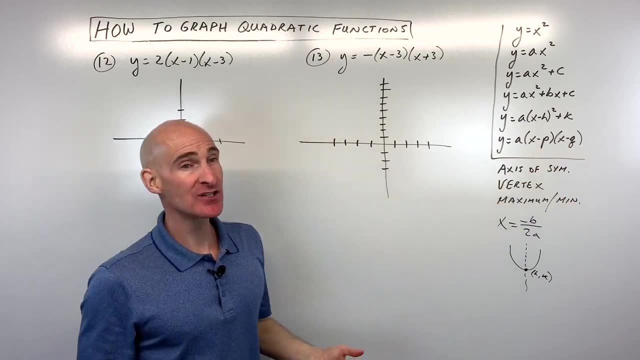 It's narrow And you've got a pretty good sketch of the graph Number 12 and number 13,. we're going to be working with what's called the intercept form of the equation of a quadratic, okay, of a parabola. 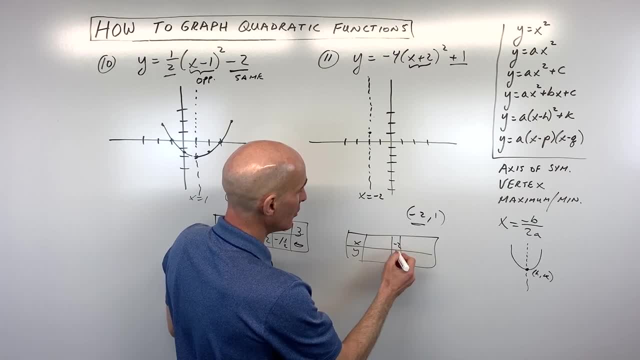 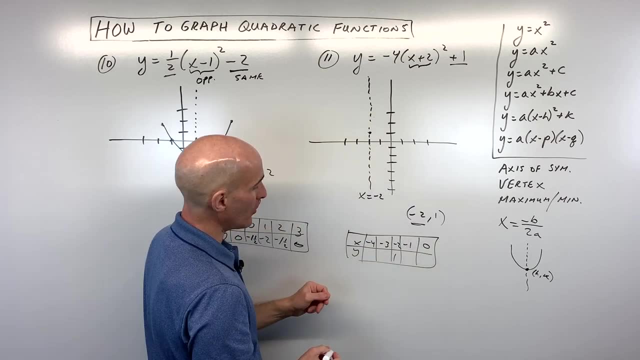 this is probably students' favorite way of doing it. Put that vertex in the middle: negative 2,, 1.. And let's pick some points on either side. So negative 3,, negative 4,, negative 1, and 0.. 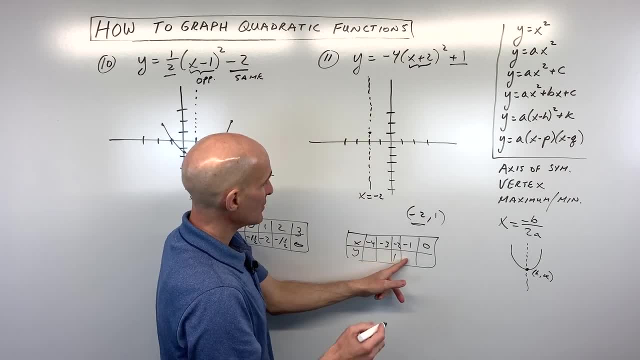 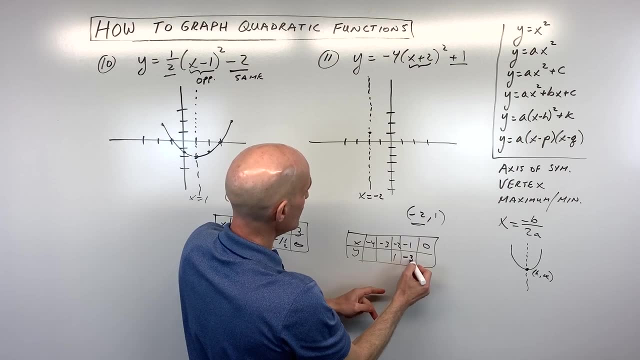 So if we put in let's see negative 1, that would be pretty easy- Let's see negative 1 plus 2 is 1.. 1 squared is 1 times negative. 4 is negative. 4 plus 1 is negative 3.. So that 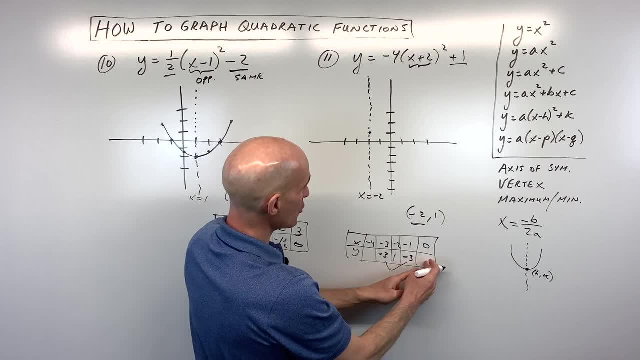 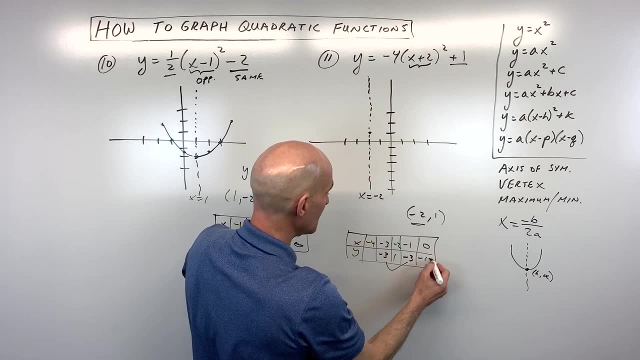 means this: one here is also negative. 3, right, They're the same. If we put 0 in, 0 is going to be easy to work with. 0 plus 2 is 2.. 2 squared is 4.. 4 times negative. 4 is negative. 16 plus 1 is negative 15.. That. 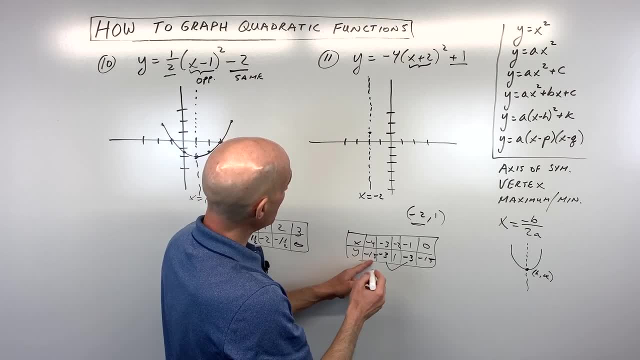 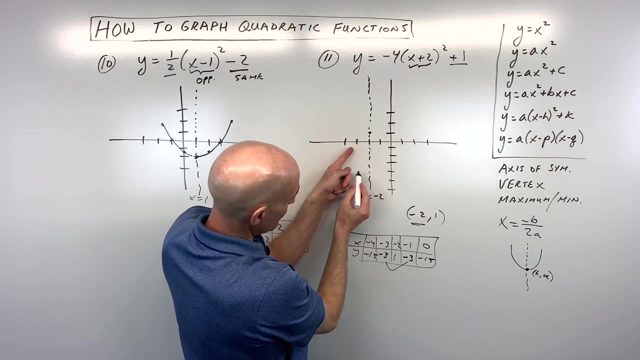 means. this one over here is also negative 15.. These ones are probably going to go way off the graph, So let's just do these ones. in the middle. We've got negative 3, negative 3,, which is right here, And then we have negative 1, negative 3,, which is right here. So you 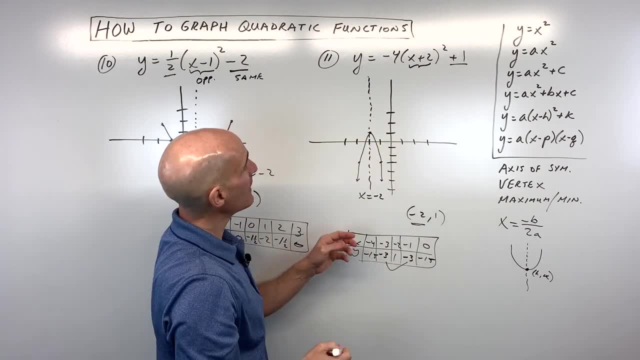 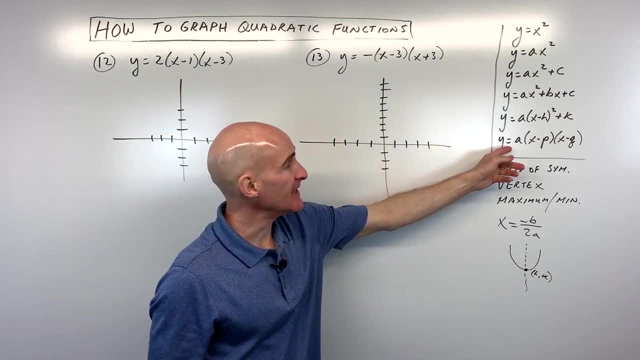 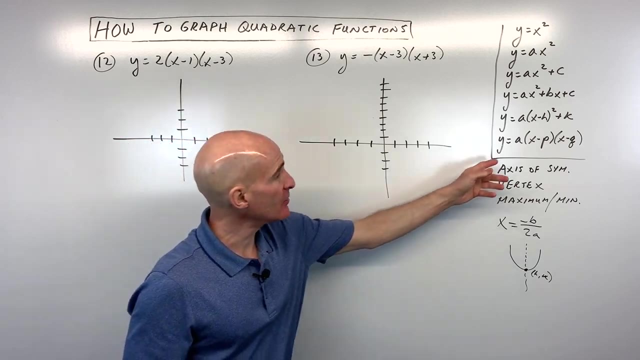 can see it's opening down, It's narrow, And you've got a pretty good sketch of that. So here's the graph, Number 12 and number 13,. we're going to be working with what's called the intercept form of the equation of a quadratic, okay, of a parabola, And the idea here is, with the intercept, 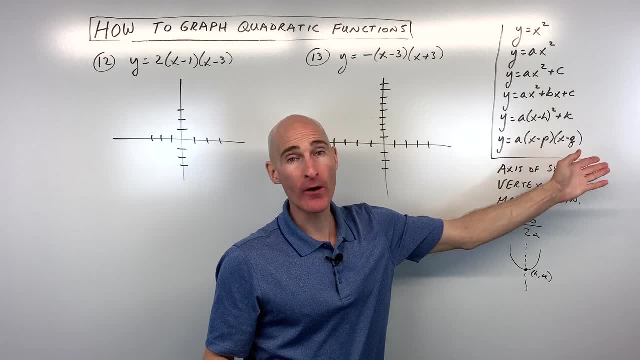 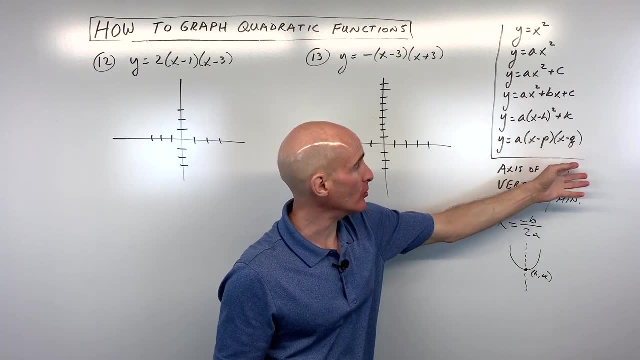 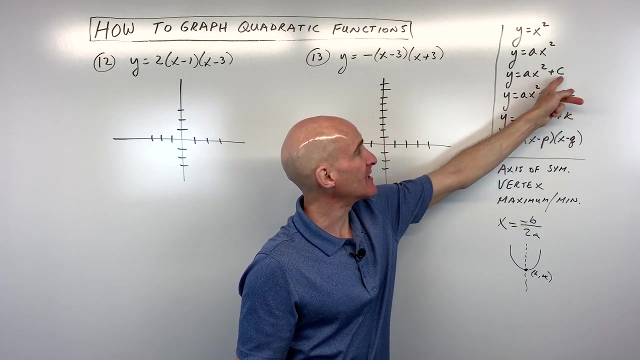 form is when it's in this form, this factored form, what we can easily identify are the x-intercepts, or what are often referred to as the zeros, Whereas over here, in the vertex form, we can easily identify the vertex In this form, here we can easily identify the. 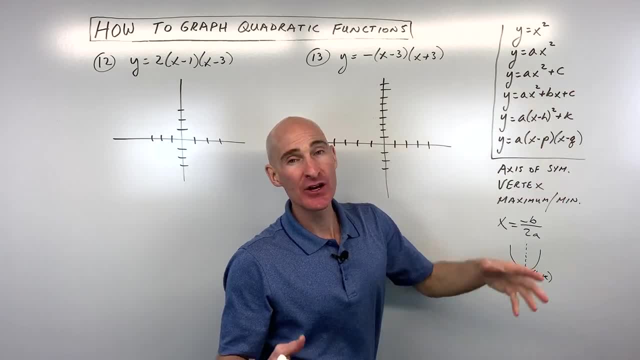 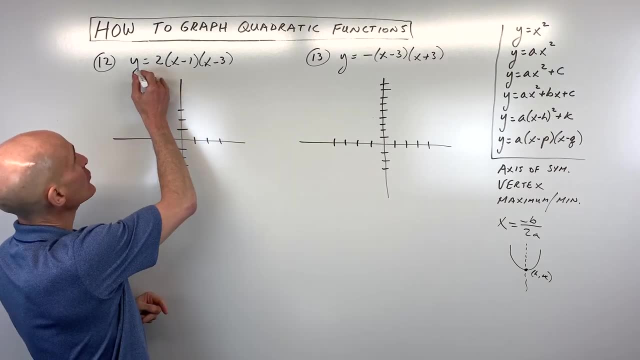 y-intercepts. Right, Because we have the c-values and the y-intercepts. So each form has kind of like its positives and its negatives, right? But for this one we can see it's in the factored form And the way we find those zeros. remember, the zeros means where the y-value is equal. 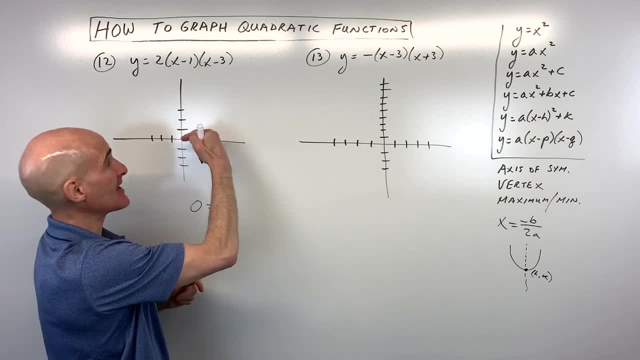 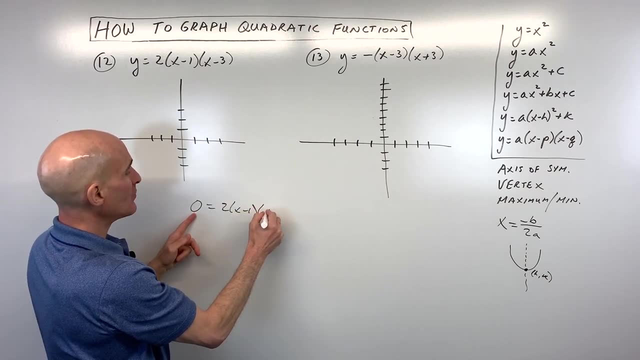 to zero. When y is zero, that means we're right along the x-axis, because we're not going up or down, And that gives us those x-intercepts. So what we do is we set y equal to zero, And what you do is you set these factors or these groups equal to zero, So you can make a mini. 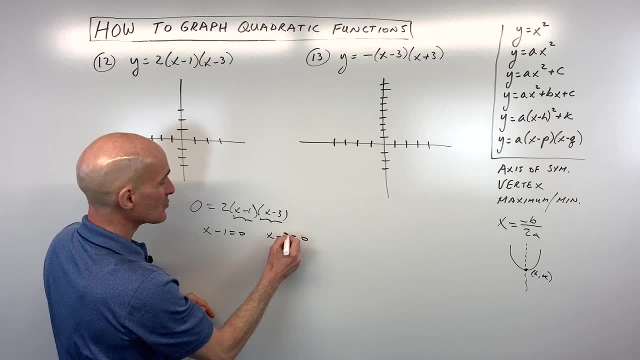 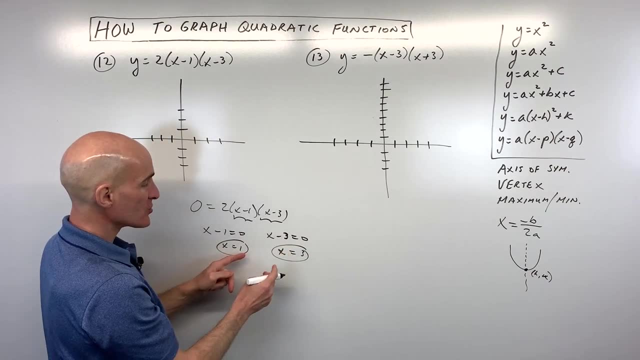 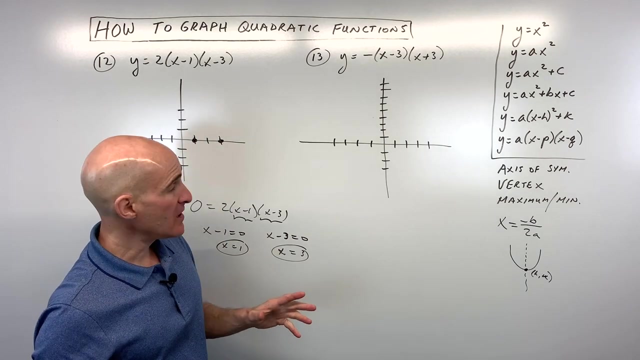 equation: x minus 1 equals zero And x minus 3 equals zero. Add 1 to both sides, Add 3 to both sides And you can see that our zeros or our x-intercepts are going to be at 1 and 3.. Now what we can do from here. 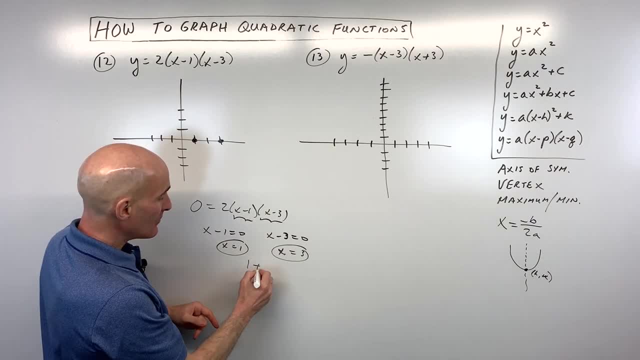 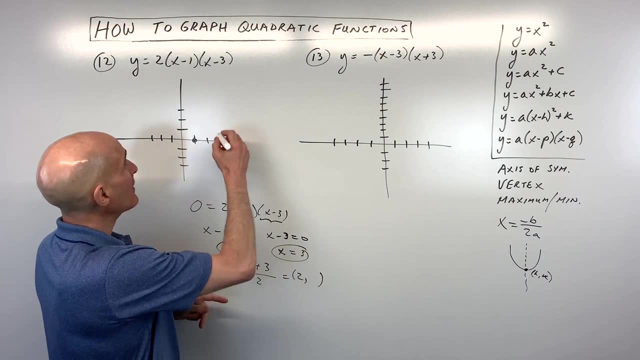 once we find these x-intercepts is we can add them together and divide by 2.. So 1 plus 3 is 4, divided by 2 is 2.. Now, what does that 2 do for us? Well, it gives us the axis of. 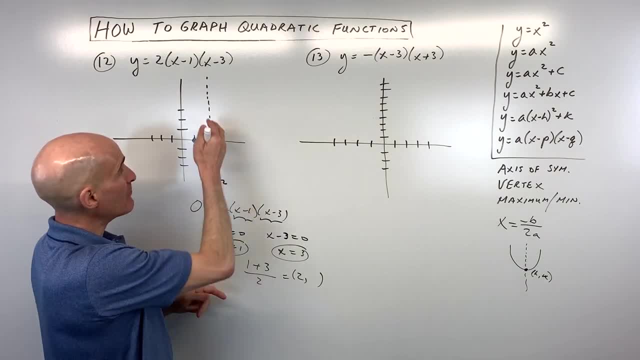 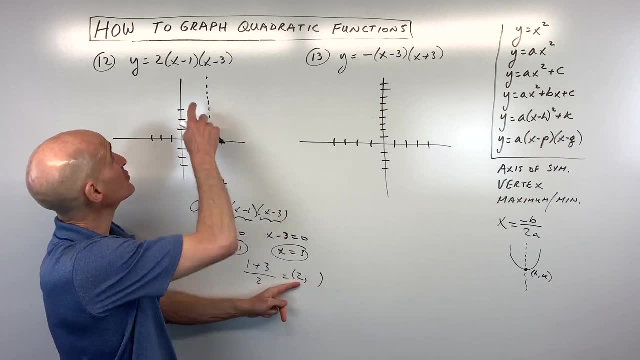 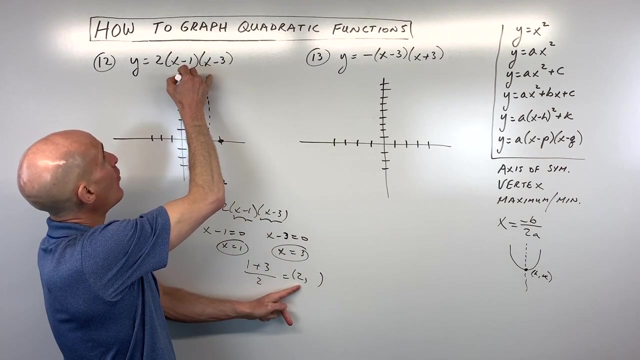 symmetry. OK, and because the vertex lies along that axis of symmetry, we know the x-coordinate of the vertex is going to be 2.. All we have to do now is put the 2 back in for x to find our y-coordinate of our vertex, and we got it. So let's do that. 2 minus 1 is 1, and 2 minus 3 is negative, 1 and so 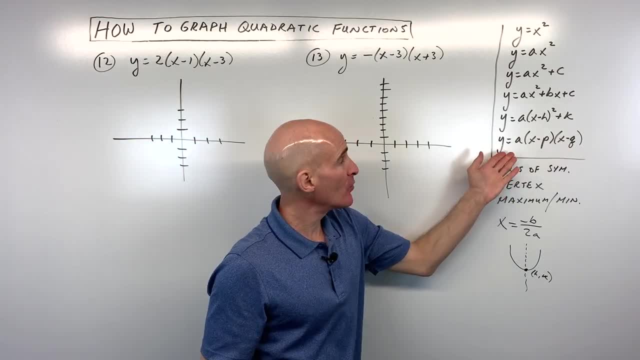 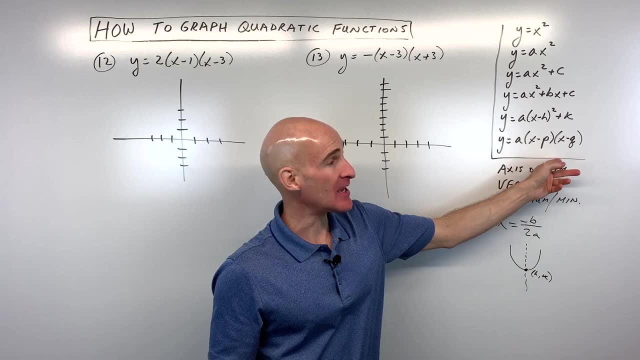 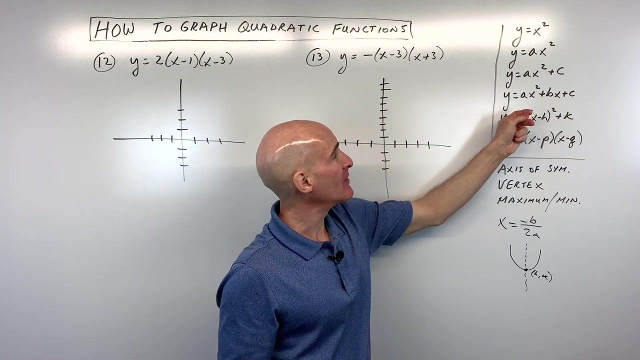 And the idea here is, with the intercept form, is the, when it's in this form, this factored form, what we can easily identify are the x-intercepts, or what are often referred to as the zeros, Whereas over here, in the vertex form, we can easily identify the vertex In this form here. 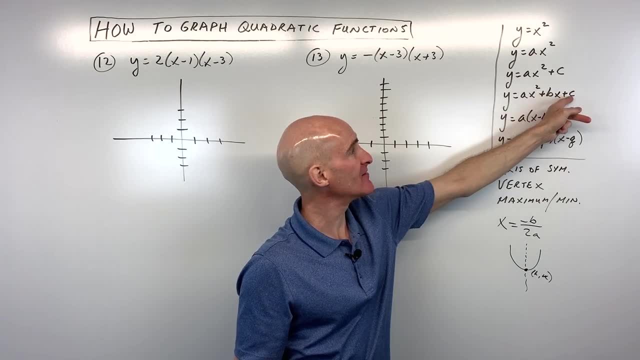 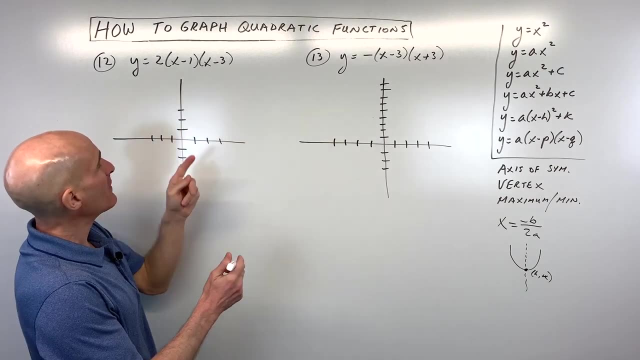 we can easily identify the y-intercept right, because we have the c-values, the y-intercept. So each form has kind of like its positives and its negatives, right. But for this one we can see it's in the factored form And the way we find those zeros. remember, the zeros means where the 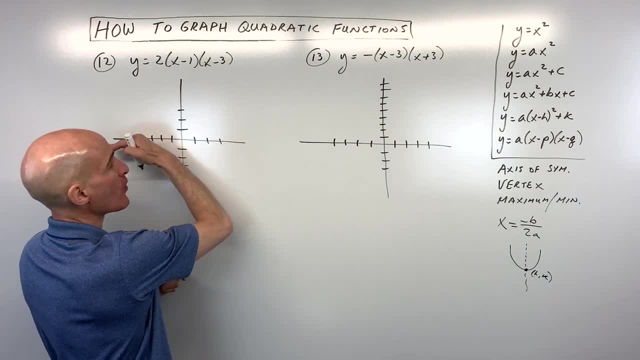 y-value is equal to zero. When y is zero, that means we're right along the x-axis, because we're not going up or down, and that gives us those x-intercepts. So what we do is we set y equal to zero and 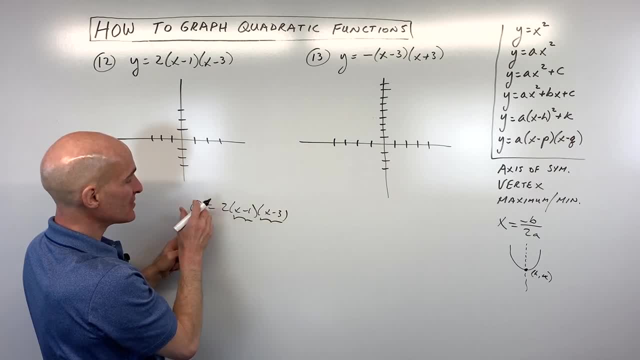 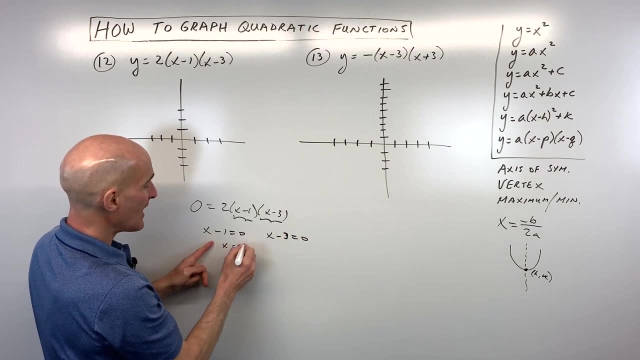 what you do is you set these factors or these groups equal to zero. So you can make a mini equation: x minus one equals zero and x minus three equals zero. Add one to both sides, add three to both sides and you can see that our zeros or our x-intercepts are going to be at one and. 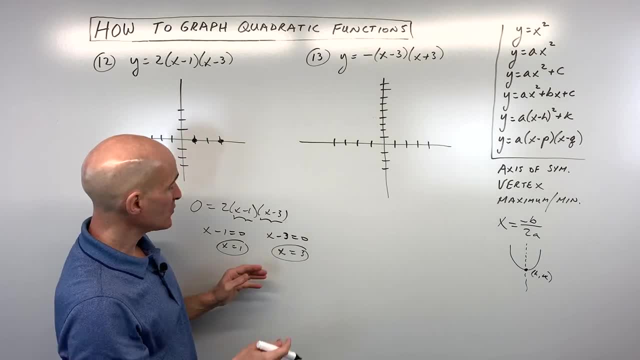 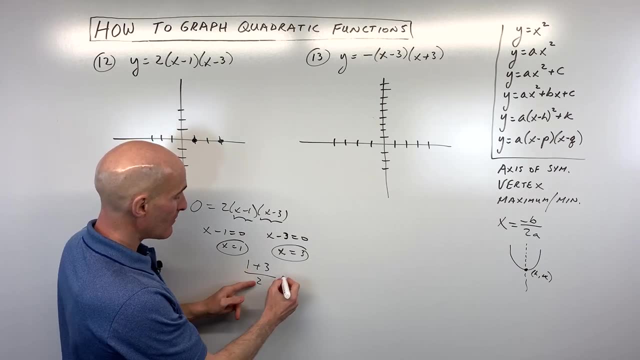 three. Now, what we can do from here, once we find these x-intercepts, is we can add them together and divide by two. So one plus three is four, divided by two is two. Now what does that two do for us? 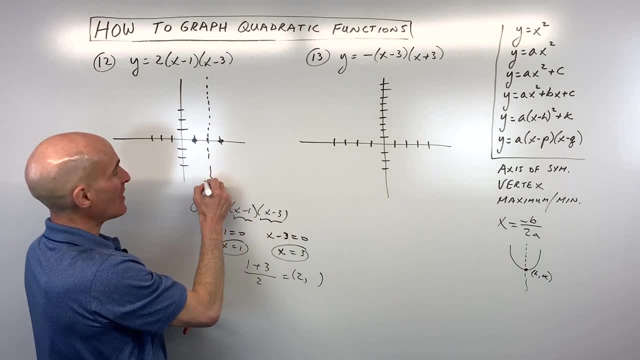 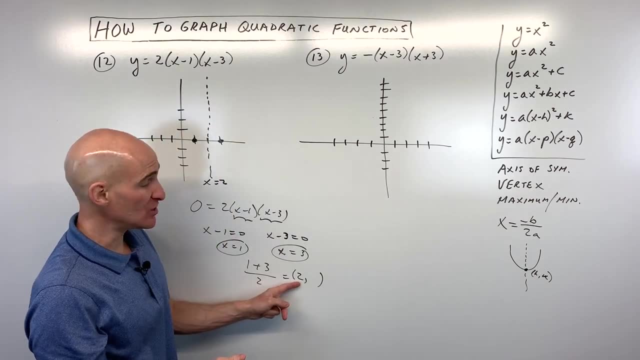 Well, it gives us the axis of symmetry. so x equals two, and because the vertex lies along that axis of symmetry, we know the x-coordinate of the vertex is going to be two. All we have to do now is put the two back in for x to find our y-coordinate of our vertex, and we got it. 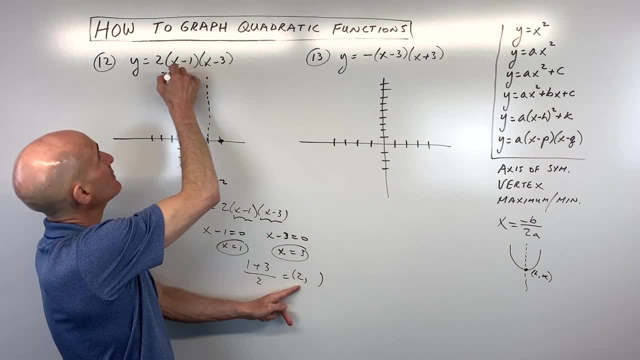 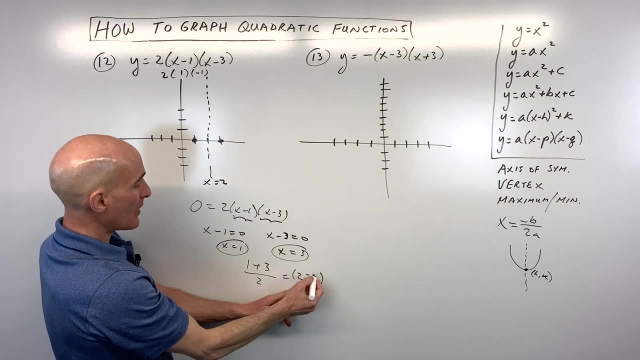 So let's do that: Two minus one is one, and two minus three is negative one, and so we have two times one is two times negative, one is negative two, and so now we've got our vertex here at two negative two. 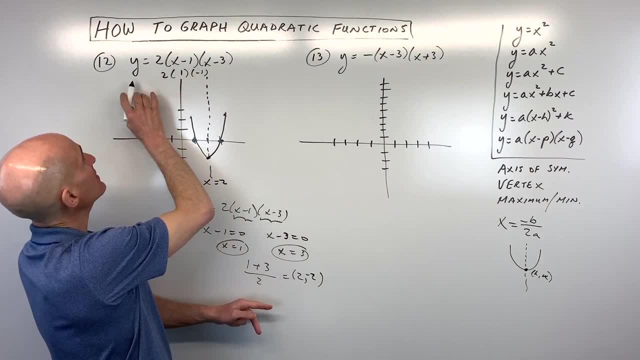 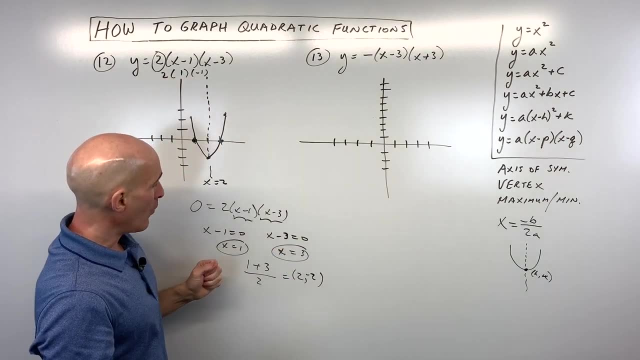 one thing to notice is that see how this a value is positive. that tells us the graph is opening up. if this was negative, then it would be opening down. now, what I want to show you here is we were doing the negative b over 2a. that was for the standard form, but here what we're doing is we're 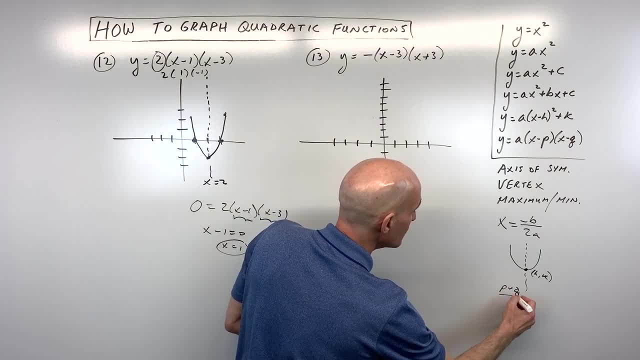 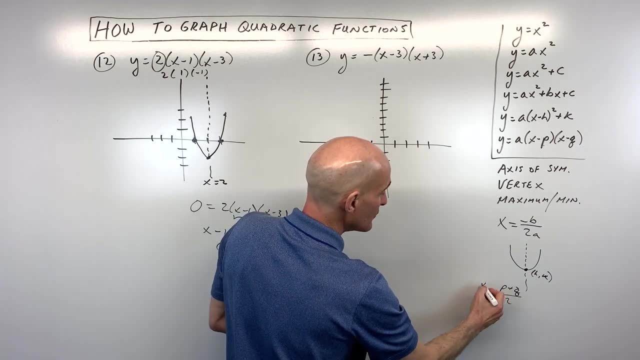 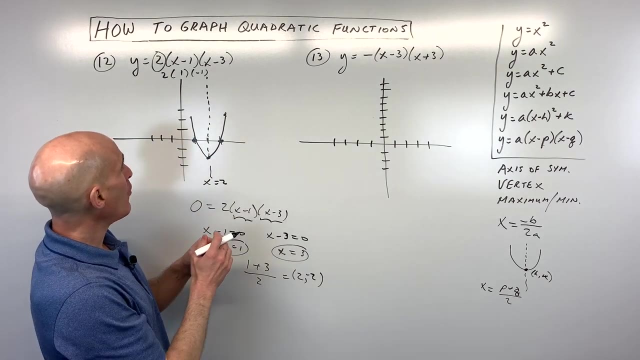 doing p plus q divided by 2. so p and q, these are our x intercepts. if you add those together and divide by 2, that's going to give you the x coordinate of the vertex and also the axis of symmetry. so now we've got a pretty good graph. if you want to plot some more points, you can instead. 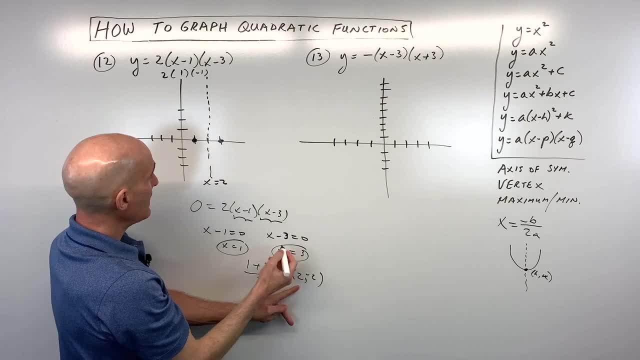 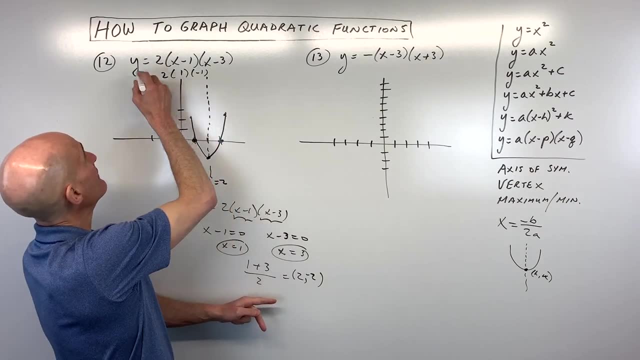 we have 2 times. 1 is 2 times negative, 1 is negative 2, and so now we've got our vertex here at 2 negative 2.. One thing to notice is that see how this a value is positive. that tells us the graph. 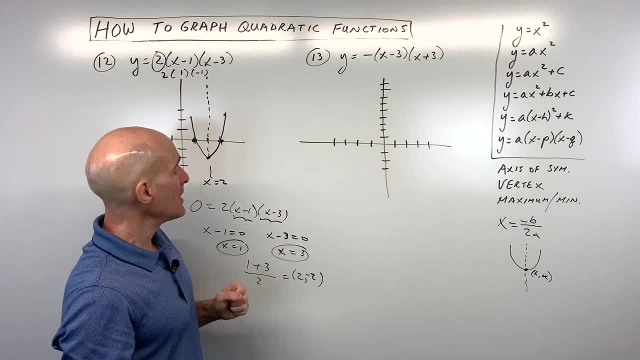 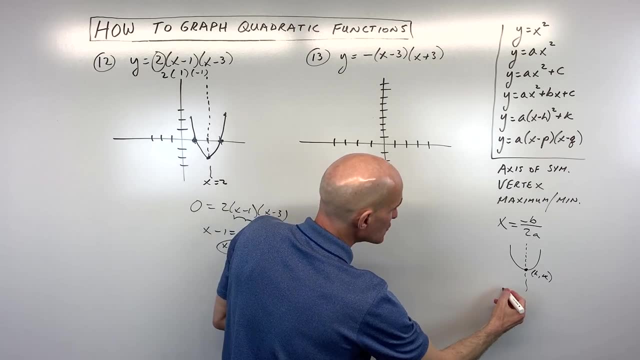 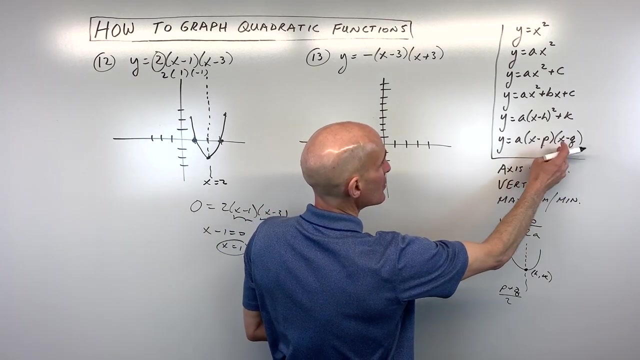 is opening up. If this was negative, then it would be opening down. Now what I want to show you here is we were doing the negative b over 2a. that was for the standard form. but here what we're doing is we're doing p plus q divided by 2. So p and q, these are our x-intercepts. if you add those, 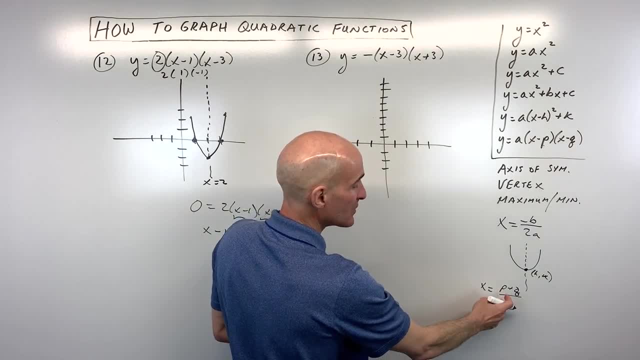 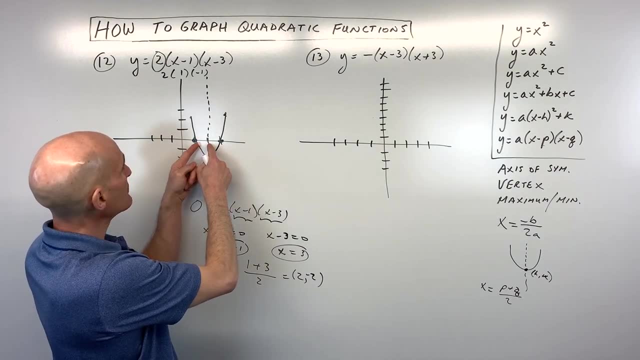 together and divide by 2. that's going to give you the x-coordinate of the vertex And also the axis of symmetry. So now we've got a pretty good graph. If you want to plot some more points, you can. instead of plotting like we did, 1, 2 and 3, we could do like 0. that would give you your. 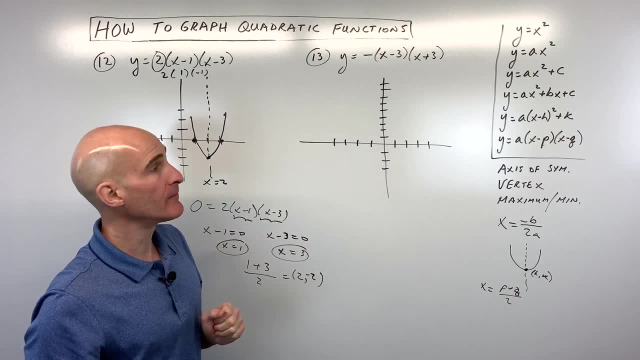 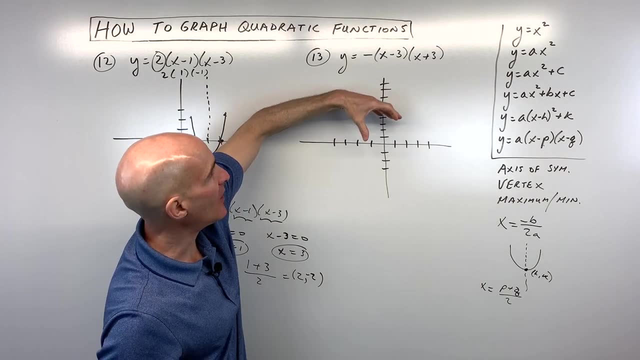 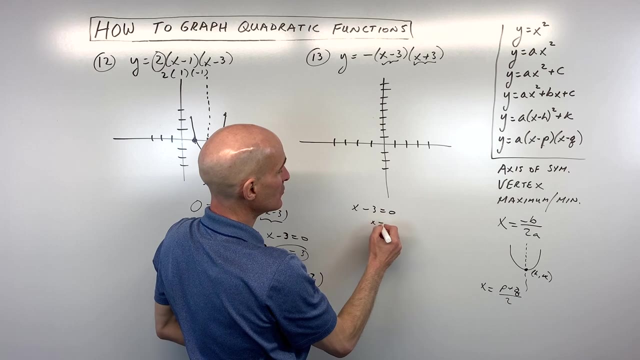 y-intercept, or you could 4. you can pick some other points to get more on your graph For number 13. now notice that this a value is negative or negative 1, so we know it's going to open down. If we set each of these factors equal to 0, we're going to get x minus 3 equals 0, so x equals 3. 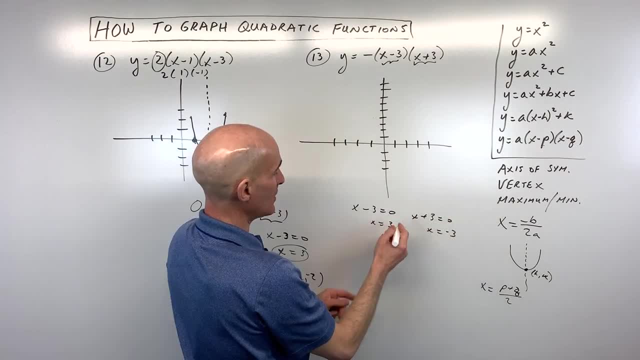 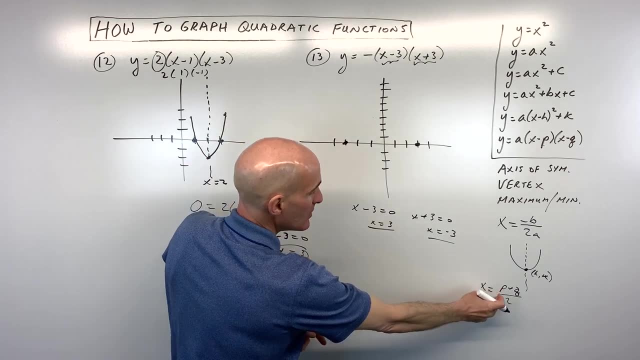 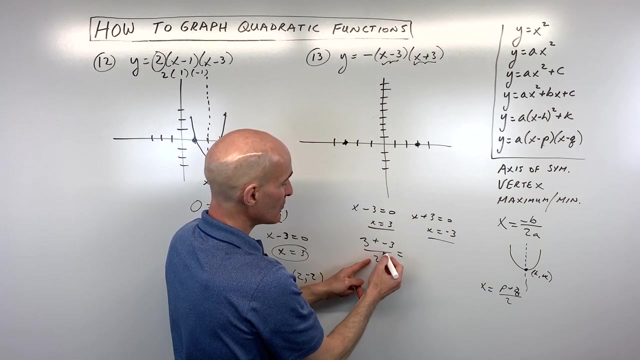 and x plus 3 equals 0.. So x equals negative 3.. So this is where it's going to be crossing the x-axis here, at 3 and negative 3. and if we use our p plus q over 2 formula, just like an average, you're adding them together and dividing by 2. that comes out to 3 plus negative 3 is 0. divided by 2 is 0.. 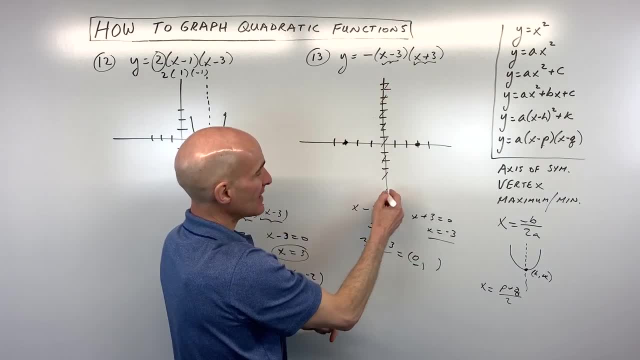 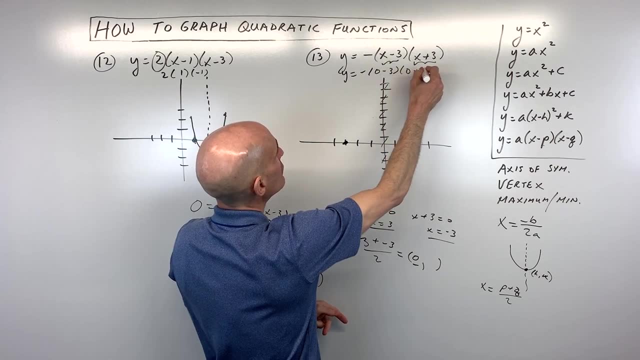 Okay, so this is our axis of symmetry. right here, on the y-axis, x equals 0. If we put 0 back in, we get negative 0 minus 3 times 0 plus 3.. Which is negative 9 times negative is positive 9.. So this is going to be 0 comma 9.. 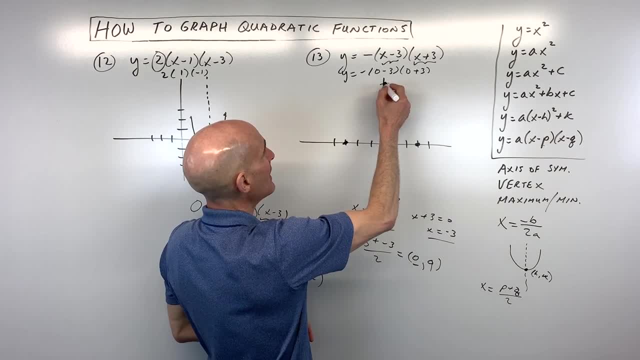 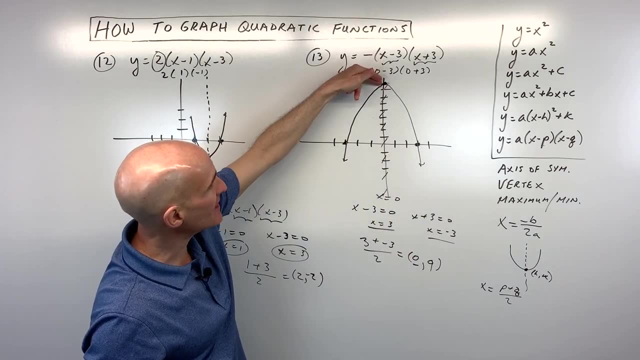 1, 2, 3, 4, 5, 6, 7, 8, 9, and now we have a pretty good sketch of our parabola. It's opening down because a is negative. We've got our vertex here, which was the average of the two x-intercepts. This is a. 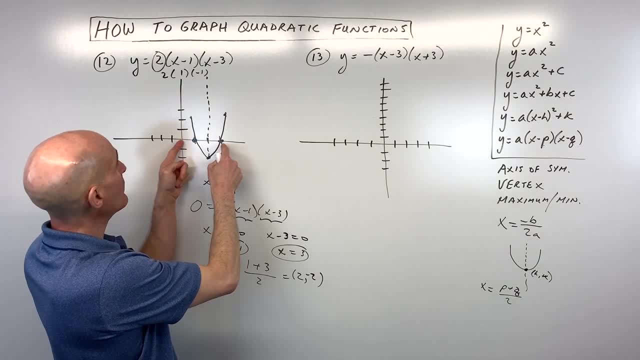 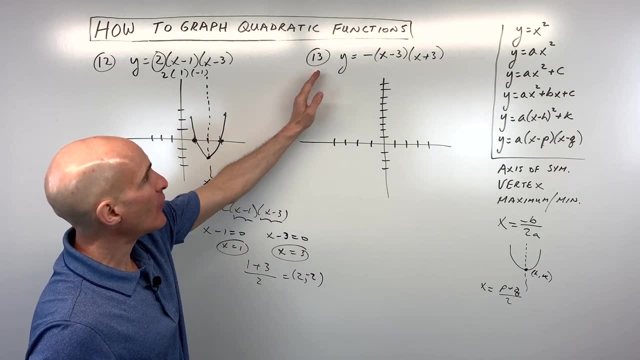 of plotting like we did, 1, 2 and 3. we could do like 0. that would give you your y intercept, or you could 4. you can pick some other points to get more on your graph. for number 13. now notice that this a value is negative or negative 1, so we know it's going to open down if we set each of these. 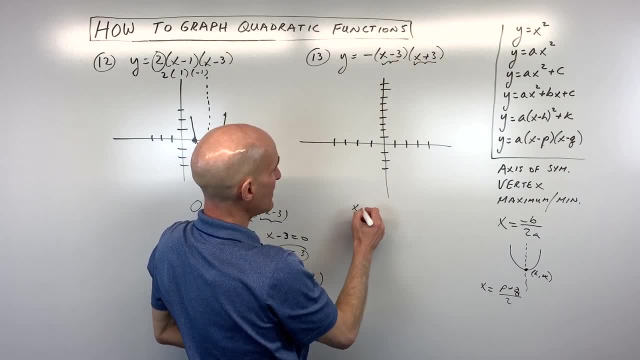 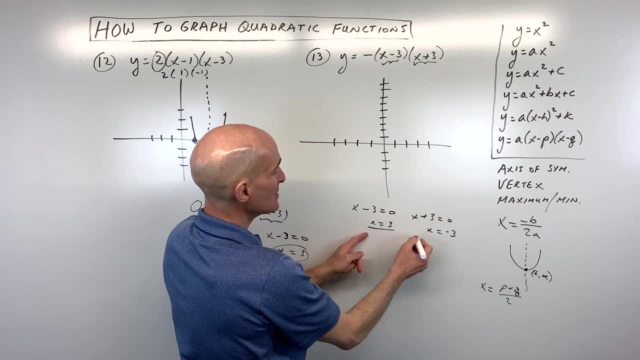 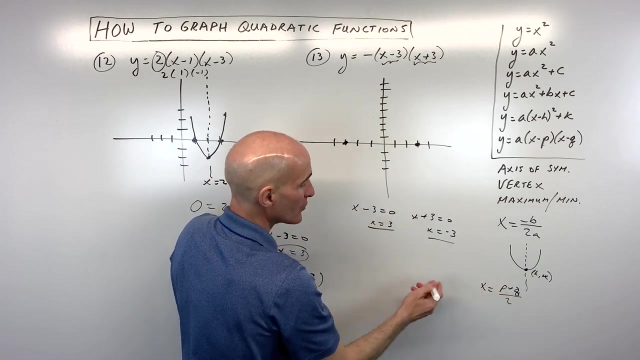 factors equal to 0, we're going to get x minus 3 equals 0, so x equals 3, and x plus 3 equals 0, so x equals negative 3. so this is where it's going to be crossing the x-axis, here, at 3 and negative 3, and if we use our p plus q over 2 formula, just. 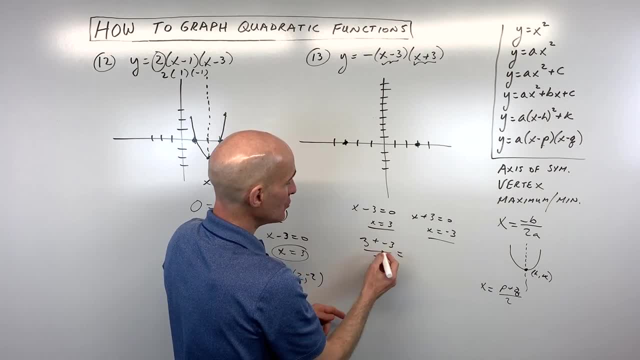 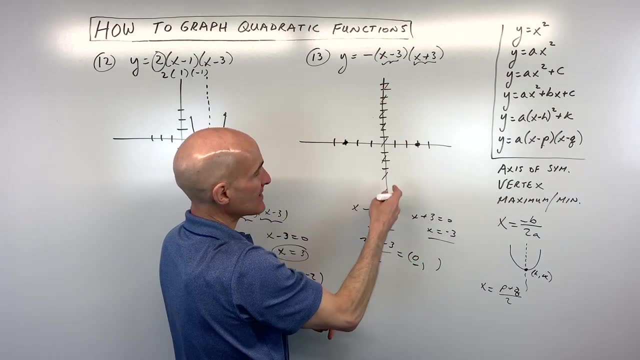 like an average. you're adding them together and dividing by 2. that comes out to 3 plus negative. 3 is 0. divided by 2 is 0. okay, so this is our axis of symmetry. right here. on the y-axis, x equals 0. 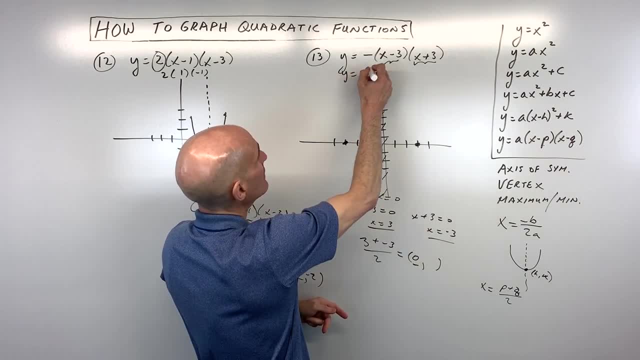 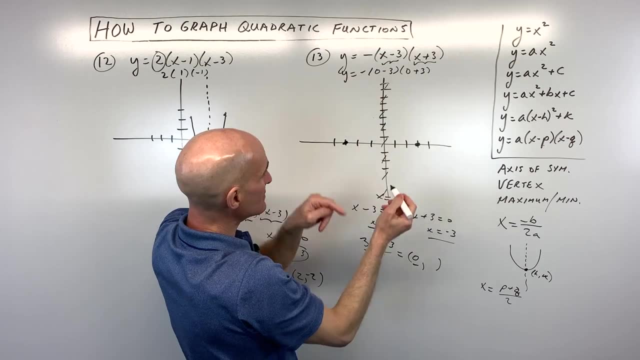 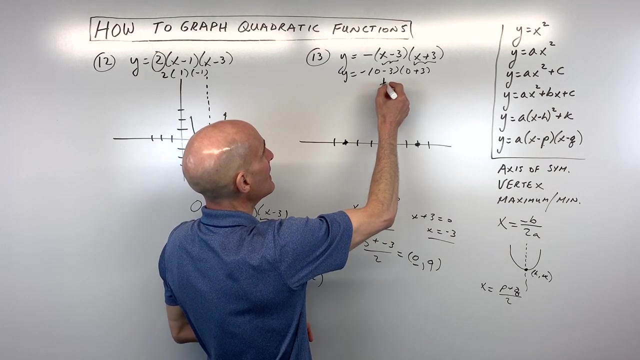 if we put 0 back in, we get 0 negative 0 minus 3 times 0 plus 3, which is negative. 9 times negative is positive 9. so this is going to be 0 comma 9, 1, 2, 3, 4, 5, 6, 7, 8, 9, and now we have a pretty good sketch of our 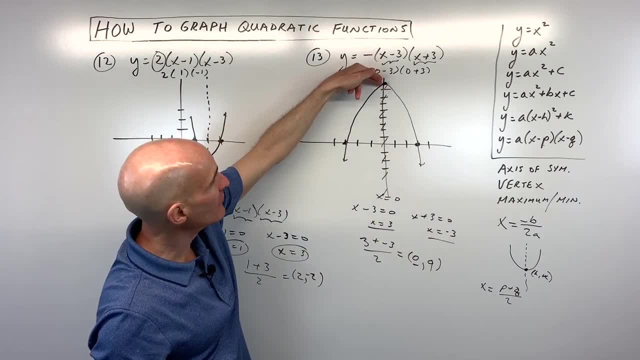 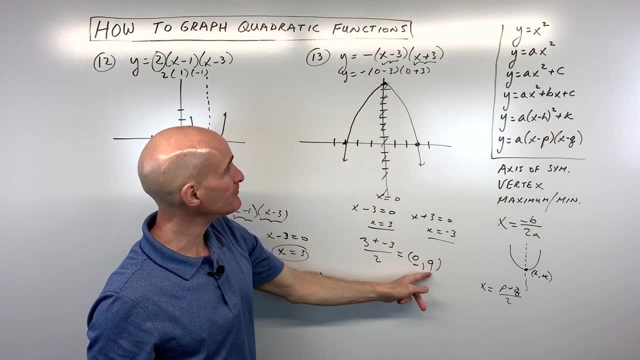 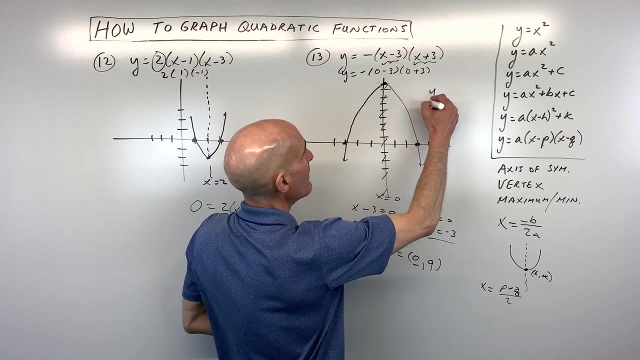 parabola. it's opening down because a is negative. we've got our vertex here, which was the average of the two x intercepts. this is a maximum and the maximum value is 9 and we know the axis of symmetry. x equals 0. we know that the range is going to be below this maximum, so y is less than or equal to. 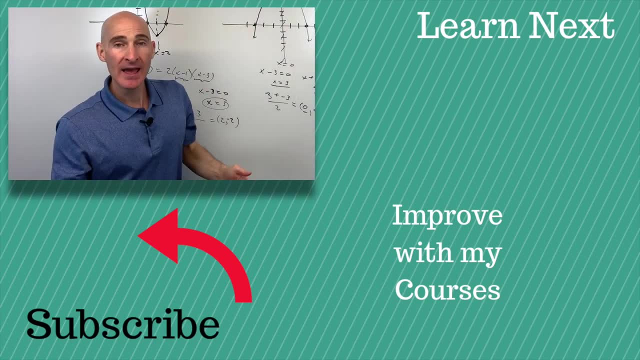 9, the domain is all real numbers and you got it. so in the comments, put down your favorite method for graphing these quadratus or these parabolas, and if you want to see more examples, follow me over to that video right there where i'll dive into some more examples. i'll see you in the next. 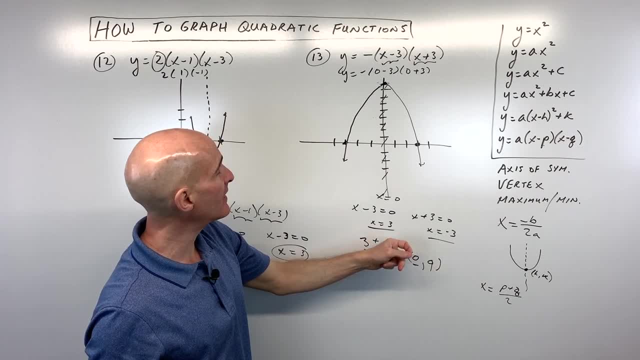 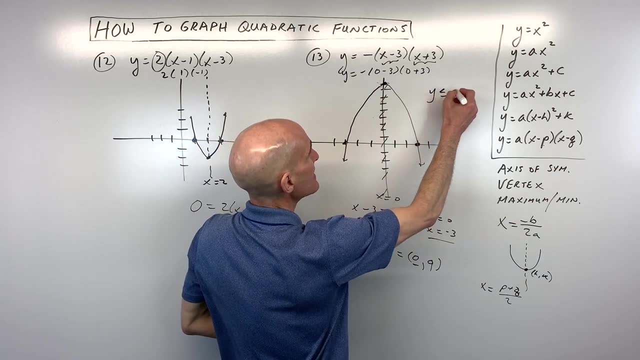 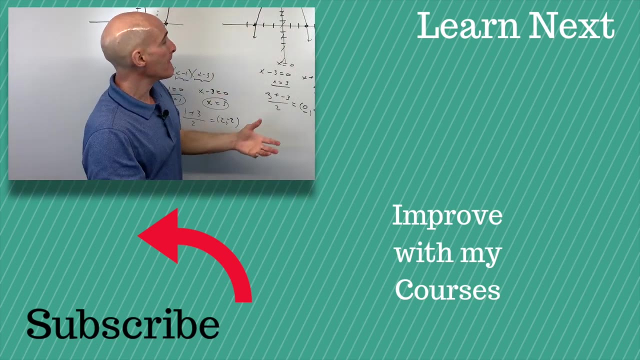 maximum and the maximum value is 9, and we know the axis of symmetry: x equals 0.. We know that the range is going to be below this maximum, so y is less than or equal to 9.. The domain is all real numbers and you got it. So in the comments, put down your favorite method for graphing these quadratus or these parabolas and if you want to see more examples, follow me over to that video right there where I'll dive into some more examples. I'll see you in the next video. 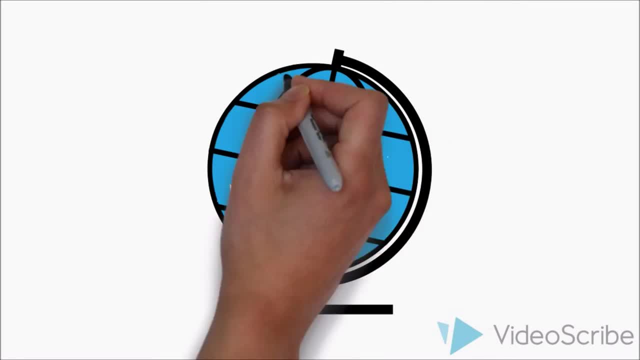 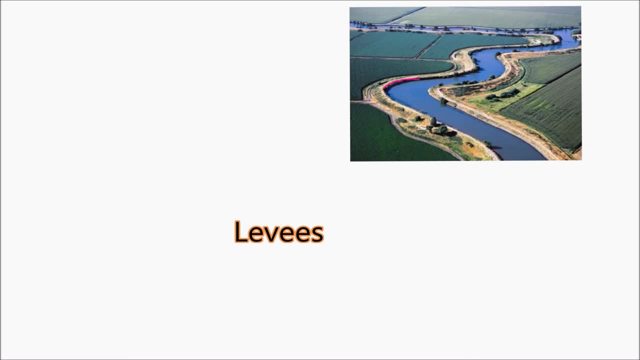 Hello everyone. In this video we're going to be looking at another river feature. In this case we're going to be looking at levees, and specifically natural levees. You can see that I'm labelling them over here on the photograph. They're those little raised sections that you get on either side of the river that prevent river flooding and are famous for having failed in the Hurricane Katrina disaster. 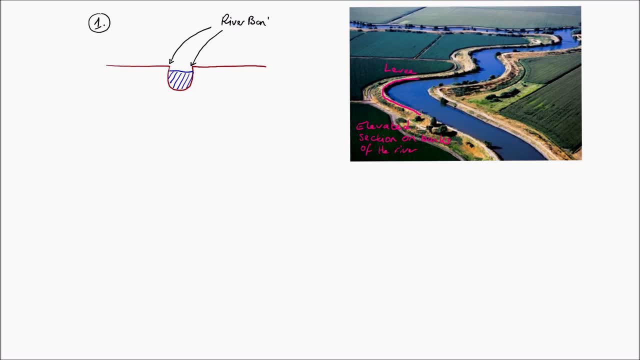 So how does a levee form? Well, a levee forms over here, directly on the river banks that I'm labelling in Diagram 1, and they're a naturally occurring and naturally forming feature. So what occurs is, as we can see in Diagram 2, is that during a flood conditions, or during flood conditions, when the water level rises above the banks, 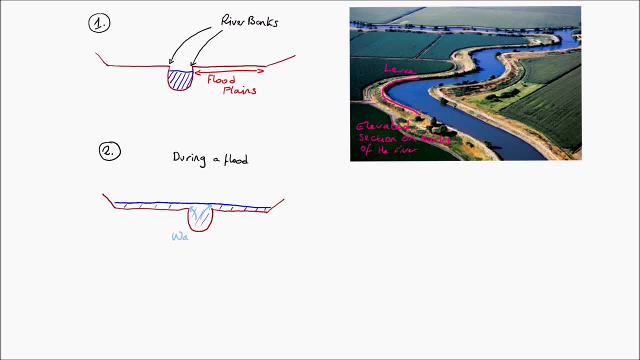 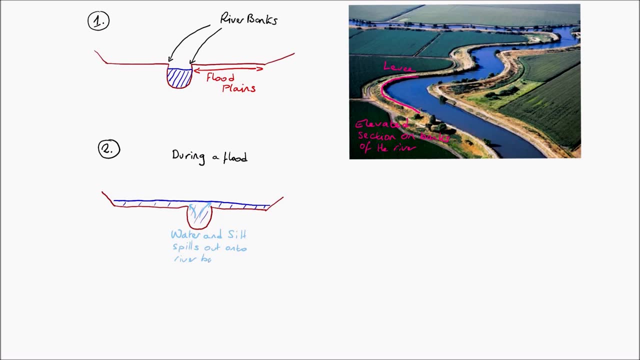 that the area directly on either side of the bank is the first area where they're going to be exposed to additional friction, And large stones and silt are first deposited directly in the areas that I'm marking with a little red circle. This is because this is where they lose their energy first and it's the place where all the larger sediment is deposited. 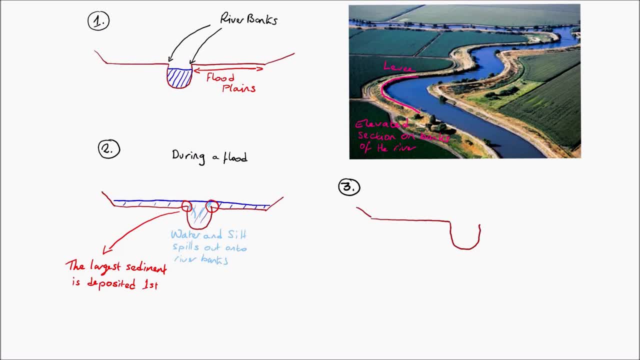 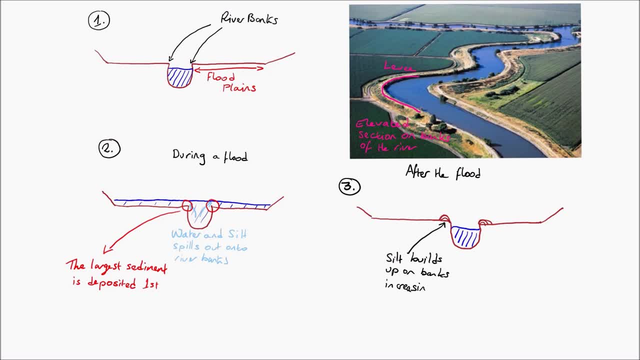 what it does is that it forms this elevated section that you can see both on the diagram and in the photograph. What these levers can do is they can increase the river carrying capacity and they prevent the river flooding in the future, because now the channel can hold more water.